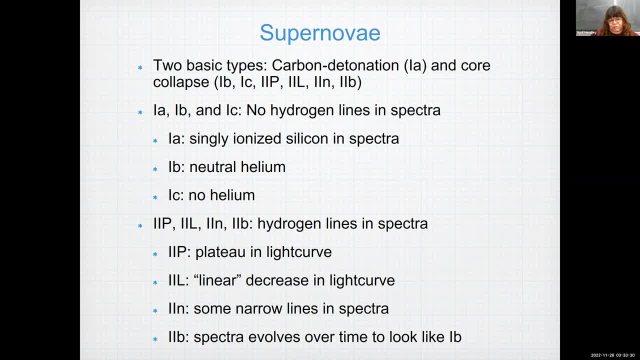 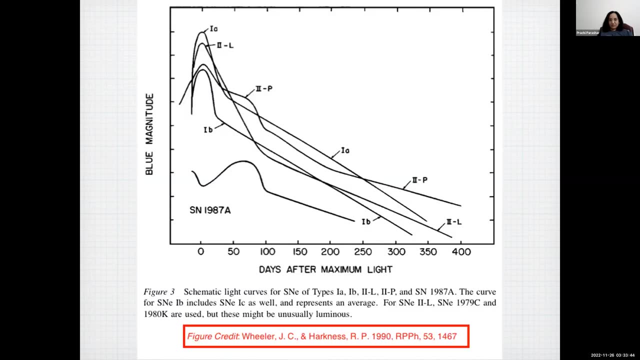 Okay, For the most part I'm not going to worry too much about all the different types. I'm just going to worry mostly about carbon debt, difference between carbon detonation and core collapse. Oh, I guess the next slide isn't quite explaining them yet. 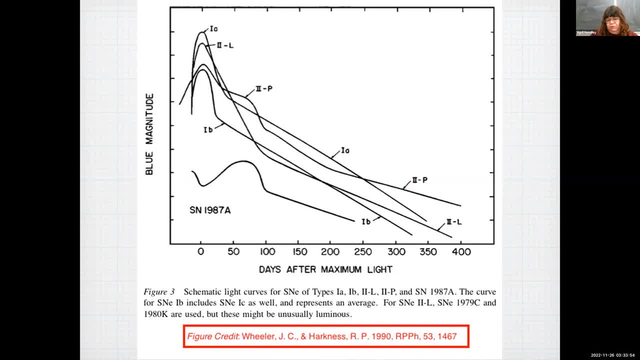 This shows basically how they brighten. They don't reach peak brightness immediately. It takes about a week, And the one that we are most connected with Gary Burse is 1c, which is also the same line as 1b. 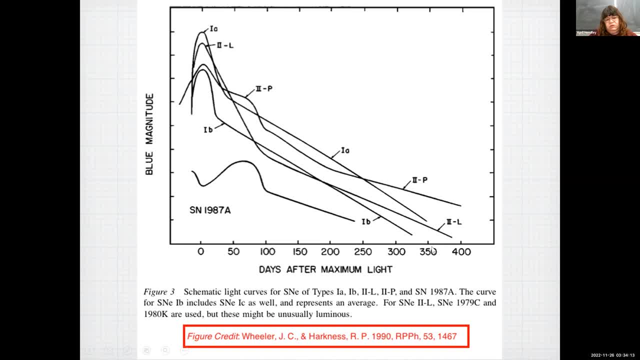 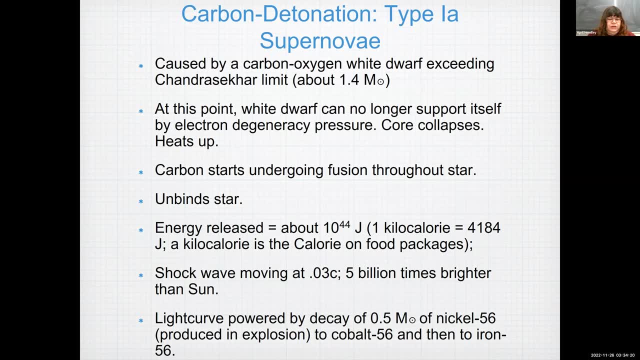 On this, Okay, Okay, So different types. I'm going to go with core collapse first and get it out, or not. core collapse, carbon detonation first and get it out of the way, And then worry about core collapse, carbon detonation or detonation. the ones that's not connected to Gary Burse are the ones that's also referred to as type 1a, and what they are is a carbon. 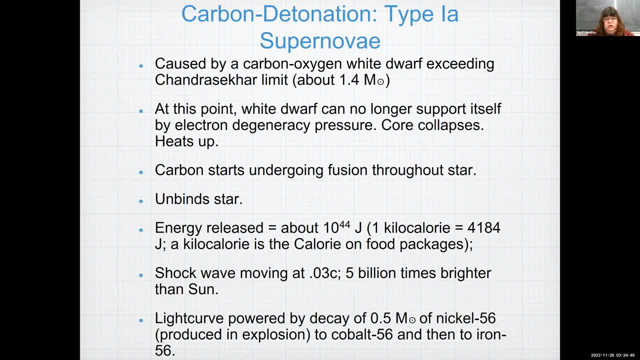 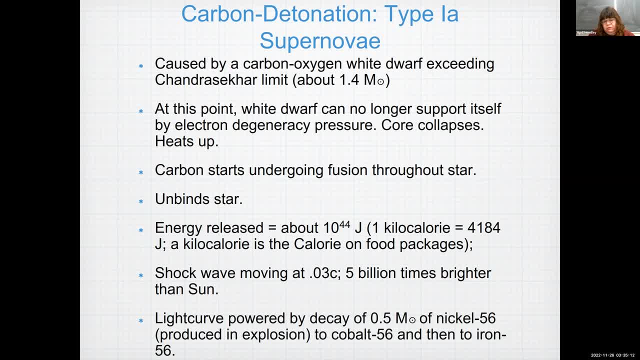 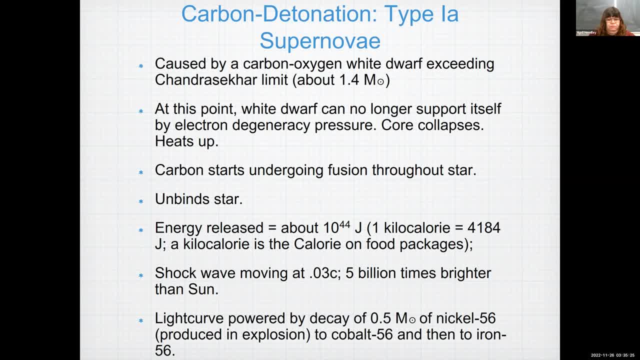 If they got squeezed anymore they basically get smashed into protons and get mostly neutrons. But and up until 1.4 solar masses the electrons resisted that half. But once this white dwarf reaches 1.4 solar masses it's not going to be able to do anything. 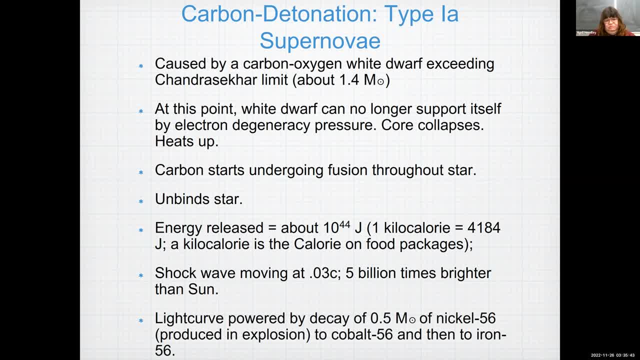 The time at which it hits the first electron and goes to 1.4 solar masses is basically that no longer can prevent gravity from collapsing it further. The time at which it hits the first electron and goes to 1.4 solar masses is basically that no longer can prevent gravity from collapsing it further. 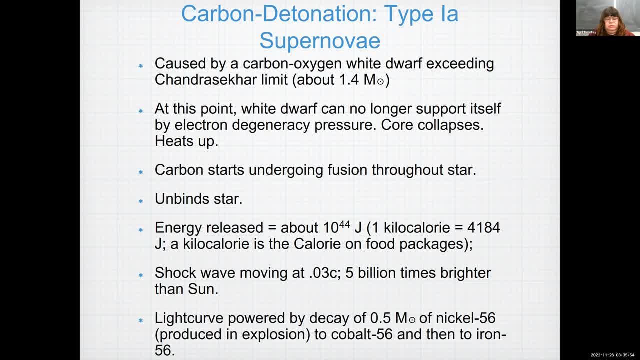 The core will collapse as it classes. it heats up and carbons undergoing fusion throughout the star at once And basically the star blows up. And basically the star blows up, Let's see releases a lot of energy. It's about 10 to the 44th joules. 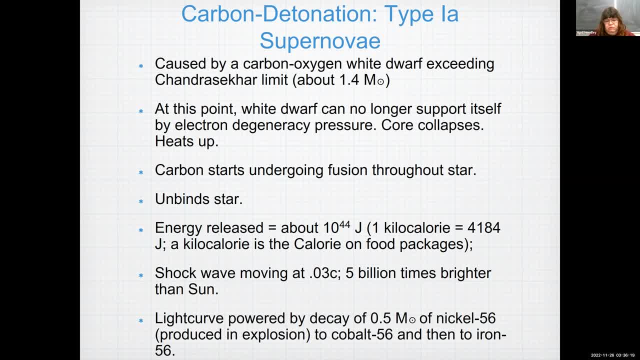 Let's just say a lot And you get shockwave moving outward about roughly 0.03 times the speed of light and they're about five billion times brighter than the sun. The one thing with these type of supernovas: they all have about the same brightness. so we 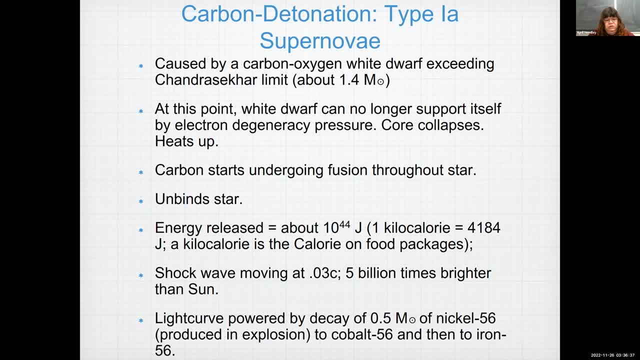 use them to get estimate distances to the galaxies they occurred in. Last slide applies to both this type of supernova and the core flaps. The light doesn't come from the explosion itself. In the explosion you get basically nickel 56 produced about half the solar mass. The M with the circle and dot means solar mass. 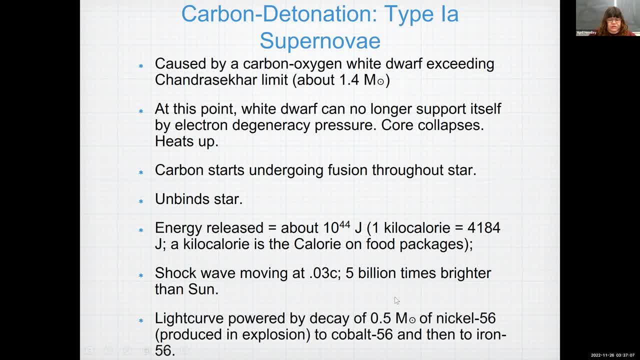 Anyway, nickel 56 is radioactive. It decays to cobalt 56, which is also radioactive, and that decays to iron 56. And the light from the supernova basically comes from that radioactive decay. Like I said, that applies to both carbon detonation and the core class supernovas. 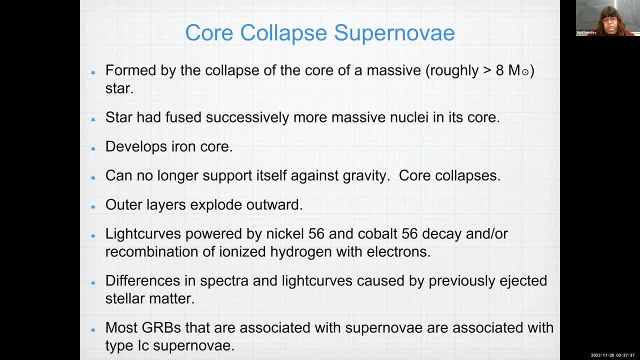 Anyway, the core class supernova is formed basically by death of a massive star, roughly more than eight times the mass of the sun. Anyway, a star that massive can fuse a lot heavier elements in its core than our sun can. Our sun will fuse hydrogen to helium and then helium to carbon, and that's basically it for our sun. The more massive star can fuse the carbon and so on and so on, until it finally fuses silicon to iron. Once it gets the iron core, it has a problem. It can't get energy out of iron by fission or fusion. Basically, to get iron to undergo either fission or fusion. 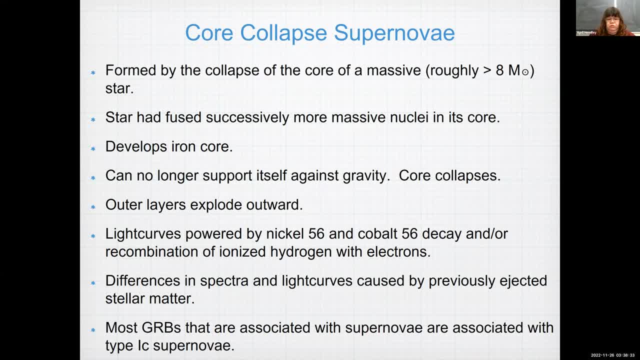 you have to add energy to iron to get it to do one of those two. But you can't get energy out of the iron by fusion or fission, which means it suddenly loses its energy source and it can't support itself against gravity. Up until that point the star supported itself against gravity. because you have this hot. 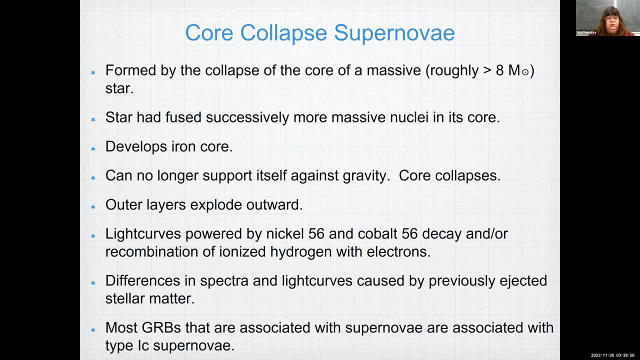 basically it's hot and it's trying to expand because it's so hot while gravity was trying to pull it inward and there was a balance. But whenever get iron- like I said, you can't get energy out by iron- It can't support itself against gravity and the core collapses. 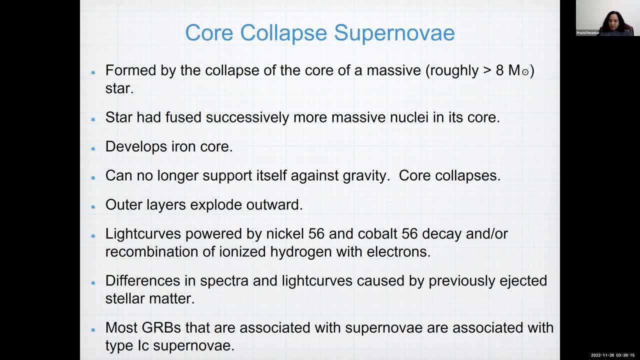 So can I ask a very tangent question here, Like: so all the other elements can be made by fusion, which happens inside the star up till iron, Yeah, But beyond that you cannot fuse anything to keep creating higher elements. That is what I'm hearing. 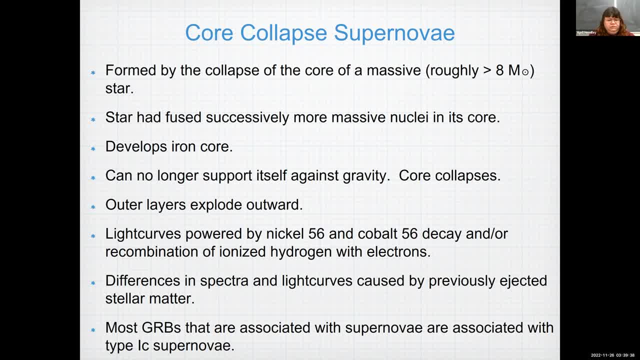 Well, you can't get energy out of them by, you can't get energy out of fusion past iron. So, by any chance, do you know, like, how the heavier elements are formed? then I think some of those formed in supernovae, some in some reaction at the very end of the star's life. 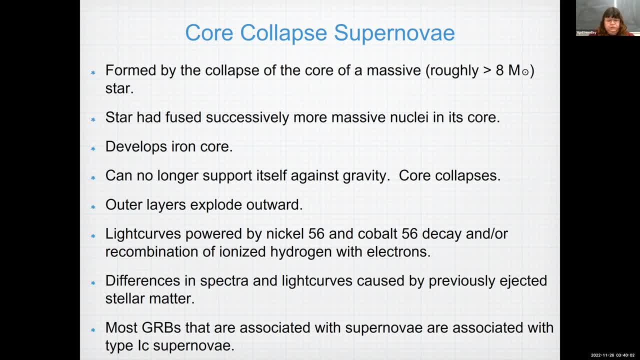 There's various methods on how some of them get formed, but So, but basically during those, some of them get formed during the supernova itself, And is it true that, like I mean at the core of our earth also, like there is some sort of radioactive reaction happening? 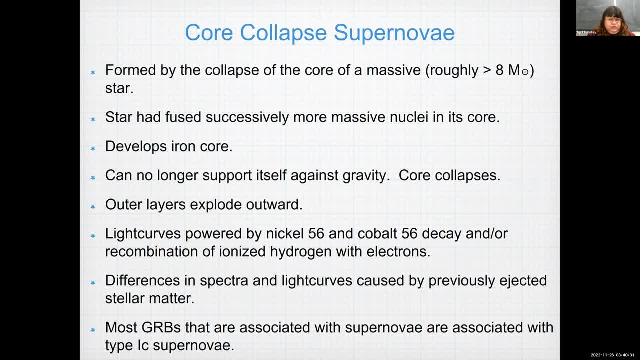 I think so. I think so. that was at one point that just didn't, Didn't work, Didn't work, Didn't work, Didn't happen, generated some of the energy, the or heat that the core had. whether it still has much going on, i 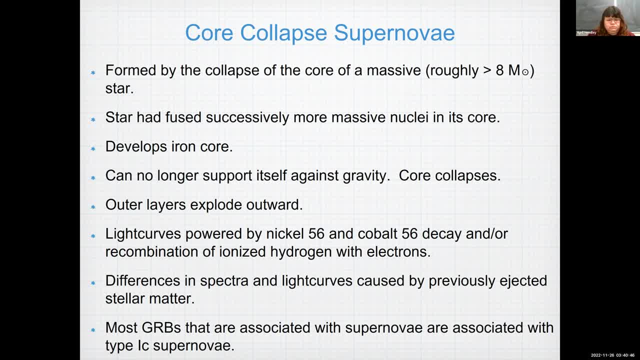 really don't know for sure. okay, yeah, okay. so i said, the core can't support itself against gravity anymore and it collapses, and it basically more or less collapses to a certain point. i almost wouldn't compare it to hits bottom picture, like a ball being dropped in it bouncing, but basically, 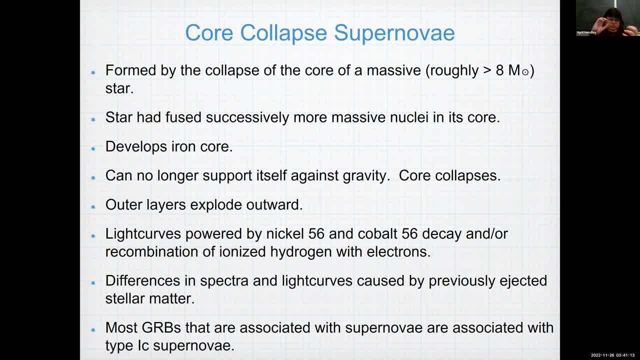 collapses, hits bottom and then basically rebounds back. and when it rebounds back, it basically slams into the outer layers of the star and basically blast them off, and and and. so during all that, you get the nickel 56 produced which, like i said, decays to cobalt 56, which then 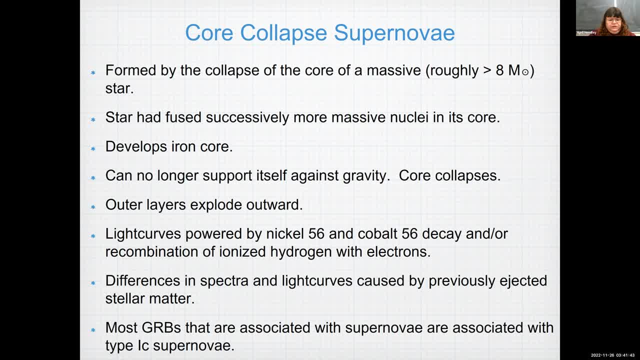 decays to iron 56, you get ionized hydrogen and electrons recombining and and the differences in the spectra and the light curves that we see with the core collapses caused by stuff that's previously been ejected from the star, or caused by stuff that's previously been ejected from the star or possibly some of the surrounding interstellar medium. 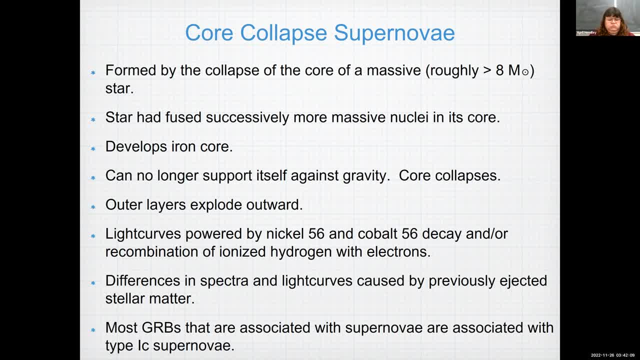 possibly some of the surrounding interstellar medium. like: if we don't see any hydrogen, that means the like: if we don't see any hydrogen, that means the stars basically already lost most of the hydrogen. stars basically already lost most of the hydrogen outer envelopes that they've. 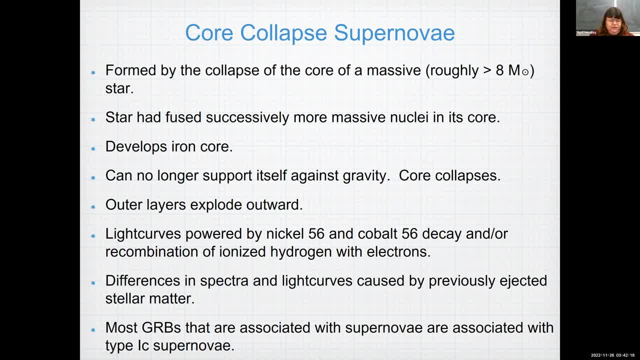 outer envelopes that they've. that's basically. that's basically: stars lose mass and expel the mass. stars lose mass and expel the mass. um, and if we don't see any hydrogen, that, and if we don't see any hydrogen, that means that's basically already been lost. 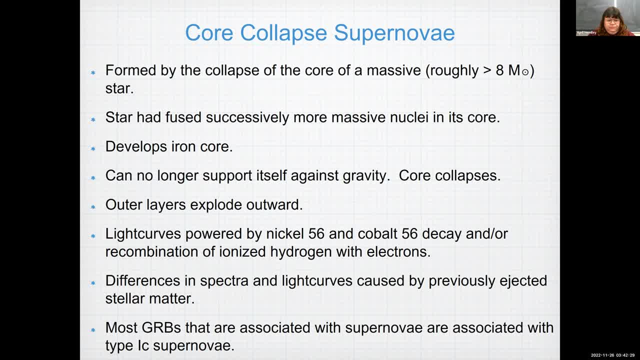 means that's basically already been lost, and stars it's lost. the helium that means, and stars it's lost. the helium that means the helium's, the helium's. we don't see helium in their spectrum, so we don't see helium in their spectrum, so we don't see helium in their spectrum. so and um. 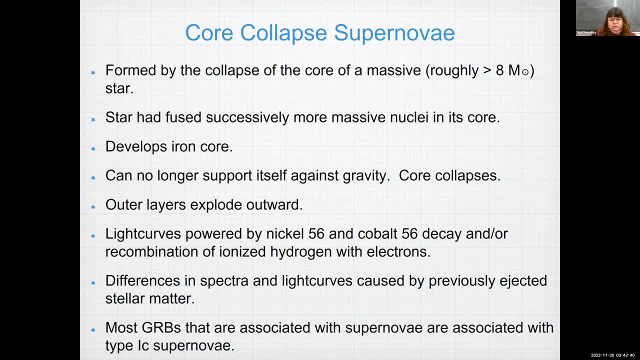 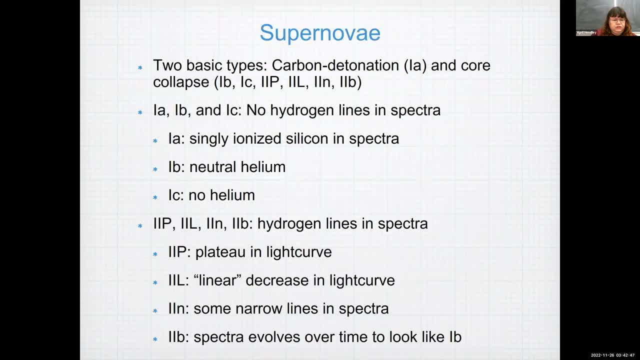 and um, anyway, anyway, anyway, most of the gamma reverse are associated. most of the gamma reverse are associated. most of the gamma reverse are associated with um, with um, with um supernova that's type 1c supernova, that's type 1c supernova, that's type 1c. if i go back for a second, 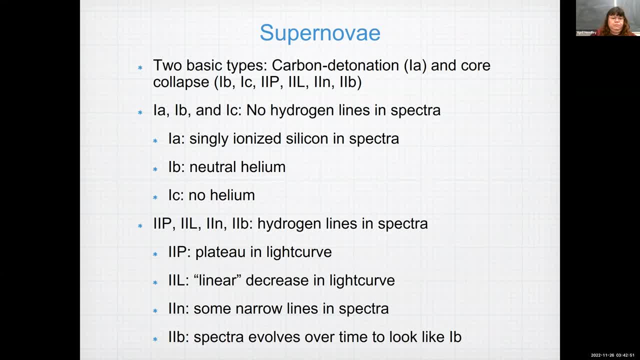 if i go back for a second, if i go back for a second, type 1c is one that we don't see. hydrogen. type 1c is one that we don't see. hydrogen. type 1c is one that we don't see hydrogen or helium. 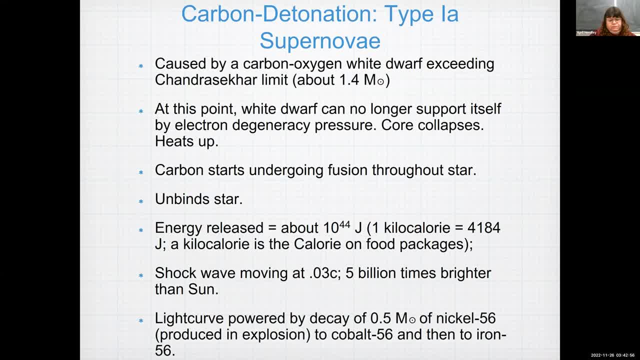 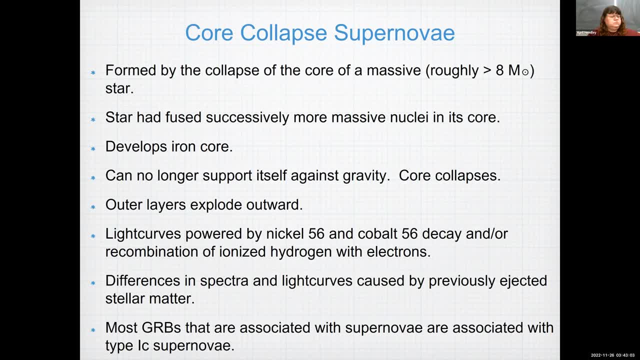 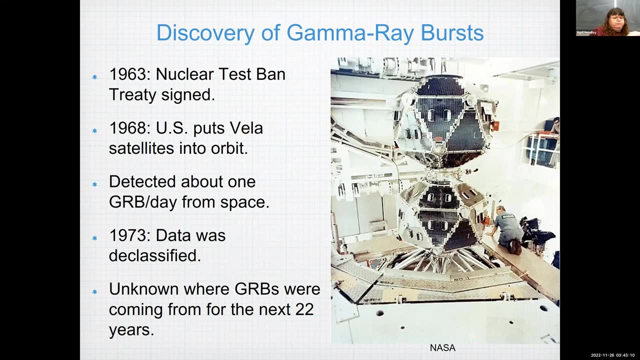 or helium, or helium, so it's lost both the out. so it's lost both the out. so it's lost both the out: hydrogen and helium. but that was around hydrogen and helium, but that was around hydrogen and helium, but that was around the core, the core, the core. 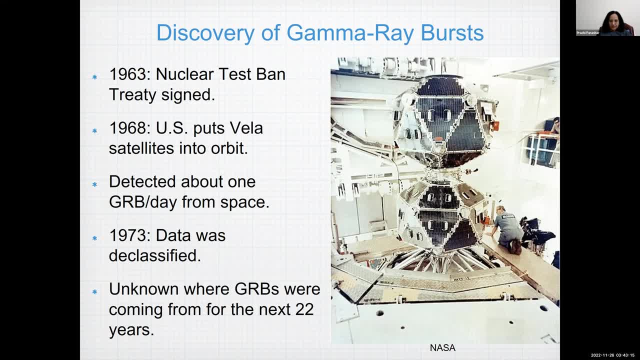 so once the once it collapses, uh. so, once the once it collapses, uh. so once the once it collapses, uh, and ejects the outer layer out, and ejects the outer layer out, and ejects the outer layer out, what it becomes, what it becomes, what it becomes, um. 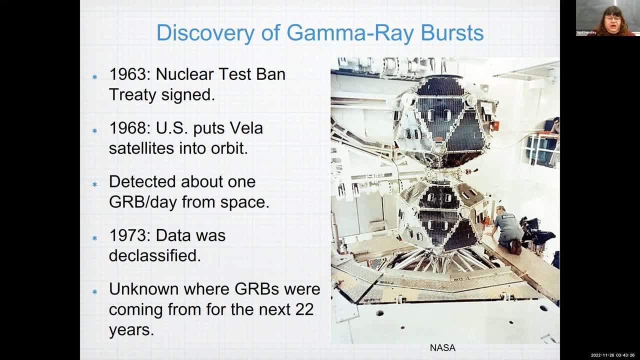 um, um, well after, well after, well after, after the supernova, the outer layers after the supernova, the outer layers after the supernova, the outer layers keep expanding and we see a supernova keep expanding and we see a supernova keep expanding and we see a supernova remnant. 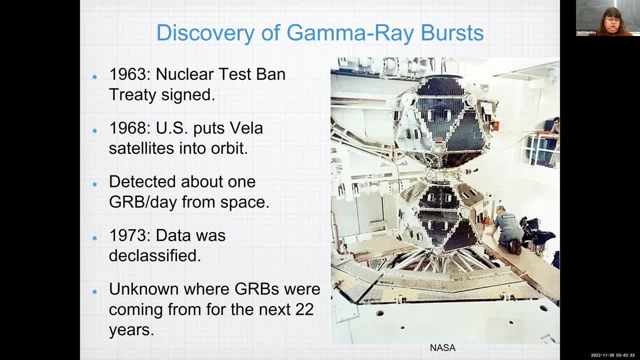 remnant, remnant in the center part, in the center part, in the center part. what's left? what's left? what's left? if it's on the lower mass side, it, if it's on the lower mass side, it. if it's on the lower mass side, it becomes a neutron star. 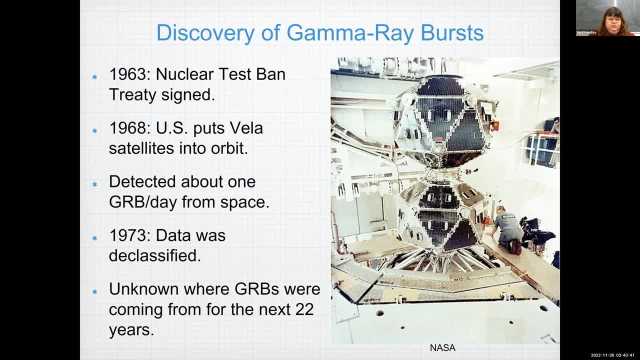 becomes a neutron star, becomes a neutron star, which is, which is, which is about the size of a, about the size of a, about the size of a metropolitan area, metropolitan area, metropolitan area, and has a density like that of the atomic, and has a density like that of the atomic. 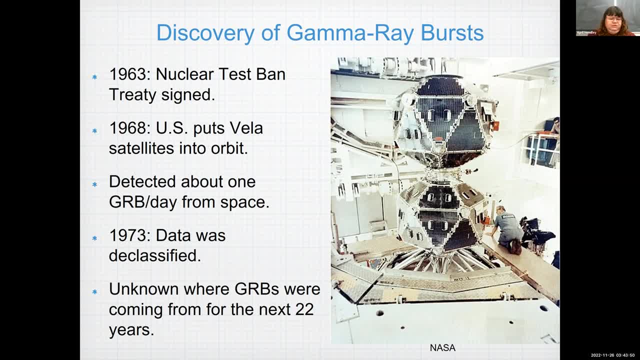 and has a density like that of the atomic nucleus, nucleus, nucleus and they and they, and they spin very fast, spin very fast, spin very fast. like, like, like, seconds, fractions of a second seconds, fractions of a second seconds, fractions of a second. some of them, even, some of them, even. 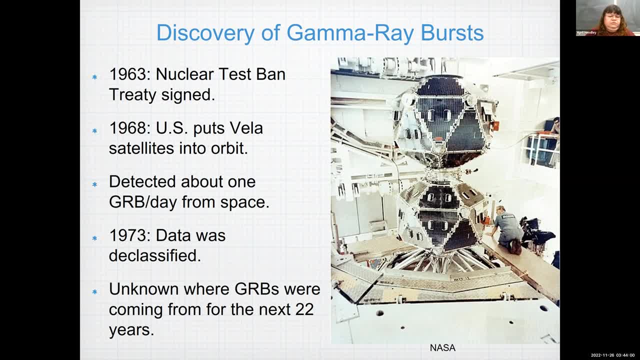 some of them even hundreds of a second, or hundreds of a second, or hundreds of a second, or um, um, um, and they also have very strong magnetic and they also have very strong magnetic and they also have very strong magnetic fields, fields, fields. if it's on the, if what's left is on the. 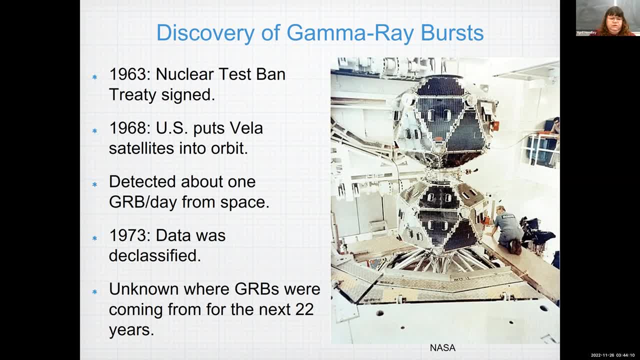 if it's on the, if what's left is on the, if it's on the, if what's left is on the higher mass, higher mass, higher mass, side, side side, then we don't know of any force that. then we don't know of any force that. 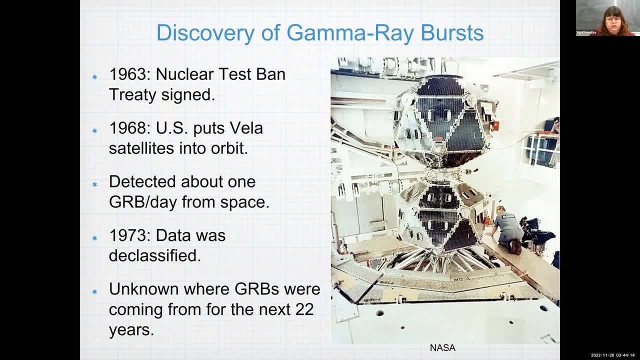 then we don't know of any force that will keep it from collapsing all the way, will keep it from collapsing all the way, will keep it from collapsing all the way, currently, currently, currently. then it becomes a black hole, then it becomes a black hole, then it becomes a black hole, whether it actually collapses all the way. 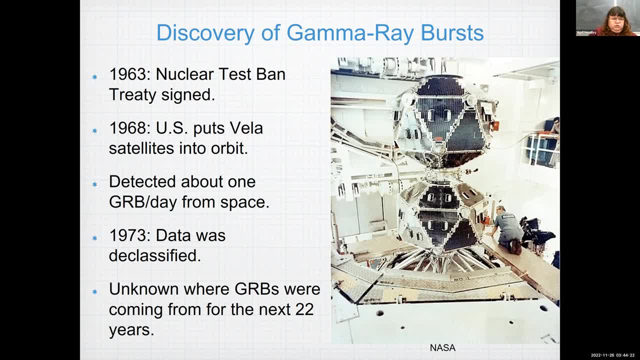 whether it actually collapses all the way, whether it actually collapses all the way to a singularity, though. to a singularity though. well, that part um, well, that part um. well, that part um, basically, our physics will last until it, basically, our physics will last until it. basically, our physics will last until it gets very tiny, but not all the way to. 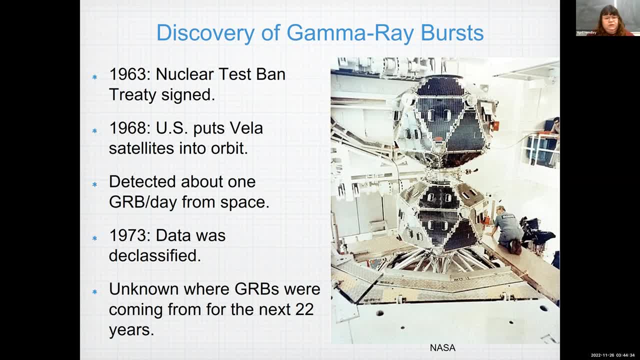 gets very tiny, but not all the way to. gets very tiny, but not all the way to zero radius and and and though, since we can't get light, or though since we can't get light, or though, since we can't get light or anything out of a black hole, it's kind. 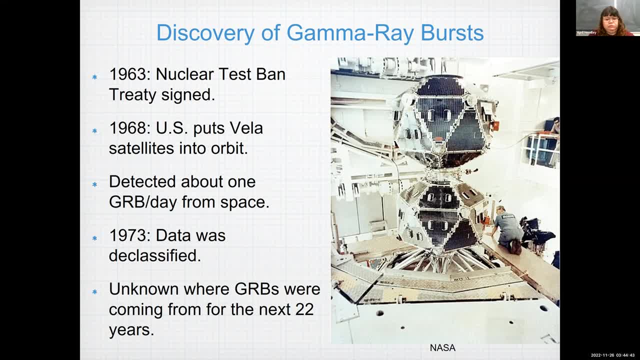 anything out of a black hole. it's kind anything out of a black hole. it's kind of hard to of hard to of hard to actually see what happens inside, actually see what happens inside, actually see what happens inside. so okay, so okay, so okay, so next next. 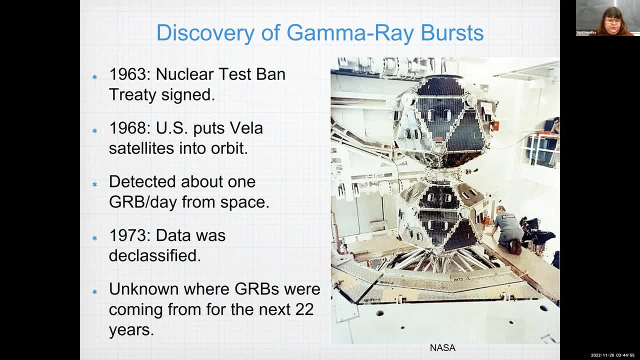 next, next, next day. it was declassified day. it was declassified day. it was declassified. however, however, however, for the next 22 years, for the next 22 years, for the next 22 years, it wasn't certain where the gamma. it wasn't certain where the gamma. 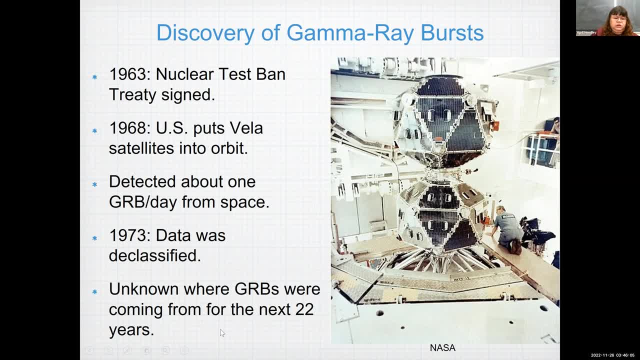 it wasn't certain where the gamma reverse were coming from, what produced reverse were coming from, what produced reverse were coming from, what produced them. basically, basically, basically, we couldn't, we couldn't, we couldn't. we could get a general area of the sky. we could get a general area of the sky. 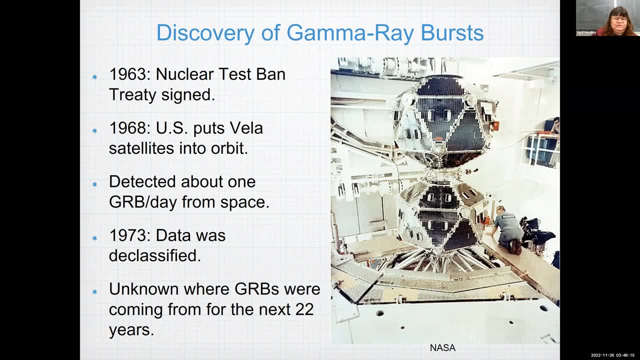 we could get a general area of the sky where one came from, but we couldn't where one came from. but we couldn't where one came from, but we couldn't localize exactly where that one came. localize exactly where that one came, localize exactly where that one came from, it was still over a large area. 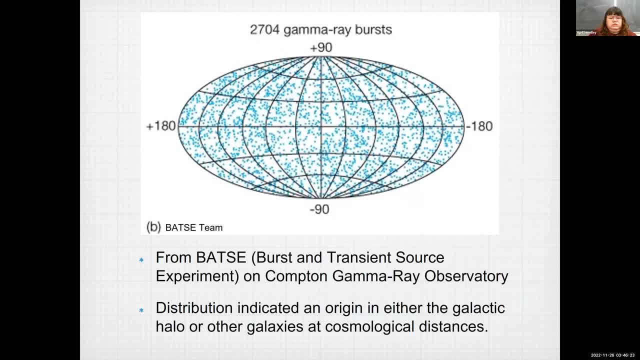 from it was still over a large area. from it was still over a large area. what we could do was get. what we could do was get. what we could do was get them with each individual and reduce to them with each individual, and reduce to them with each individual and reduce to small enough area that we could get kind. 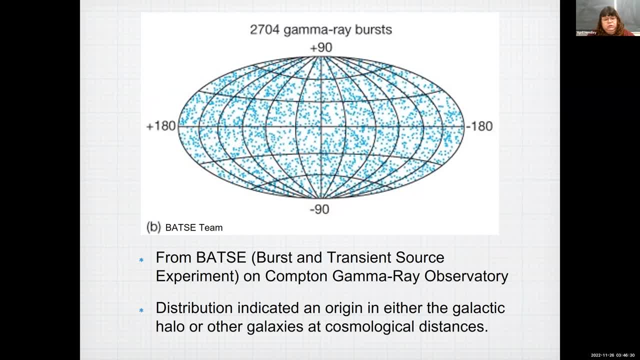 small enough area that we could get kind, small enough area that we could get kind of an overall distribution on the sky, of an overall distribution on the sky, of an overall distribution on the sky. and this is and this is and this is from from from one satellite. 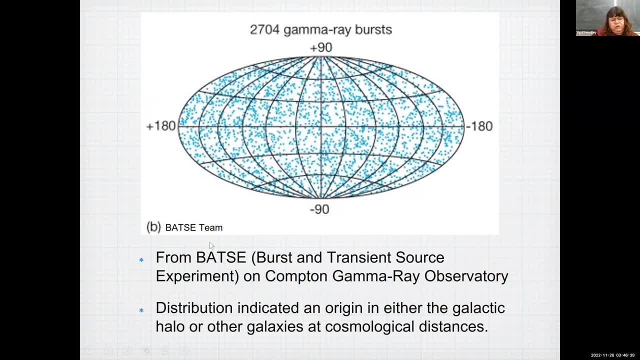 one satellite. one satellite called burst and transient source called burst and transient source called burst and transient source. experiments on experiments on experiments on: was on compton gamma ray observatory. was on compton gamma ray observatory. was on compton gamma ray observatory and basically shows 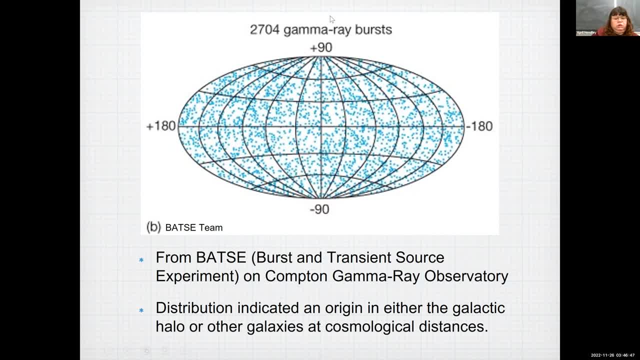 and basically shows, and basically shows: whoops, how'd i, whoops, how'd i, whoops, how'd i? i don't know why i hit, but i don't know why i hit, but i don't know why i hit, but, um, um, um, basically, it shows the distribution. 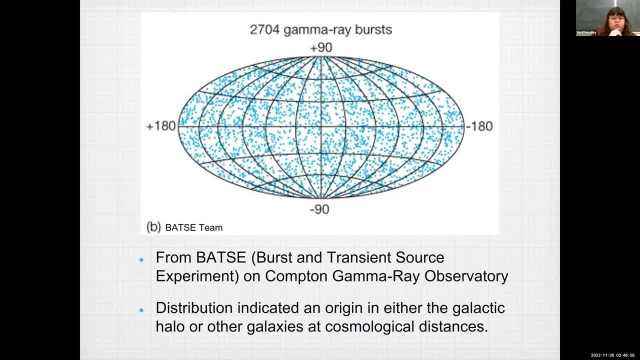 basically it shows the distribution, basically it shows the distribution overall on sky, overall on sky, overall on sky, and there was no and there was no and there was no certain area on the sky where they were certain area on the sky where they were certain area on the sky where they were localized. that seemed to be more. 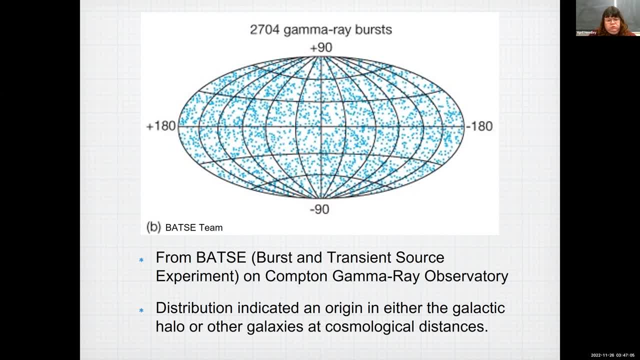 localized, that seemed to be more localized, that seemed to be more uniformly distributed. uniformly distributed, uniformly distributed, which led them to conclude. it was which led them to conclude. it was which led them to conclude. it was either something like, either something like, either, something like um the galactic halo that surrounds 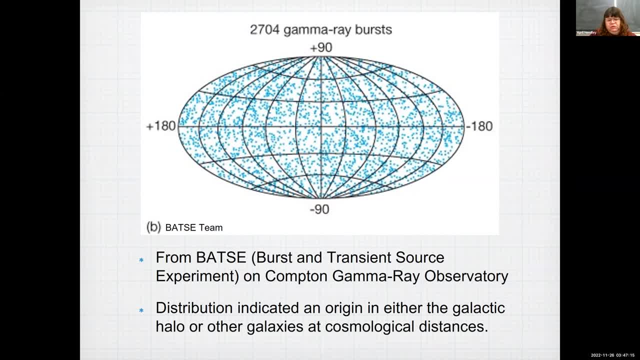 um the galactic halo that surrounds um the galactic halo that surrounds our galaxy, our galaxy, our galaxy, or or or other galaxies at cosmological distances, other galaxies at cosmological distances, other galaxies at cosmological distances. it actually turned out to be. it actually turned out to be. 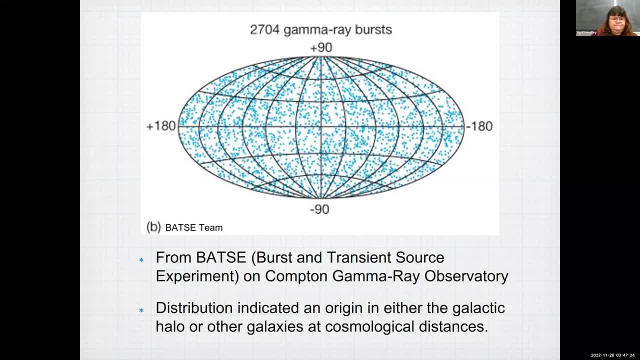 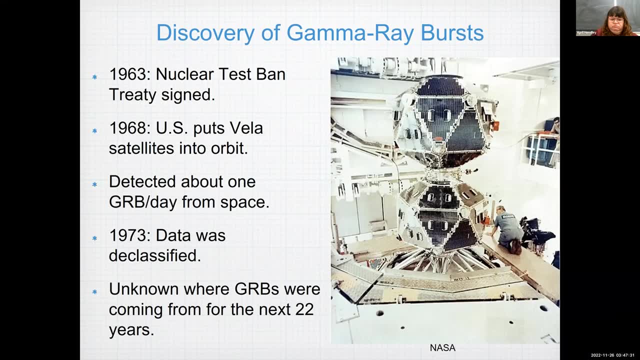 it actually turned out to be the other galaxies at cosmological, the other galaxies at cosmological, the other galaxies at cosmological distances, distances, distances, so so, so, um, but, like i said, didn't know that for um. but, like i said, didn't know that for um, but, like i said, didn't know that for about 22 years. 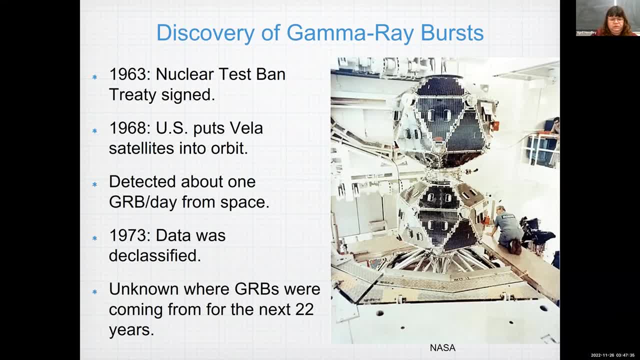 about 22 years. about 22 years until after the um, until after the um, until after the um data was declassified, or so so. on this data was declassified, or so so. on this data was declassified, or so so. on this slide like: what is the relevance of a? 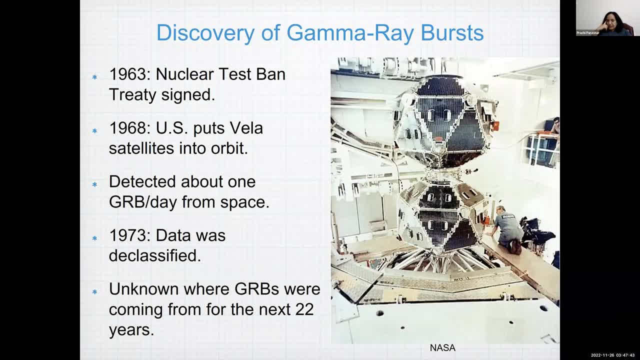 slide like: what is the relevance of a slide like: what is the relevance of a nuclear test? uh ban treaty. and sending nuclear test: uh ban treaty. and sending nuclear test: uh ban treaty. and sending the satellite in the sky. the satellite in the sky, the satellite in the sky? well, there's villa satellites is how the 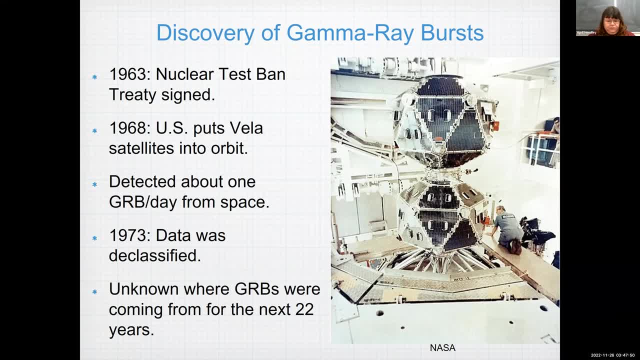 well, there's villa satellites is how the well, there's villa satellites is how the was what first detected the gamma was what first detected the gamma was what first detected the gamma, reverse from reverse from reverse, from coming from space, coming from space, coming from space, and they were basically. 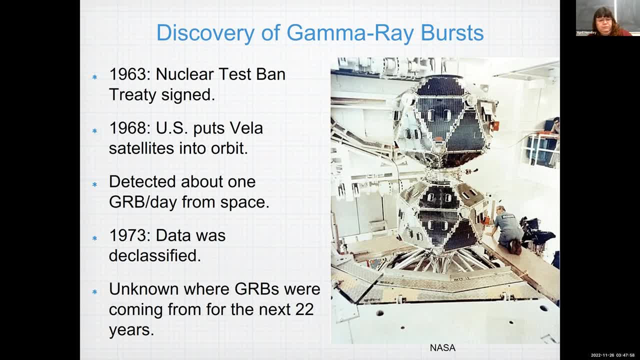 and they were basically, and they were basically put up to watch for someone violating a. put up to watch for someone violating a. put up to watch for someone violating a nuclear test ban treaty. okay, okay, okay. in other words, if the tree hadn't been, in other words, if the tree hadn't been. 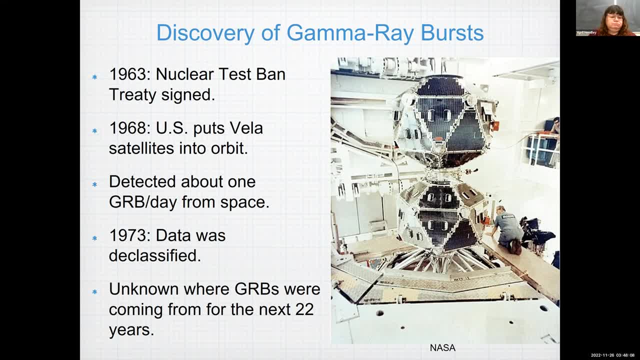 in other words, if the tree hadn't been signed, and signed, and signed, and you guys haven't put up the satellites, you guys haven't put up the satellites. you guys haven't put up the satellites. have been, have been, have been, might have been longer before we. 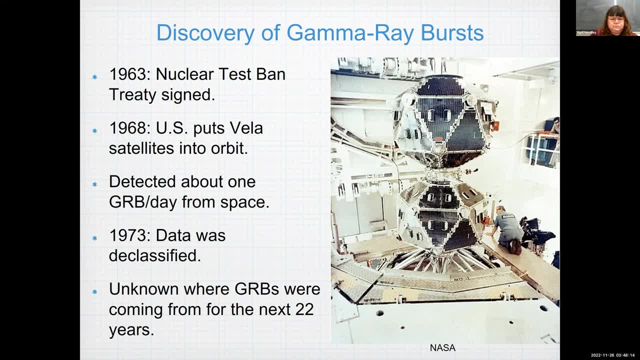 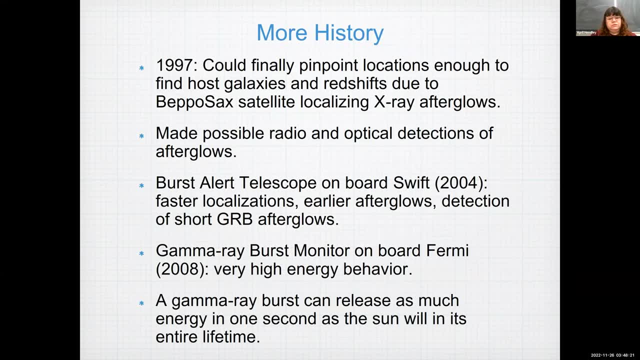 might have been longer before. we might have been longer before we discovered gamma reversed, discovered gamma reversed, discovered gamma reversed. okay, um, so anyway. um, i'm in 1990, about 1997, we could start. i'm in 1990, about 1997, we could start. 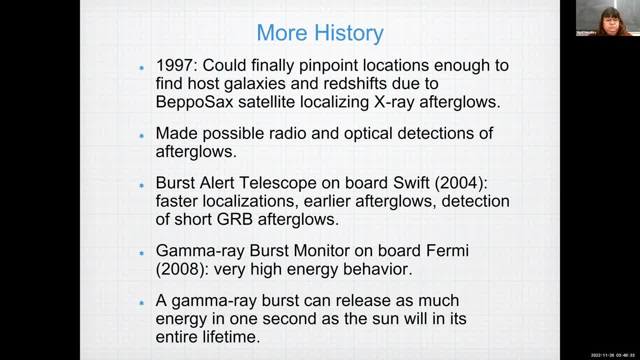 i'm in 1990, about 1997, we could start pinpointing the locations, pinpointing the locations, pinpointing the locations, um, um, um enough that we could find host, enough that we could find host, enough that we could find host galaxies, the red shifts, that was mainly. 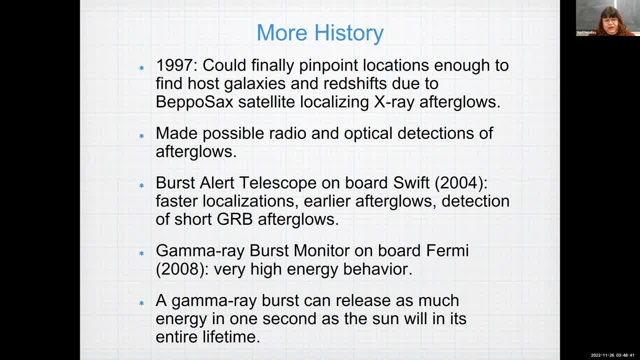 galaxies, the red shifts, that was mainly galaxies. the red shifts, that was mainly due to due to due to satellite called beppo sax, basically satellite called beppo sax, basically satellite called beppo sax, basically finding the x-ray afterglows and finding the x-ray afterglows, and 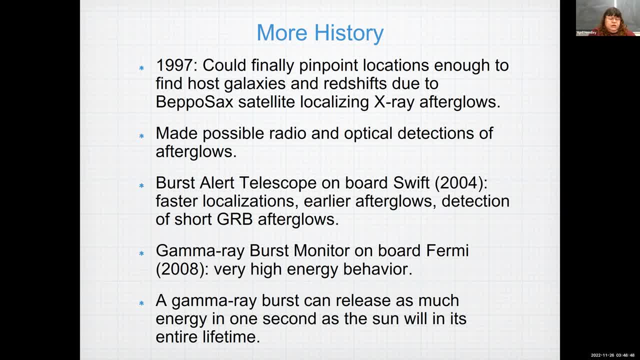 finding the x-ray afterglows and since we can get, since we can get, since we can get, basically we can get the image resolve. basically we can get the image resolve. basically we can get the image resolve, images and stuff and x-ray better than images and stuff and x-ray better than. 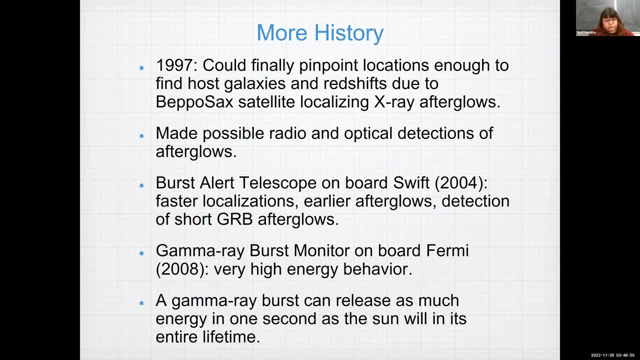 images and stuff and x-ray better than gamma rays. we could get a gamma rays. we could get a gamma rays. we could get a better location, better location, better location. so so, so, um once we could get the x-ray, um once we could get the x-ray afterglows and get the locations we 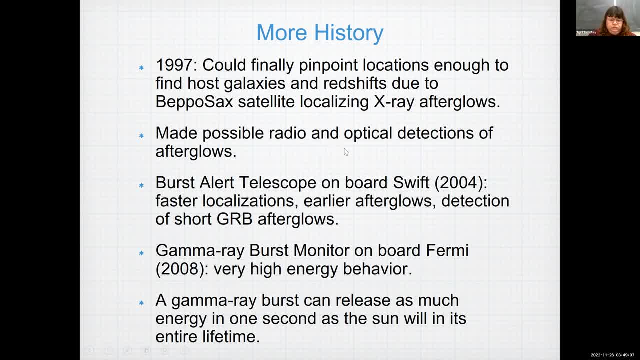 afterglows and get the locations we afterglows and get the locations we started being able to find radio and started being able to find radio and started being able to find radio and optical afterglows, optical afterglows, optical afterglows. so and eventually we could find. 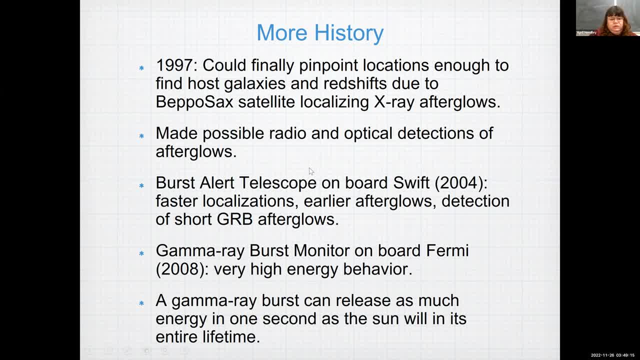 so and eventually we could find so and eventually we could find, like i said, the host galaxies and, like i said, the host galaxies and, like i said, the host galaxies, and eventually we could even find like, if, eventually we could even find like, if eventually we could even find like, if there was a company supernova we could. 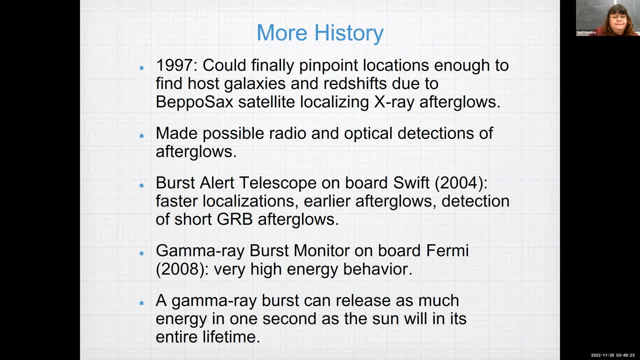 there was a company supernova we could. there was a company supernova, we could. find that too. find that too, find that too. so, um, so, um, so um. first alert telescope: one more swift first alert telescope- one more swift first alert telescope. one more swift, um, um. 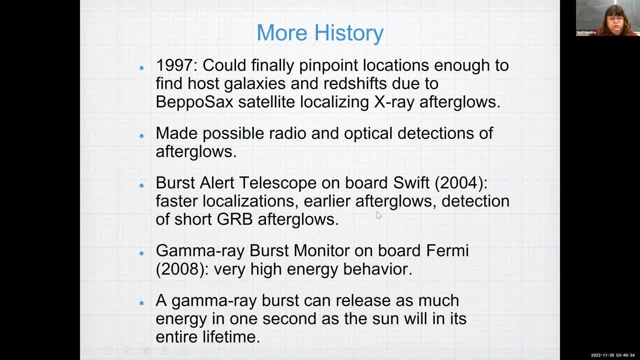 um, basically allow faster organizations, basically allow faster organizations, basically allow faster organizations. earlier after glows, earlier after glows, earlier after glows. um, um, um, could find the short dairy burst after could find the short dairy burst after. could find the short dairy burst after glows. 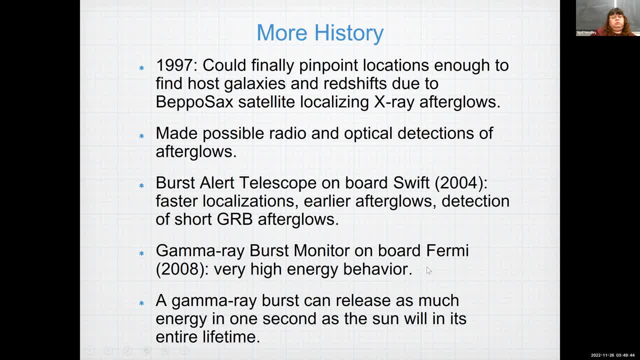 glows, glows. talk about what that means by short, and talk about what that means by short, and talk about what that means by short, and a bit, a bit, a bit. there's two types of two. there's two types of two. there's two types of two broad categories of gamma ray bursts. 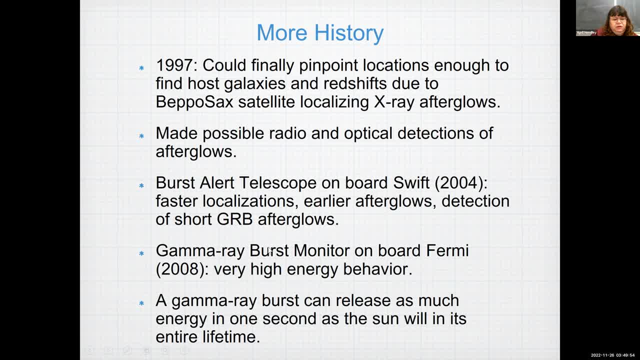 broad categories of gamma ray bursts. broad categories of gamma ray bursts um, um, um. let's see gary burst monitor on board. let's see gary burst monitor on board. let's see gary burst monitor on board fermi, which is x-ray satellite. fermi, which is x-ray satellite. 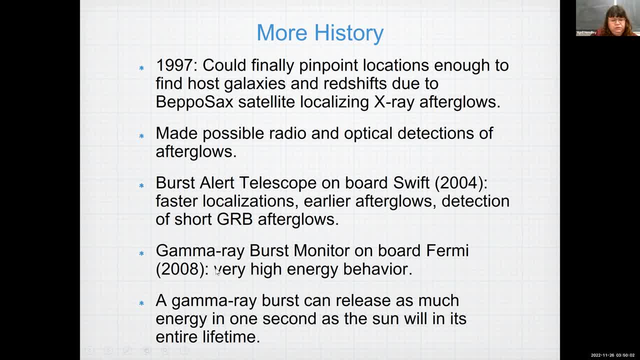 fermi, which is x-ray satellite, light, light, light or x-ray telescope or x-ray telescope or x-ray telescope, um, anyway, it could get very high energy, anyway, it could get very high energy, anyway, it could get very high energy. behavior, behavior, behavior, um, basically, basically, basically investing. 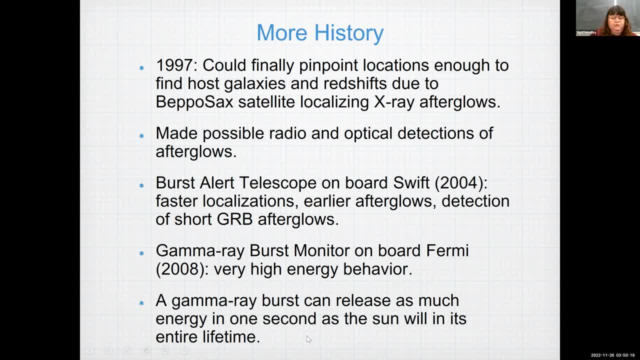 investing, investing. sorry, i just realized this doesn't sorry. i just realized this doesn't sorry. i just realized this doesn't quite fit in my habit. but again we burst. quite fit in my habit, but again we burst. quite fit in my habit, but again we burst. can release much energy in one second. 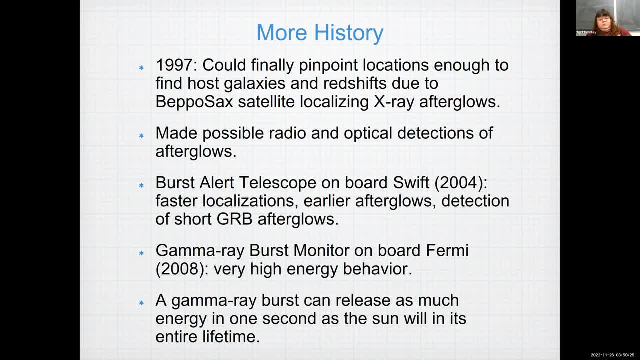 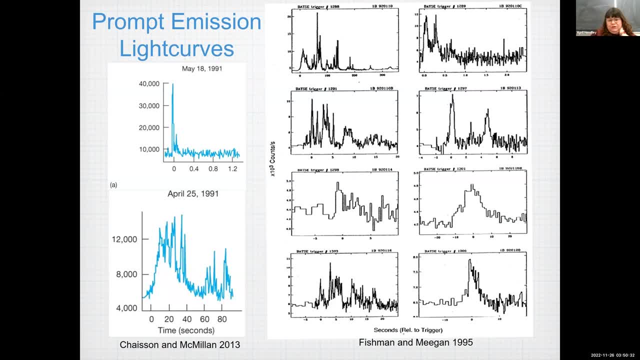 can release much energy in one second, can release much energy in one second, stumble in this entire lifetime. okay, okay, so this slide, okay so this slide, okay so this slide. don't worry about, don't worry about, don't worry about the actual numbers here. 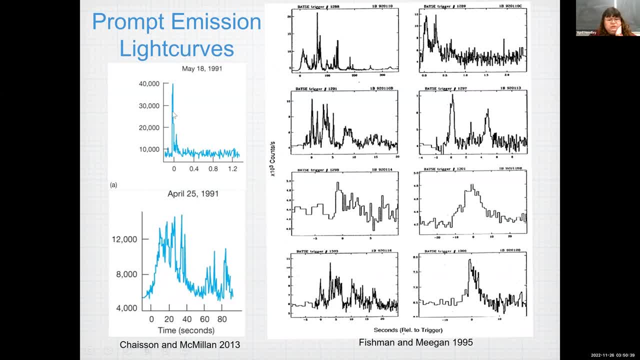 the actual numbers here. the actual numbers here. the thing i want to just point out is the thing i want to just point out is the thing i want to just point out is like, like, like, say this one, like how it has just, say this one, like how it has just. 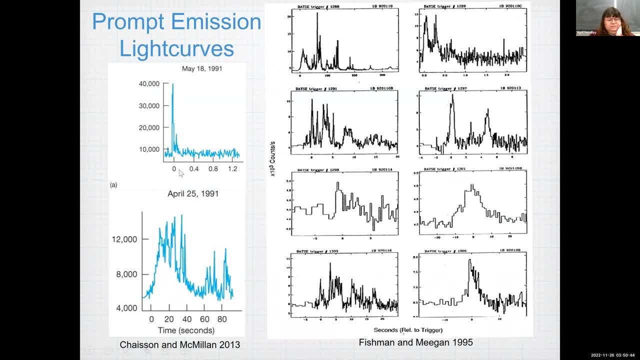 say this one like how it has just single spike. well, this one has a bunch single spike. well, this one has a bunch single spike. well, this one has a bunch of spikes. so there's variation in that you of spikes. so there's variation in that you of spikes. so there's variation in that you can see. 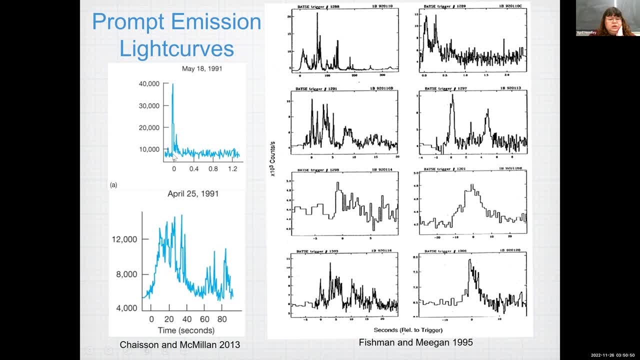 can see, can see over here. they vary in the number of over here. they vary in the number of over here. they vary in the number of spikes too. spikes too, spikes too. the time, the duration. some are really the time the duration, some are really the time the duration. some are really short, some are a lot longer. 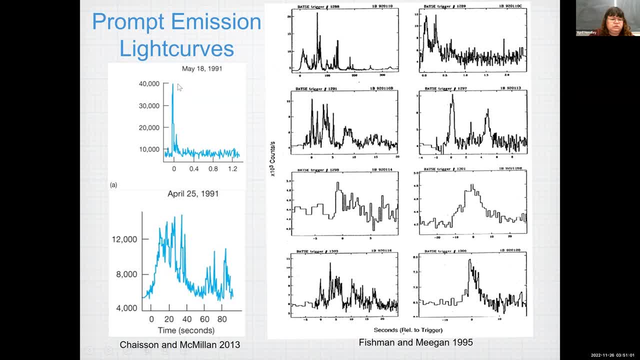 short, some are a lot longer. short, some are a lot longer. some- the this is in terms of counts. some, the this is in terms of counts. some, the this is in terms of counts. some are, some are. some are brighter, some are dimmer. there's quite a. 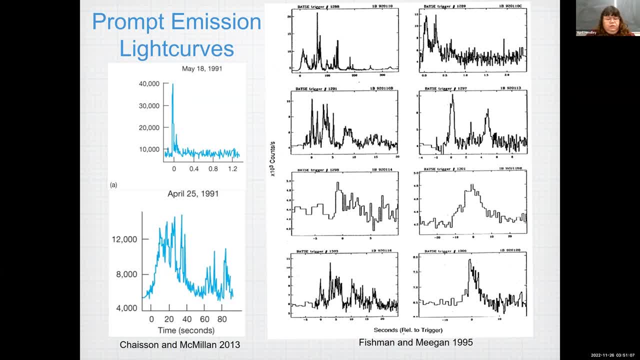 brighter, some are dimmer. there's quite a brighter, some are dimmer. there's quite a bit of variation in bit of variation in bit of variation in how bright, how long. what's on the, how bright, how long. what's on the, how bright, how long, what's on the vertical axis here? 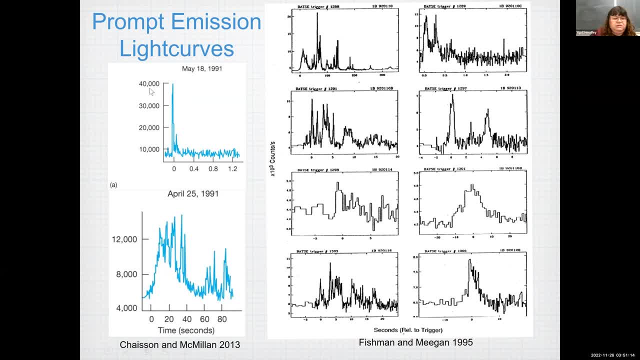 vertical axis here, vertical axis here, uh, i mean, uh, i mean uh. i mean it's basically intensity like counts per. it's basically intensity like counts per. it's basically intensity like counts per second, second, second. so so why it is so low in uh? so so why it is so low in uh? 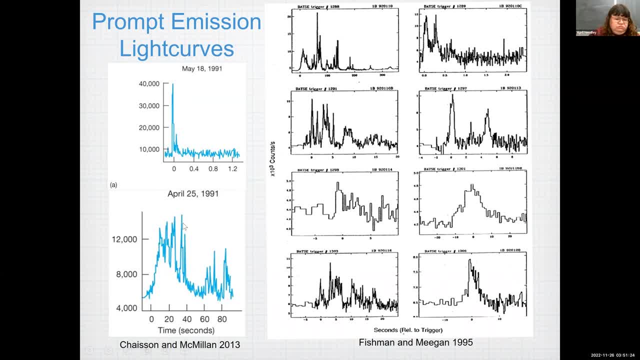 so so why it is so low in? uh, in the bottom one, in the bottom one, in the bottom one, just it varies from burst to burst, so just it varies from burst to burst. so just it varies from burst to burst. so, and this one it may turn out to be, 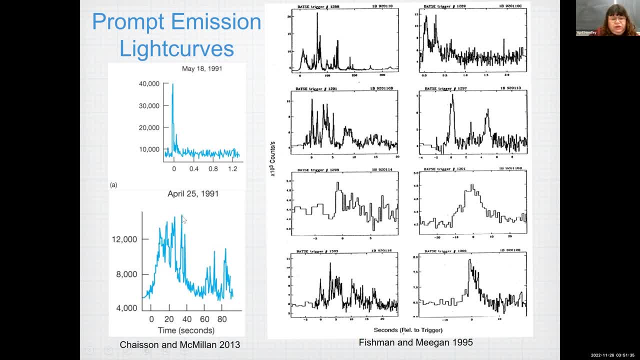 and this one it may turn out to be, and this one it may turn out to be, overalls, overalls, overalls, like since it's longer drawn out, it like since it's longer drawn out, it like, since it's longer drawn out, it could be, could be. 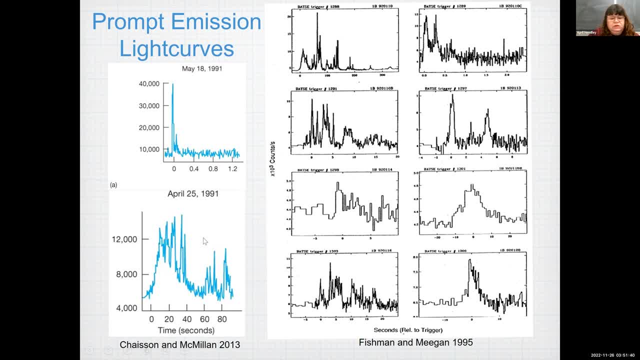 could be more similar overall. just longer drawn. more similar overall, just longer drawn. more similar overall, just longer drawn out. it's just okay out. it's just okay. out, it's just okay. there's just a bunch of variability. there's just a bunch of variability. there's just a bunch of variability between them. 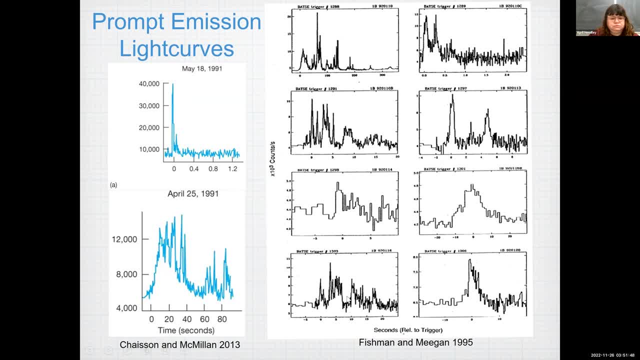 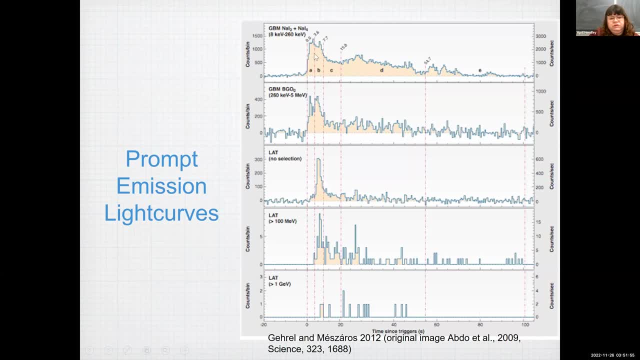 between them, between them. so there were some patterns. this here shows this is for one burst. this here shows this is for one burst. this here shows this is for one burst. and you see the and you see the and you see the difference in the in different parts of. 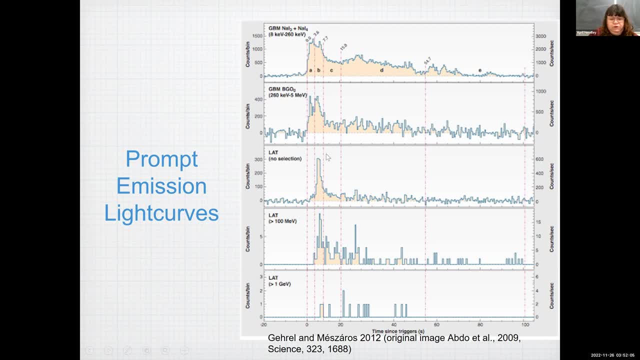 difference in the in different parts of difference in the in different parts of the spectrum too, for the spectrum too. for the spectrum too. for just the prompt for the actual gamma, just the prompt for the actual gamma, just the prompt for the actual gamma: reverse itself emission, reverse itself emission. 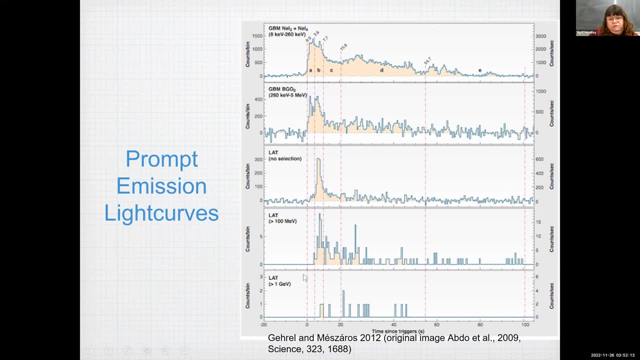 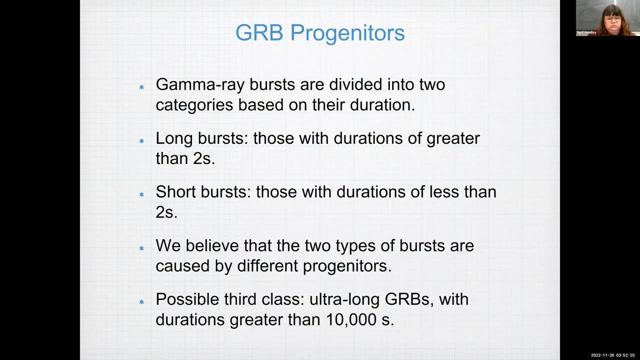 reverse itself: emission, the afterglow, the afterglow, the afterglow, so so, so i can even vary in, so i can even vary in, so i can even vary in different parts of the spectrum. well anyway, well anyway, well, anyway, the thing i was most interested in, 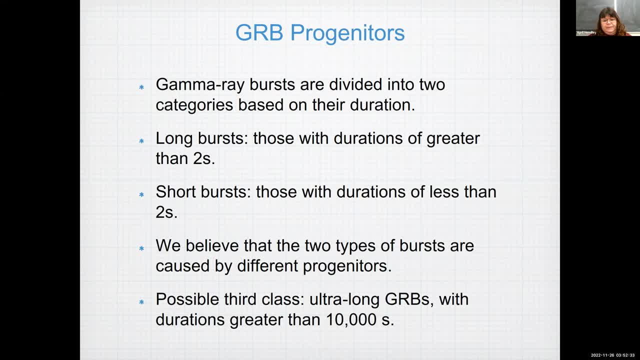 the thing i was most interested in. the thing i was most interested in is basically how we get the gamma, is basically how we get the gamma, is basically how we get the gamma reverse, basically what causes them, basically what causes them, basically what causes them. anyway, gamma burst are divided into two. 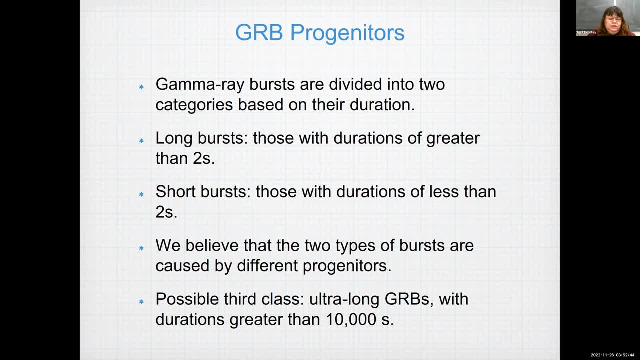 anyway, gamma burst are divided into two. anyway, gamma burst are divided into two categories: categories, categories. it's based on their duration. it's based on their duration. it's based on their duration. the um. long bursts which have durations greater. long bursts which have durations greater. long bursts which have durations greater than two seconds. 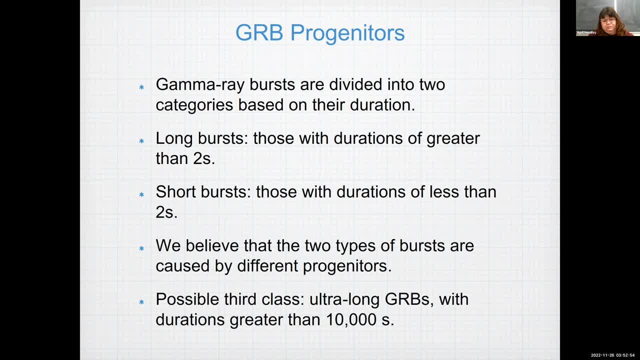 than two seconds, than two seconds and a short burst with durations less and a short burst with durations less and a short burst with durations less than two seconds than two seconds, than two seconds. so it's basically the dividing lines: two seconds, it's kind of a dividing lines two seconds, it's kind of a. 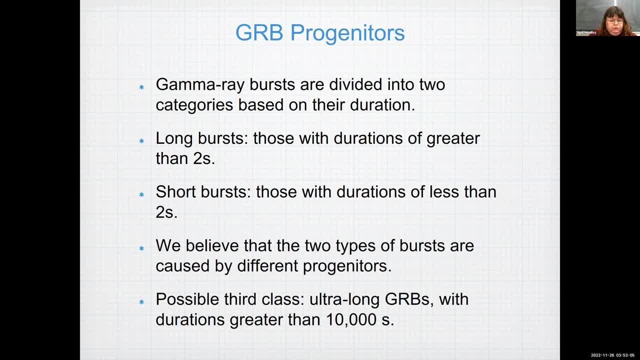 dividing lines two seconds. it's kind of a some to some debate about whether that's some to some debate about whether that's some to some debate about whether that's the most appropriate place to put the, the most appropriate place to put the, the most appropriate place to put the dividing line, because it 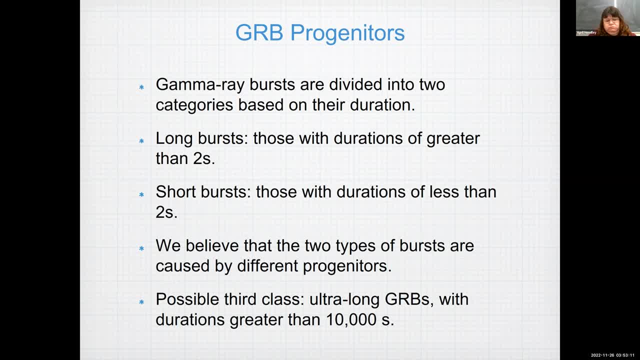 dividing line, because it dividing line, because it um, um, um, like, could it be like. could it be like, could it be a bit above two, bit below two. so the two a bit above two, bit below two, so the two a bit above two, bit below two, so the two just kind of. 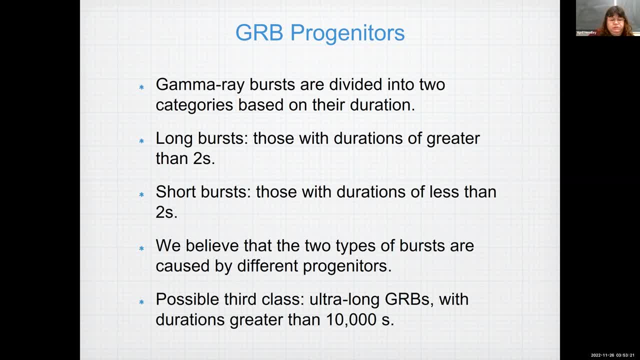 something, some people say somewhat something, some people say somewhat something, some people say somewhat. arbitrary of the second choice of two. arbitrary of the second choice of two. arbitrary of the second choice of two seconds to divide them, seconds to divide them, seconds to divide them. so so, so, but anyway, i think that 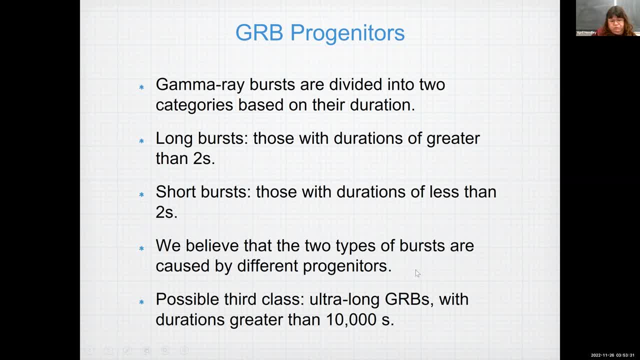 but anyway i think that, but anyway i think that two categories in general are caused by two categories in general are caused by. two categories in general are caused by two different progenitors, two different progenitors, two different progenitors. there's also a possible third class with 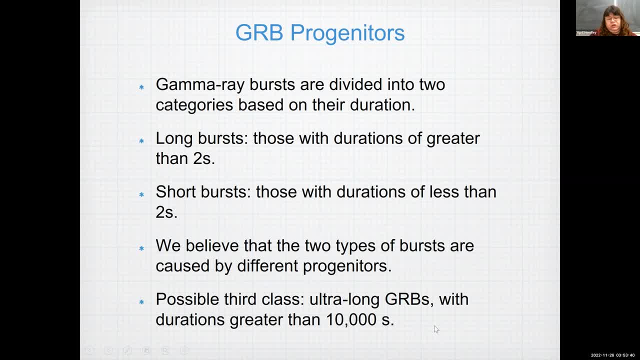 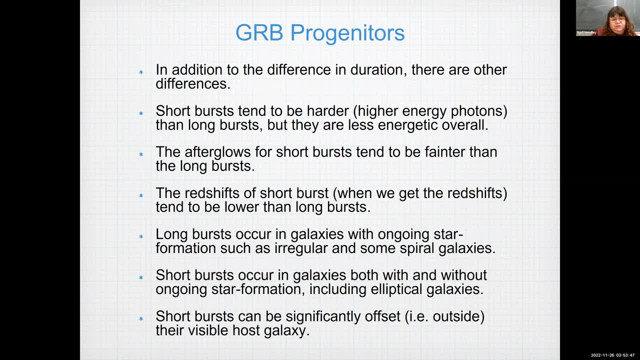 there's also a possible third class with. there's also a possible third class with ultra long gallery bursts whose ultra long gallery bursts, whose ultra long gallery bursts whose durations are longer than 10 000 durations are longer than 10 000 durations are longer than 10 000 seconds. 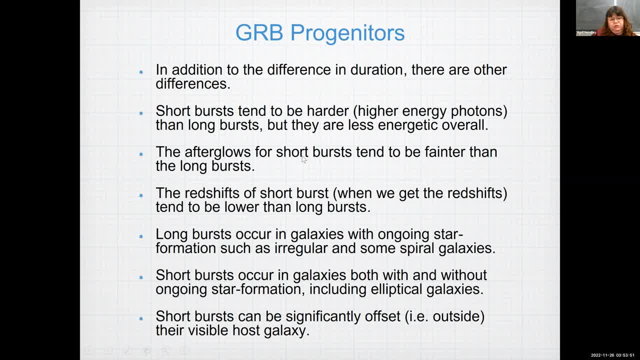 some other differences between them and some other differences between them and some other differences between them. and all this goes to what causes them. the short bursts tend to be the short bursts tend to be. the short bursts tend to be harder. higher energy photons, but less harder. higher energy photons, but less. 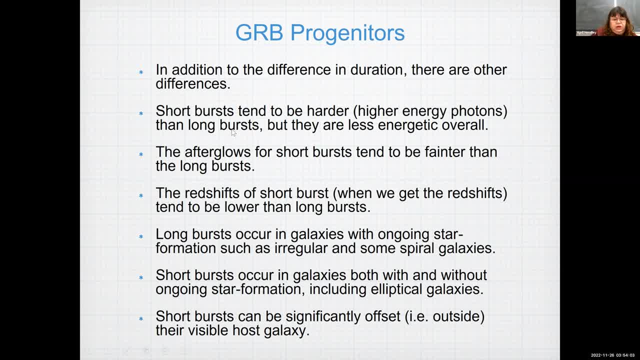 harder, higher energy photons, but less energetic overall. um, um, um. and the afterglows for short bursts tend, and the afterglows for short bursts tend, and the afterglows for short bursts tend to be fainter, to be fainter, to be fainter. so short bursts tend to be higher energy. 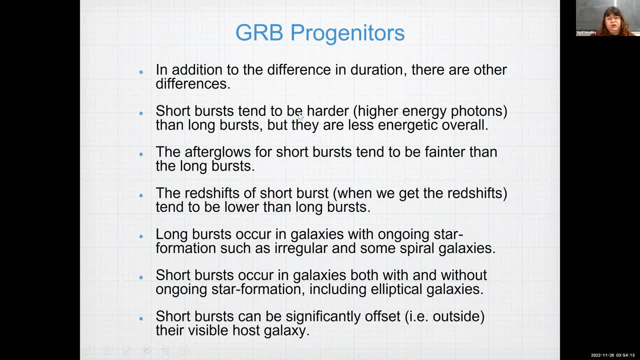 so short bursts tend to be higher energy. so short bursts tend to be higher energy photons, but less energetic. the long burst photons, but less energetic the long burst photons, but less energetic the long burst tend to be tend to be tend to be lower energy photons, but overall more. 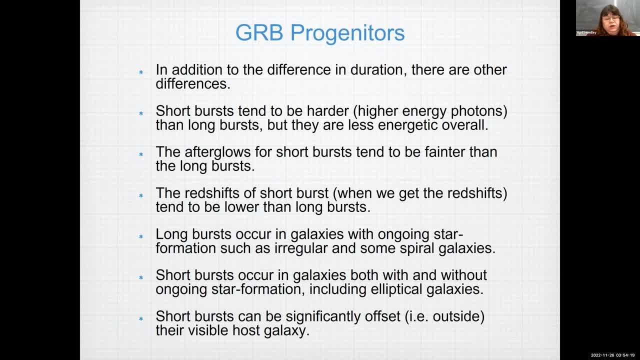 lower energy photons but overall more. lower energy photons but overall more energetic. when you energetic, when you energetic, when you look at how much of an entire event, look at how much of an entire event, look at how much of an entire event. so, so, so, um, um, um. the red shift is short burst, so we get. 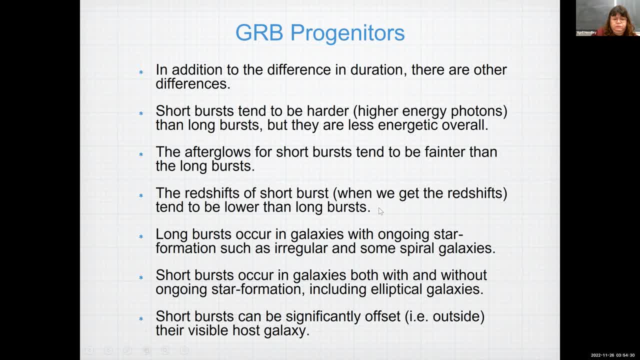 the red shift is short burst, so we get. the red shift is short burst, so we get. the red shifts tend to be lower than the. the red shifts tend to be lower than the. the red shifts tend to be lower than the long burst. that means those short bursts. 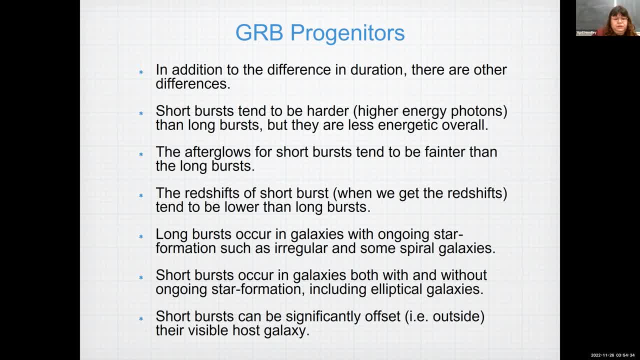 long burst. that means those short bursts tend to be closer to us. long bursts- generally occurring galaxies, with generally occurring galaxies, with generally occurring galaxies with ongoing star formation, the regular ongoing star formation, the regular ongoing star formation, the regular galaxies, some spiral galaxies, galaxies, some spiral galaxies, galaxies, some spiral galaxies, and they generally occur. and they generally occur. and they generally occur closer to the areas with the ongoing star, closer to the areas with the ongoing star, closer to the areas with the ongoing star formation, while the short bursts tend to while the short bursts tend to, while the short bursts tend to occur in galaxies. 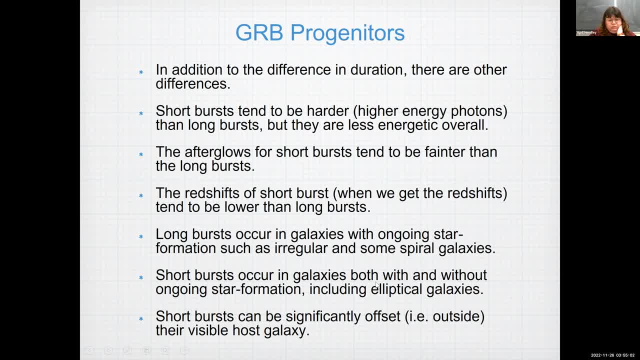 occur in galaxies. occur in galaxies, both some with ongoing, both some with ongoing, both some with ongoing star formation, star formation. star formation, but a lot of times when ones without, but a lot of times when ones without, but a lot of times when ones without ongoing star formation. 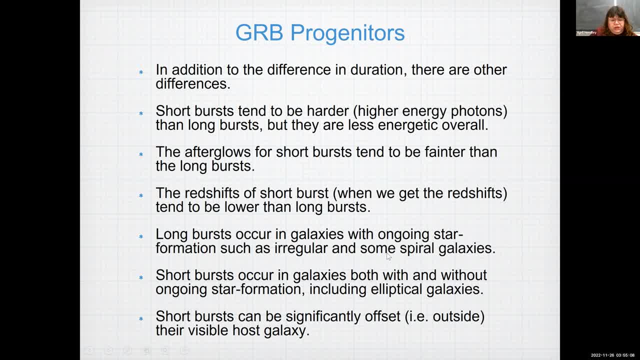 ongoing star formation. ongoing star formation, including elliptical galaxies. including elliptical galaxies. including elliptical galaxies: um, they also tend to be, or they also. um they also tend to be, or they also. um they also tend to be, or they also can be significantly offset. can be significantly offset. 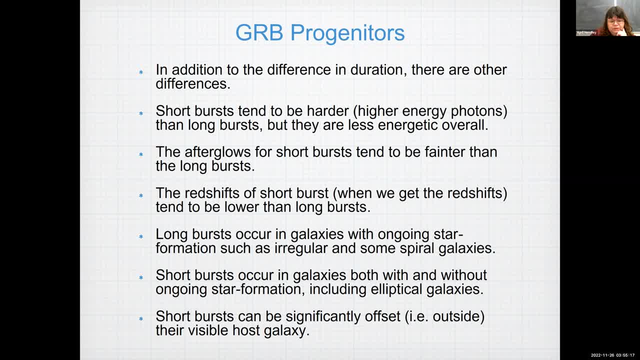 can be significantly offset from the host galaxy, basically outside from the host galaxy, basically outside from the host galaxy, basically outside the visible host galaxy, the visible host galaxy, the visible host galaxy. what this means or what this indicates, what this means or what this indicates, what this means or what this indicates, is that the long bursts 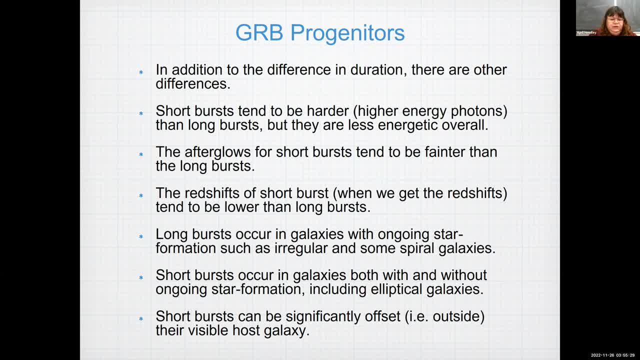 is that the long bursts is that the long bursts are basically related to something, that are basically related to something, that are basically related to something that occurs. occurs occurs like with stars that's not very long, like with stars that's not very long, like with stars that's not very long lived, or something like that. 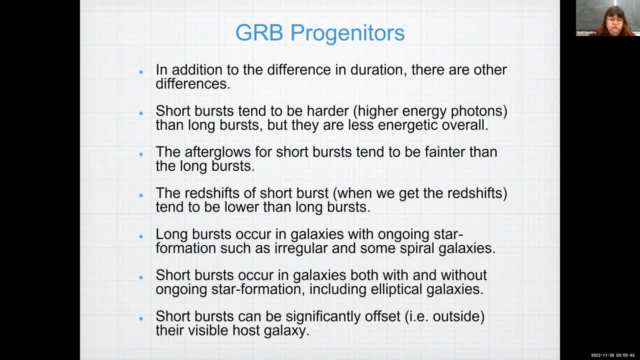 lived or something like that. lived or something like that. um while the short burst, if it's um, while the short burst, if it's um while the short burst, if it's something new: stars could be stars, something new, stars could be stars, something new: stars could be stars. that's a lot longer. lived, that's gotten. 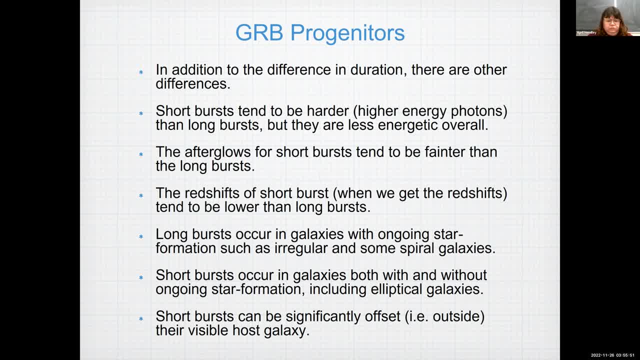 that's a lot longer lived. that's gotten. that's a lot longer lived, that's gotten. no, no, no, basically not no longer in areas with, basically not no longer in areas with basically not no longer, in areas with the ongoing star formation, the ongoing star formation, the ongoing star formation. example of what i mean is um. 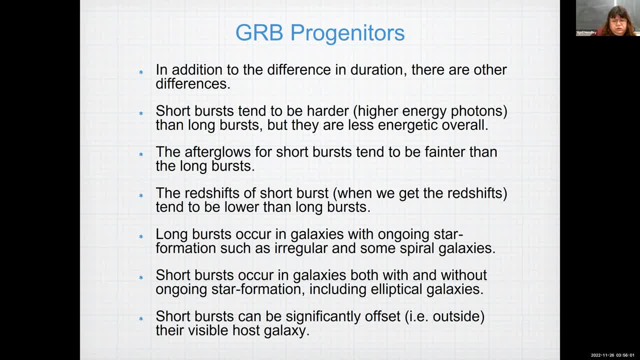 example of what i mean is um. example of what i mean is um. the massive, most massive stars, the massive, most massive stars, the massive, most massive stars, will live their entire lives and still will live their entire lives and still will live their entire lives and still be fairly close to where they formed in. be fairly close to where they formed in. be fairly close to where they formed in areas with ongoing star formations. areas with ongoing star formations. areas with ongoing star formations. low mass stars. they live so much longer. low mass stars. they live so much longer. low mass stars, they live so much longer that they. 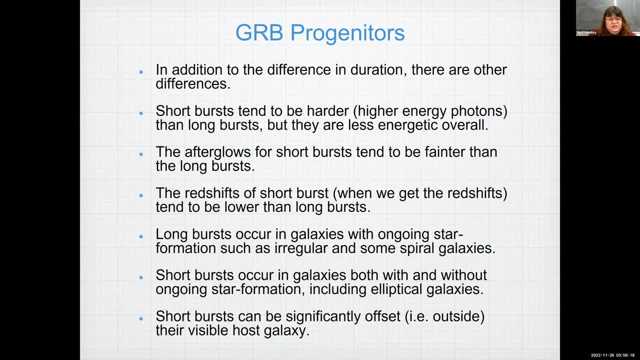 that they, that they, by the time they end up their lives, they by the time they end up their lives, they by the time they end up their lives, they may not be, may not be, may not be in the same area where they formed at in the same area where they formed at. 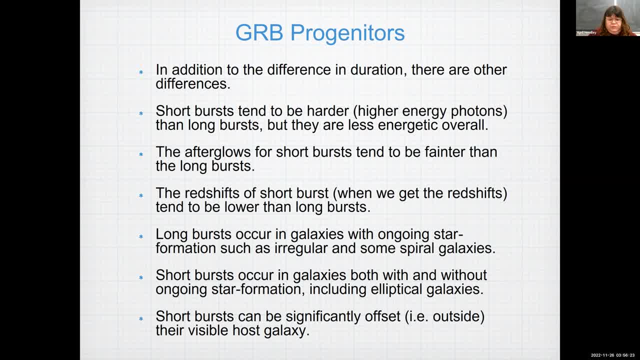 in the same area where they formed at all, they could be all they could be, all they could be. an area that had little star, an area that had little star, an area that had little star formations. so, or in the case like elliptical galaxy, or in the case like elliptical galaxy, 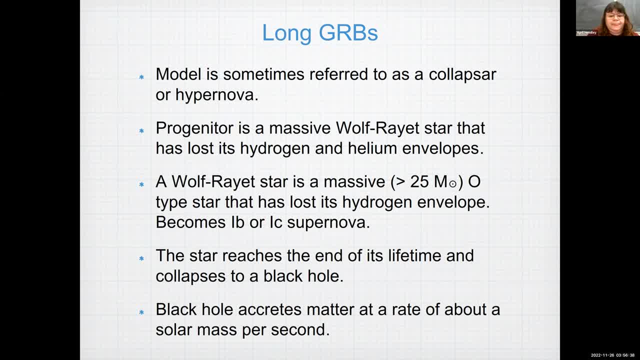 or in the case like elliptical galaxy, galaxy that no longer has an active star, galaxy that no longer has an active star, galaxy that no longer has an active star formation, okay. so, basically the galaxies that are okay. so, basically the galaxies that are okay. so basically the galaxies that are already formed. if you were looking from 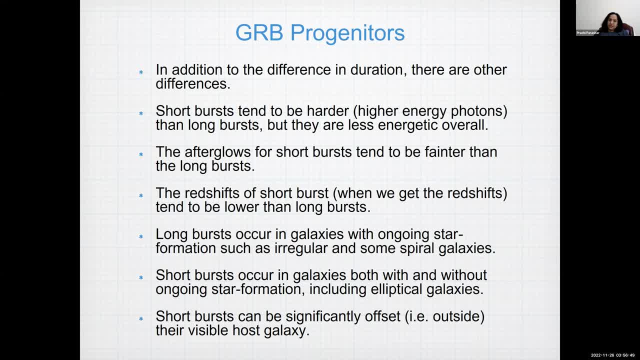 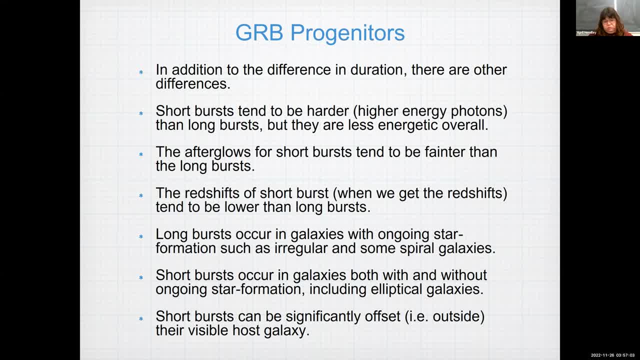 those new stars, those new stars, still for this new star formation going, still for this new star formation going, still for this new star formation, going on on on. we get the long ones, we get the long ones, we get the long ones. the short ones would be galaxies like. 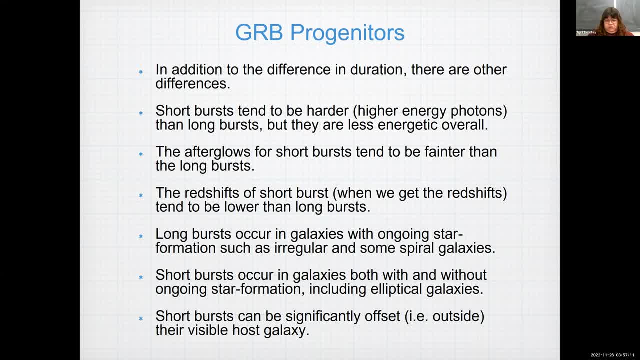 the short ones would be galaxies like. the short ones would be galaxies like more like ellipticals, more like ellipticals, more like ellipticals. or can or can or can. where there's no new star formation, where there's no new star formation, where there's no new star formation, where it's just stars, that's just. 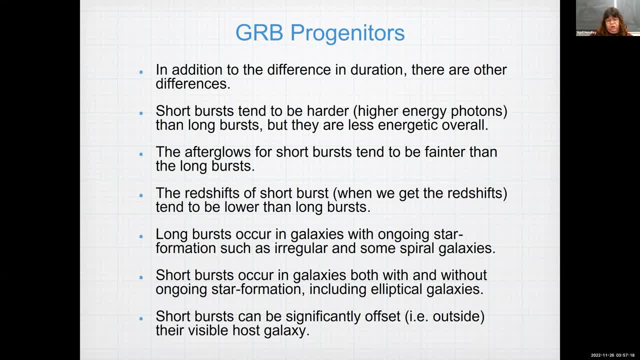 where it's just stars. that's just where it's just stars. that's just getting older, getting older, getting older. well, you have the longer, oh so longer. well, you have the longer, oh so longer. well, you have the longer, oh so longer ones are when the ongoing star. 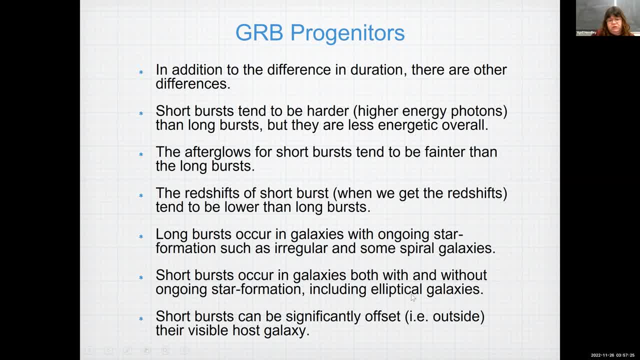 ones are when the ongoing star ones are, when the ongoing star formation is happening. yeah, formation is happening. yeah, formation is happening. yeah, well, the short ones, well, the short ones, well, the short ones, short ones can be for this ongoing star. short ones can be for this ongoing star. 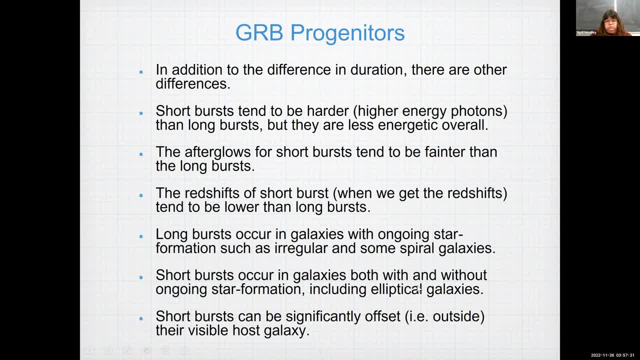 short ones can be for this ongoing star formation. but they also occur in places formation. but they also occur in places formation. but they also occur in places where there's not. isn't it like slightly confusing here? isn't it like slightly confusing here? isn't it like slightly confusing here, because the gamma ray burst is on the 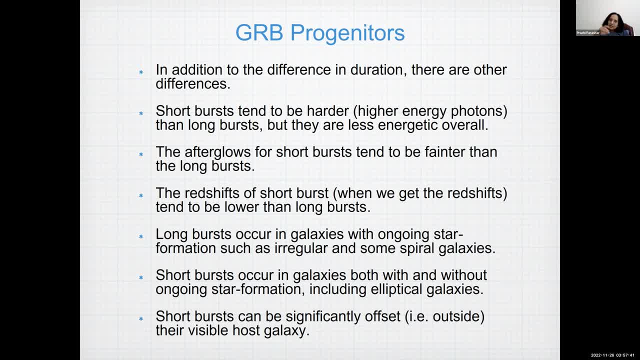 because the gamma ray burst is on the, because the gamma ray burst is on the cycle of basically, cycle of basically, cycle of basically, um, when the stars are towards the end, um, when the stars are towards the end, um, when the stars are towards the end of their cycle, right. 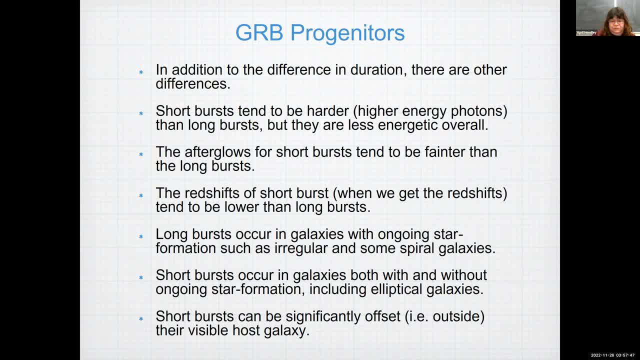 of their cycle, right of their cycle, right. one type, one type, one type. that's the thing. that's the thing. that's the thing: the long burst falling at the short, the long burst falling at the short, the long burst falling at the short, bursts, bursts, bursts. actually a different. 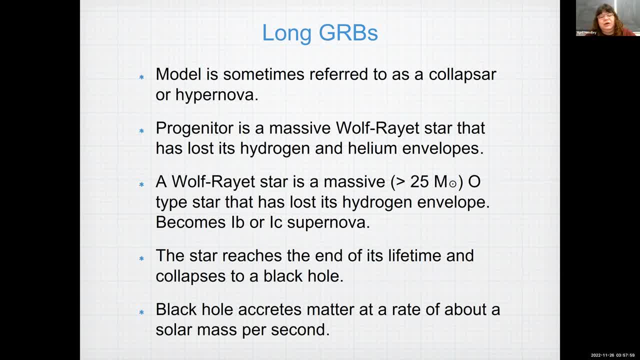 okay, so, um so, um so, um so the long burst. sometimes it's called class or a, sometimes it's called class or a, sometimes it's called class or a hypernova, hypernova, hypernova, they're basically a massive star, that they're basically a massive star that. 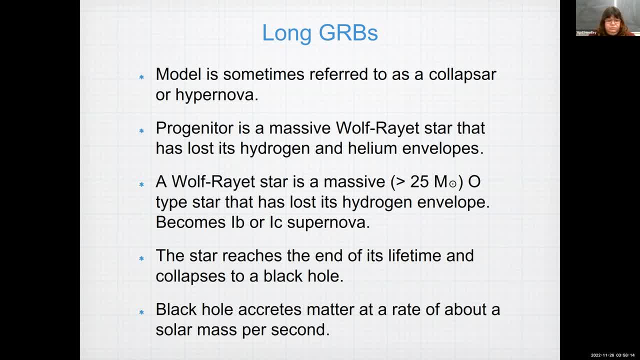 they're basically a massive star that reaches the end of its life. reaches the end of its life. reaches the end of its life generally, generally, generally. a massive what's called wolf rayet star, a massive what's called wolf rayet star, a massive what's called wolf rayet star that's lost to hydrogen helium envelopes. 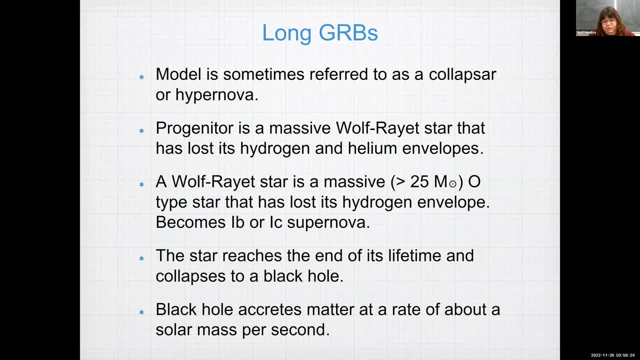 that's lost to hydrogen helium envelopes, that's lost to hydrogen helium envelopes. basically, wolf rayet star is more than basically wolf rayet star is more than basically wolf rayet star is more than about 25 times the mass of sun- about 25 times the mass of sun. 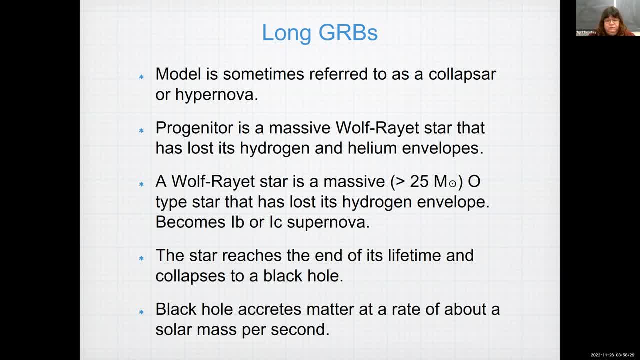 about 25 times the mass of sun. it's um one of the most massive type. it's um one of the most massive type. it's um one of the most massive type: stars, stars, stars, o stars um, o stars um o stars um. and the wolf rayet. stars lost its. 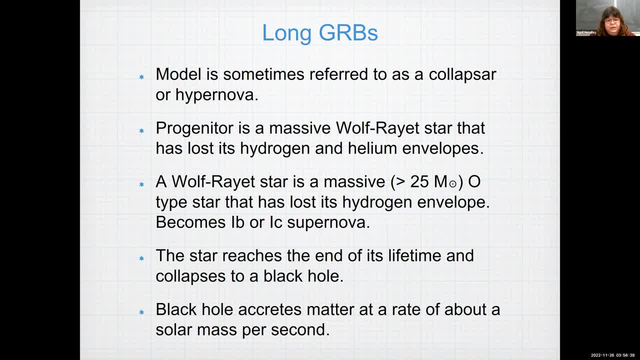 and the wolf rayet stars lost its and the wolf rayet stars lost its. hydrogen and hydrogen and hydrogen, and, like i said, the helium too, like i said the helium too, like i said the helium too, feel completely once, basically, when it feel completely once, basically when it. 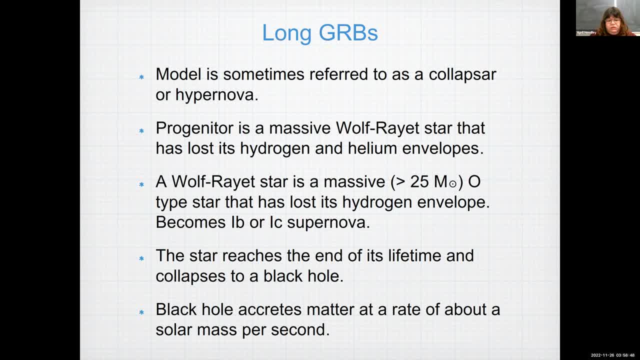 feel completely once. basically, when it gets the iron core, gets the iron core, gets the iron core, it becomes either type 1b or type 1c. it becomes either type 1b or type 1c. it becomes either type 1b or type 1c. supernova. 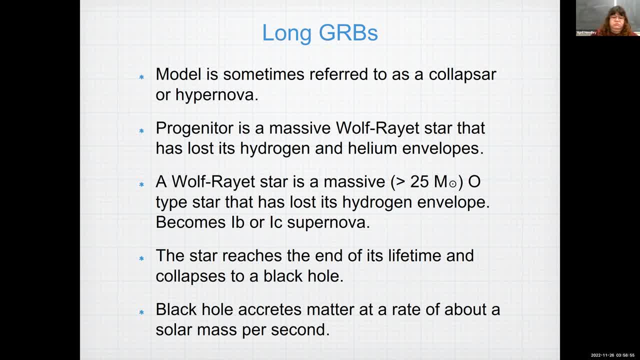 um, anyway, once the super assuming that anyway, once the super assuming that anyway, once the super assuming that happens, the core collapses to a black, happens, the core collapses to a black, happens, the core collapses to a black hole, hole, hole and the black hole retreats matter and the black hole retreats matter. 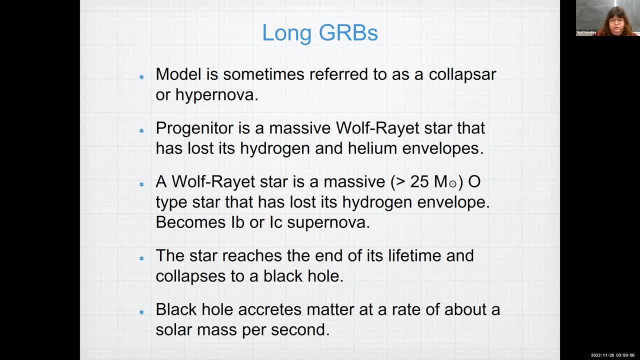 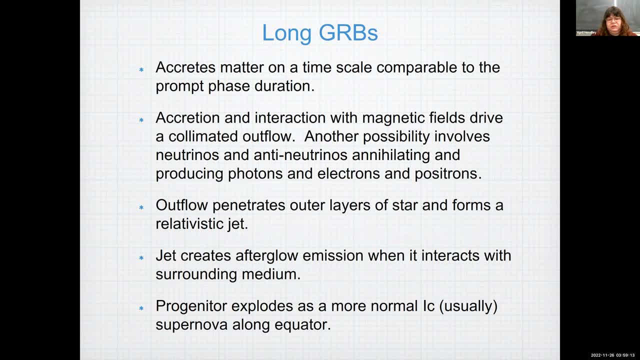 and the black hole retreats matter initially, at a rate about initially, at a rate about initially, at a rate about a solar mass per second and the amount of time it treats, and the amount of time it treats and the amount of time it treats matter at that rate is 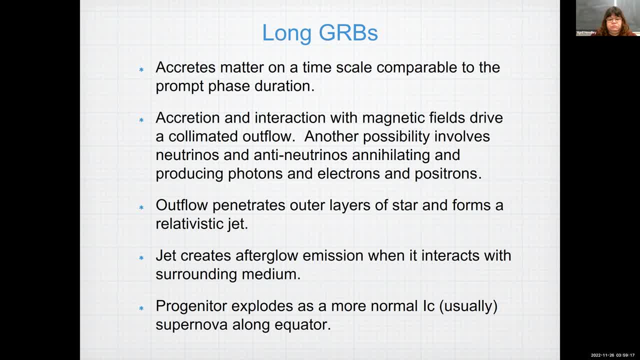 matter at that rate is: matter at that rate is basically comparable to how long the basically comparable to how long the basically comparable to how long the gamma ray bursts last anyway, um, you have, anyway, um, you have, anyway, um, you have recreation interaction with the next, recreation interaction with the next. 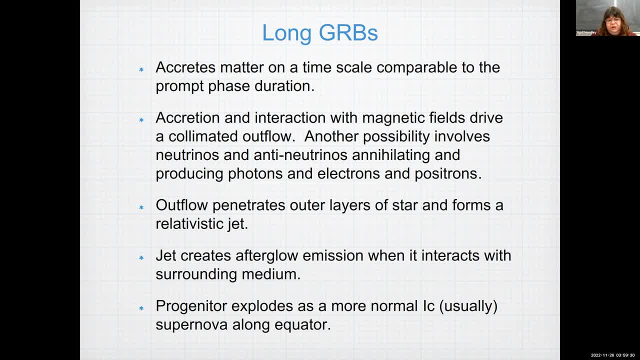 recreation, interaction with the next fields, fields, fields, and you get this collimated outflow and you get this collimated outflow and you get this collimated outflow. um other possibility. people have other possibility. people have other possibility. people have given is basically neutrinos and 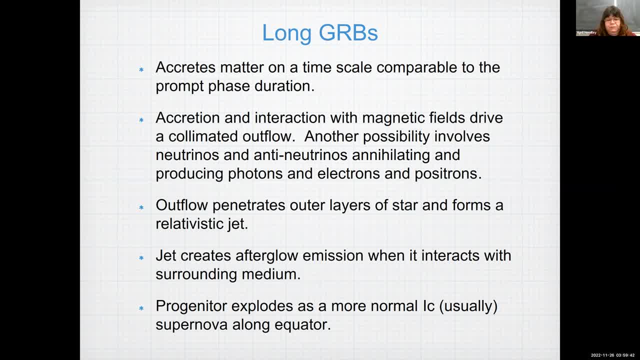 given is basically neutrinos and given is basically neutrinos and neutrinos, annihilating producers, neutrinos, annihilating producers, neutrinos, annihilating producers, photons, electrons, photons, electrons, photons, electrons, positrons, and positrons and positrons, and so and basically so, and basically so, and basically eventually somehow producing a. 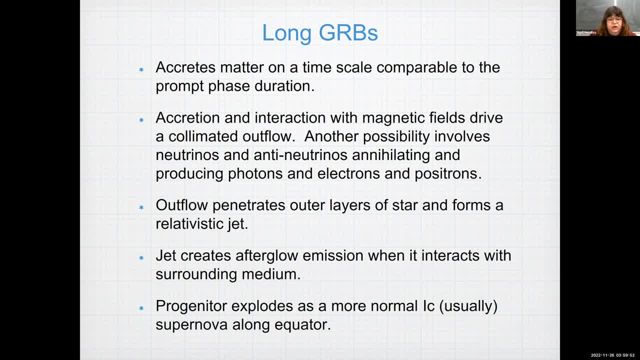 eventually somehow producing a, eventually somehow producing a relativistic jet, relativistic jet, relativistic jet, so um that jet, so um that jet, so um that jet penetrates it out of layers of star and penetrates it out of layers of star and penetrates it out of layers of star and eventually interacts with the interstellar. eventually interacts with the interstellar. eventually interacts with the interstellar medium, medium medium, the afterglow is produced when it, the afterglow is produced, when it the afterglow is produced when it interacts with interstellar medium, the interacts with interstellar medium: the. 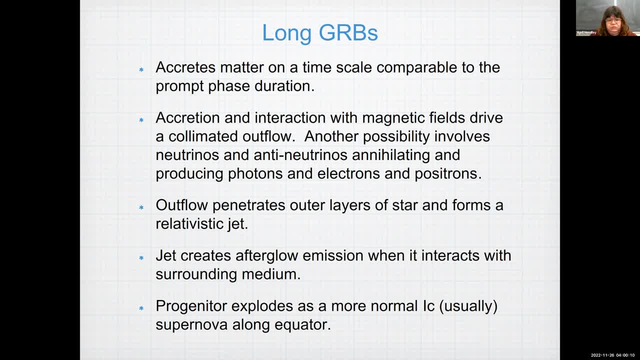 interacts with interstellar medium. the prompt dimension again reversed itself. prompt dimension again reversed itself. prompt dimension again reversed itself, is basically, is basically, is basically occurs before, occurs before, occurs before and when and when and when, with interactions before that, with interactions before that, with interactions before that, like with the star and with the jet. 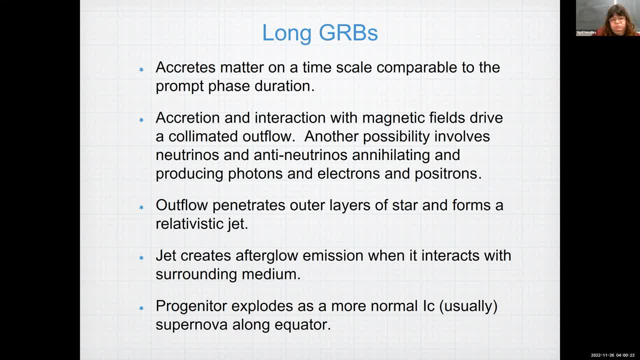 like with the star and with the jet, like with the star and with the jet itself. this interaction itself, this interaction itself, this interaction, it was basically, it was basically, it was basically. they call internal shocks inside the jet, they call internal shocks inside the jet, they call internal shocks inside the jet. that goes on. 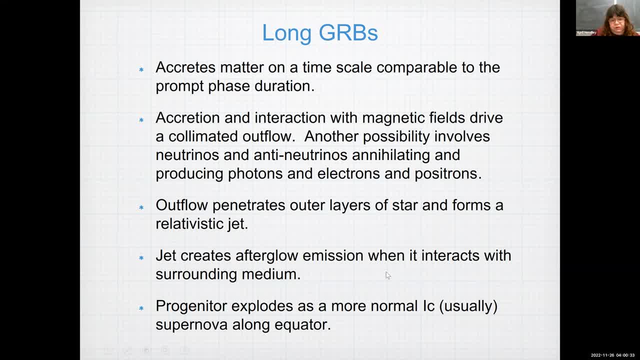 um, if you're looking at one of these stars, if you're looking at one of these stars, if you're looking at one of these stars along the equator, you'd see a more normal. along the equator, you'd see a more normal. along the equator, you'd see a more normal. 1c supernova usually. 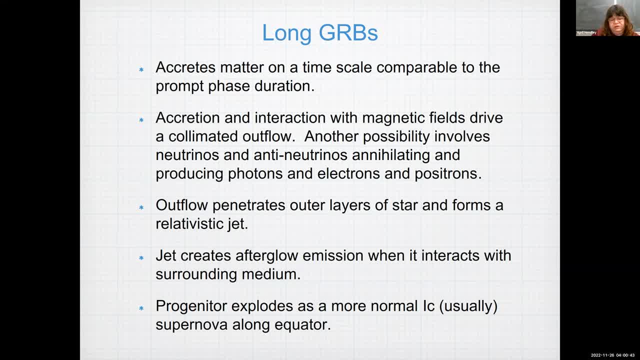 1c supernova, usually 1c supernova, usually um, um, um, in fact, in fact, in fact, along the equator, you might not see the. along the equator, you might not see the. along the equator, you might not see the gamma reversed, gamma reversed. 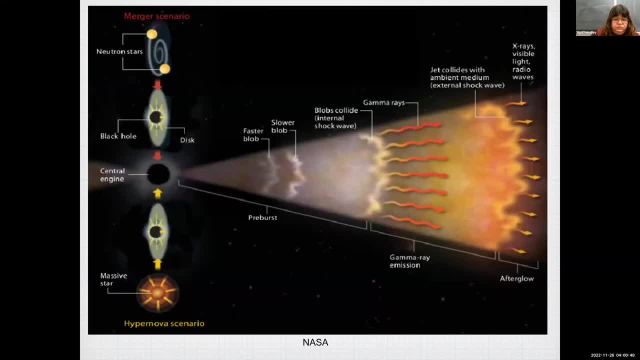 gamma reversed. so because, so the one for a massive stars, so the one for a massive stars, so the one for a massive stars? here you have the massive star, the core. here you have the massive star, the core, here you have the massive star, the core, collapse, collapse. 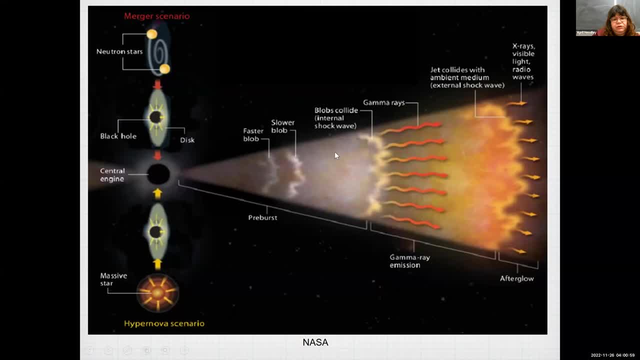 collapse like on the creation disk, like on the creation disk, like on the creation disk. and then you get the jet, and then you get the jet, and then you get the jet, and you get, and you get, and you get inside the jet the these shock inside the jet, the these shock. 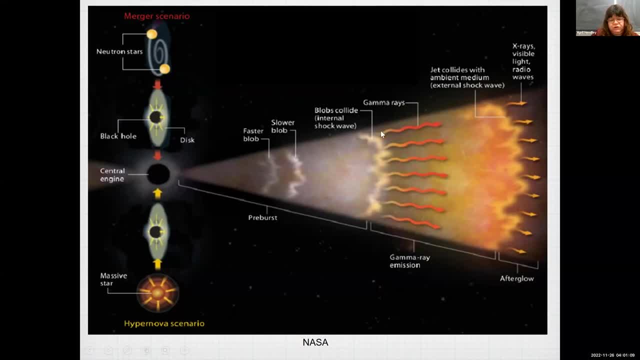 inside the jet, the, these shock blobs, some moving faster, something blobs, some moving faster, something blobs, some moving faster, something subtle, where they collide with each subtle, where they collide with each subtle, where they collide with each other, from that other, from that other, from that, then the material is moving. 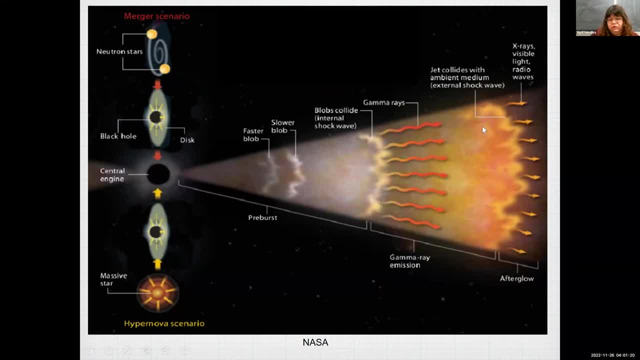 then the material is moving. then the material is moving relativistic speeds, eventually runs. relativistic speeds, eventually runs. relativistic speeds eventually runs into the aerostatic medium, into the aerostatic medium, into the aerostatic medium. get more shocks, what's called external. get more shocks, what's called external. 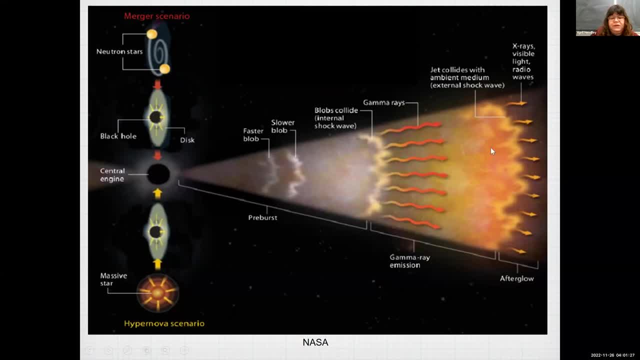 get more shocks- what's called external shocks- and shocks and shocks, and that produces the afterglow, and since that produces the afterglow, and since that produces the afterglow, and since it's slowing down over time, the it's slowing down over time, the. 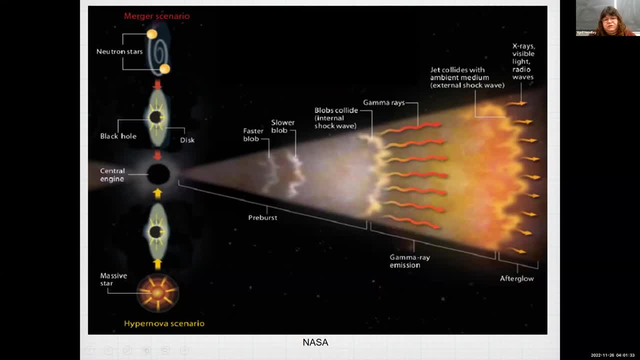 it's slowing down over time. the afterglow tends to start off in the afterglow. tends to start off in the afterglow, tends to start off in the x-rays, x-rays, x-rays eventually, eventually, eventually, become longer and longer wavelengths become longer and longer wavelengths. 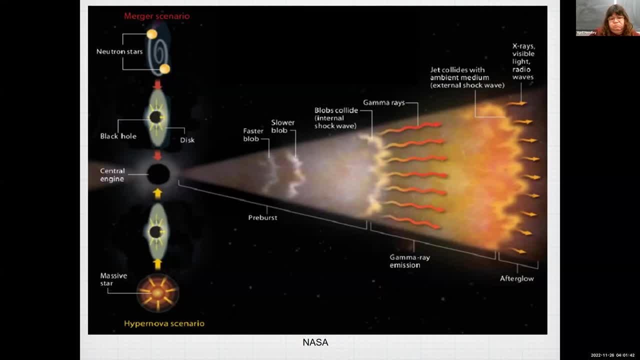 become longer and longer wavelengths. so it's kind of so, it's kind of so, it's kind of. the radio tends to be at the. the radio tends to be at the. the radio tends to be at the lighter part of the lighter part of the lighter part of the spectrum. yeah, yeah, afterglow. so 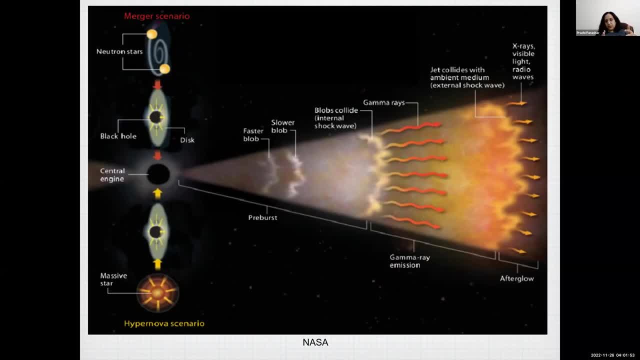 but uh, so the point is on that figure. but uh, so the point is on that figure. but uh, so the point is on that figure, like i mean. are you saying that as it like? i mean, are you saying that as it like? i mean, are you saying that as it goes, uh, 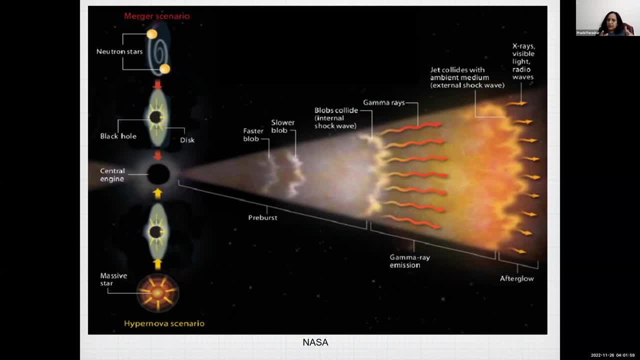 goes uh, goes uh, from gamma ray emission to afterglow, from gamma ray emission to afterglow, from gamma ray emission to afterglow, like all the gamma rays will be like i don't know, like i, i think i mean. i don't know like i, i think i mean. 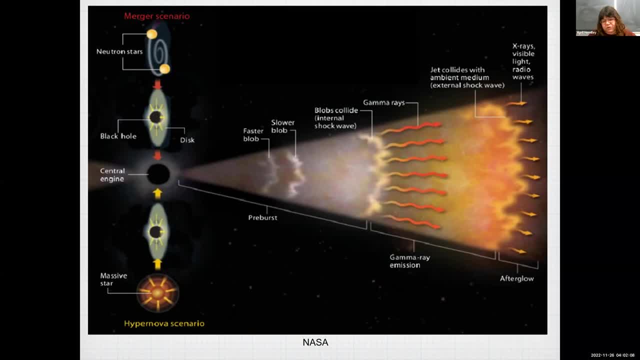 i don't know like i. i think i mean to say uh, to say uh, to say uh at the very beginning of the afterglow, at the very beginning of the afterglow, at the very beginning of the afterglow, you get gamma ray afterglow too. 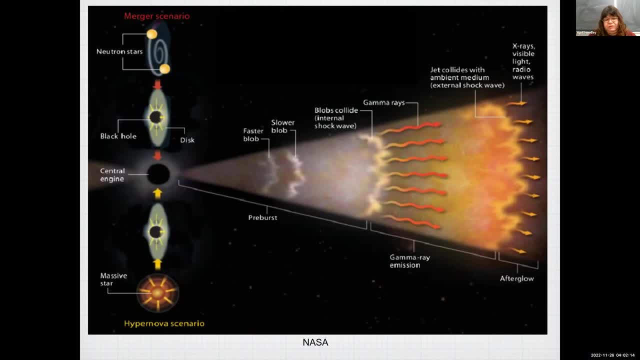 you get gamma ray afterglow too. you get gamma ray afterglow too, and then you get, and then you get, and then you get the x-rays, but the x-rays, but the x-rays, but so so, so, like so, these are basically photon right. like so, these are basically photon right. 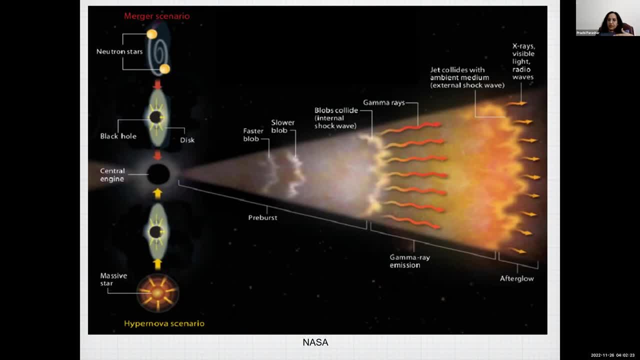 like. so these are basically photon right: very high energy photons, very high energy photons, very high energy photons. what are they colliding with to generate? what are they colliding with to generate? what are they colliding with to generate the lower energy photons, or something, the lower energy photons, or something. 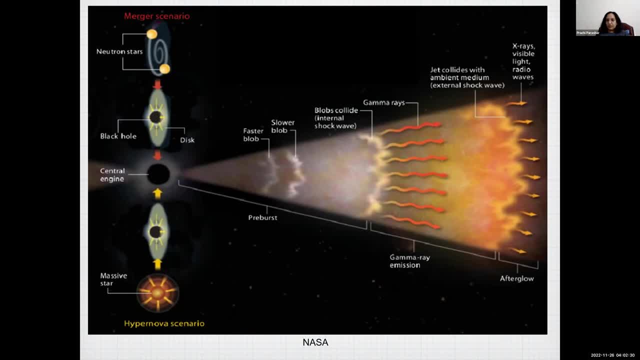 the lower energy photons, or something like: how are they creating the x-rays? like: how are they creating the x-rays? like: how are they creating the x-rays? or like later, or like later, or like later parts of their spectrum? you think of parts of their spectrum you think of? 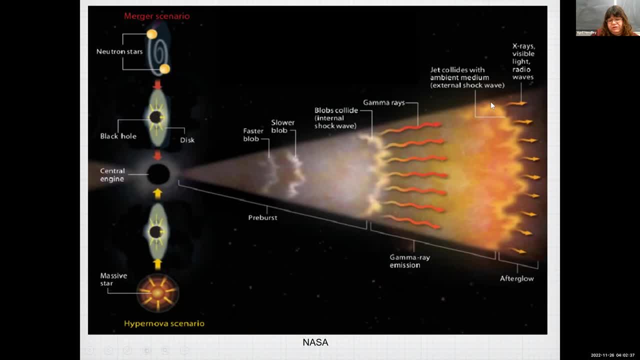 parts of their spectrum. you think of this. besides the photons, you also still this. besides the photons, you also still this: besides the photons, you also still have material itself. electrons have material itself. electrons have material itself, electrons, protons and stuff, protons and stuff, protons and stuff moving outward that's crashing into. 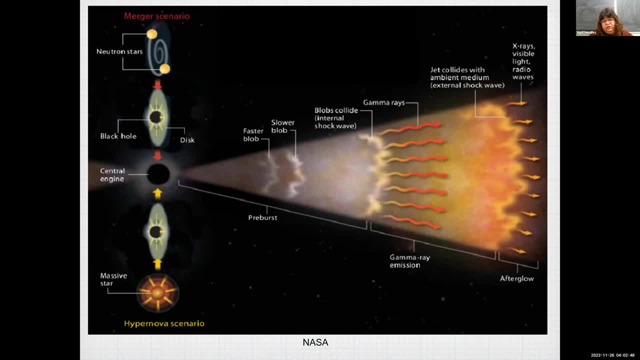 moving outward, that's crashing into moving outward, that's crashing into basically the medium surrounding the, basically the medium surrounding the, basically the medium surrounding the star of stuff, the star ejected earlier. star of stuff. the star ejected earlier. star of stuff. the star ejected earlier, before it went supernova. 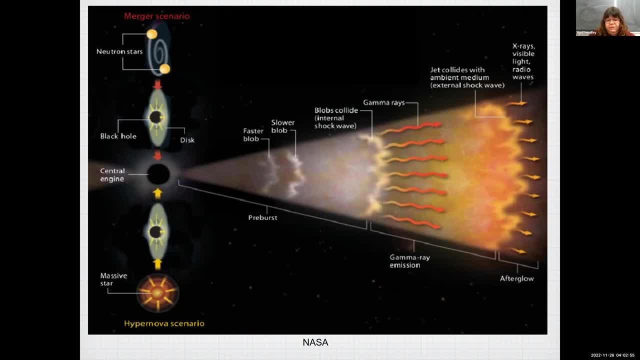 before it went supernova, before it went supernova, or if it's an area that's dusty in, or if it's an area that's dusty in, or if it's an area that's dusty in space where you have space, where you have space where you have that's enough interstellar medium around. 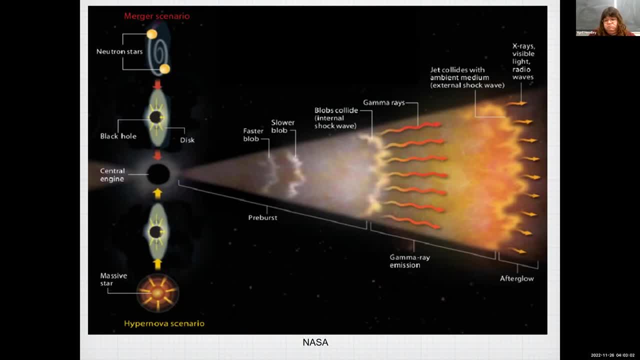 that's enough interstellar medium around. that's enough interstellar medium around it. it could be crashing into that and it it could be crashing into that and it it could be crashing into that and basically, just, basically, just, basically, just them running into that less stuff, them running into that less stuff. 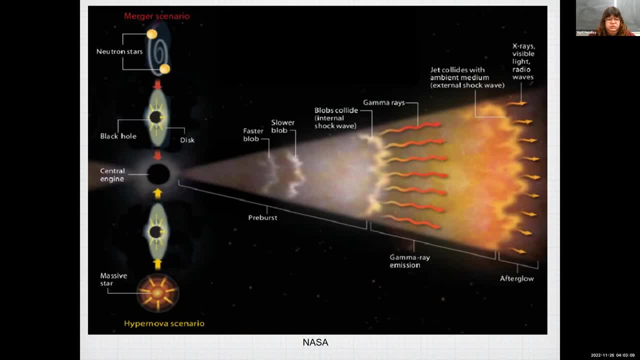 them running into that less stuff. so you get, so you get, so you get. let's see synchrotron. let's see synchrotron. let's see synchrotron. um, um, um, some, some, some something inverse compton or something, something inverse compton or something. 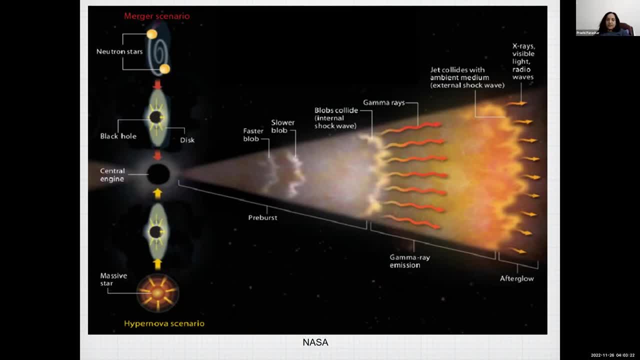 something inverse compton or something. so is it? is it so? is it? is it so? is it? is it okay to say that the very massive stars, okay to say that the very massive stars, okay to say that the very massive stars which are going to turn into black holes? 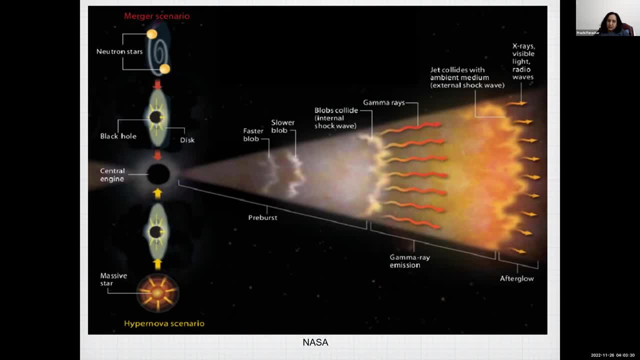 which are going to turn into black holes, which are going to turn into black holes, you will never get the very high. you will never get the very high. you will never get the very high. energetic gamma ray burst from them. energetic gamma ray burst from them. energetic gamma ray burst from them. it will always be like the later part of 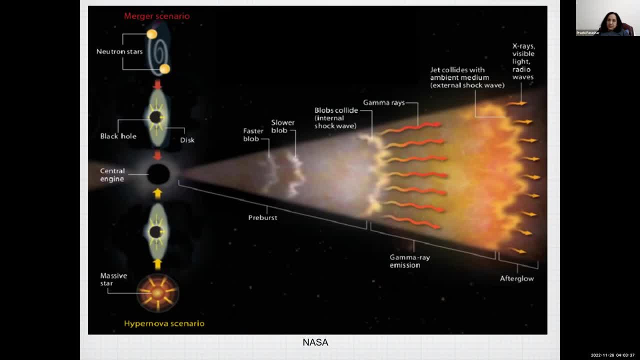 it will always be like the later part of, it will always be like the later part of the spectrum, the spectrum, the spectrum, or or or like. am i like missing something like the like? am i like missing something like the like? am i like missing something like the picture is kind of showing in such a? 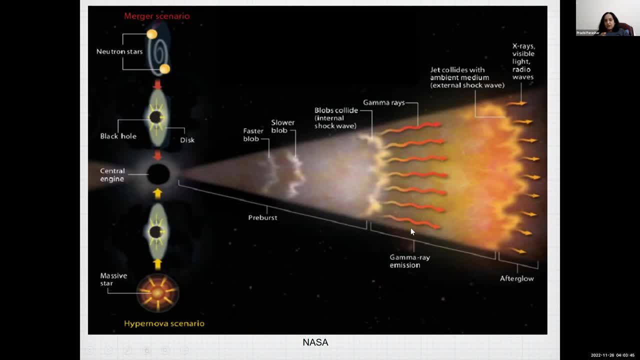 picture is kind of showing in. such a picture is kind of showing in such a fashion that there is a very high fashion, that there is a very high fashion, that there is a very high energetic gamma ray burst, but eventually energetic gamma ray burst but eventually energetic gamma ray burst, but eventually they will die down. and it will be like 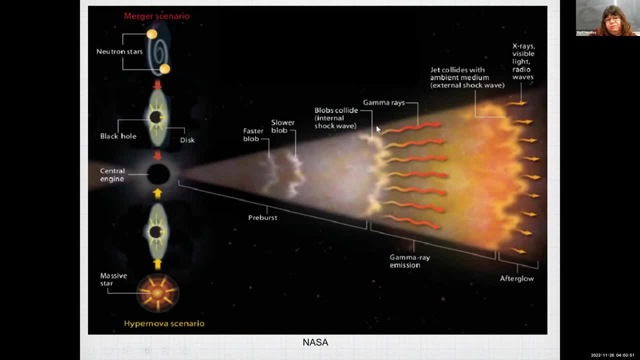 they will die down and it will be like they will die down and it will be like lower, lower, lower i think. i think i think here, like this part here is occurring here, like this part here is occurring here, like this part here is occurring earlier in time than this part, 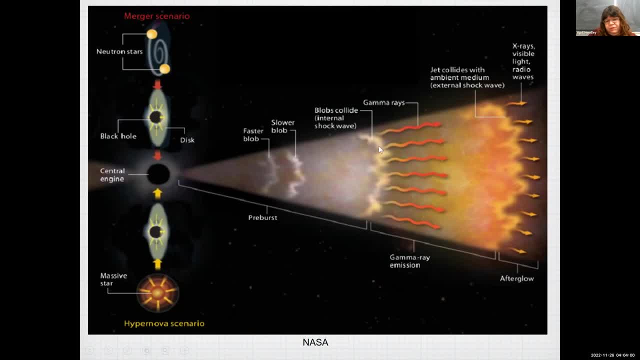 earlier in time than this part, earlier in time than this part. so this, so this, so this part that would be emitted before the part that would be emitted before the part that would be emitted before the material had reached material had reached, material had reached this far out. basically, this is: 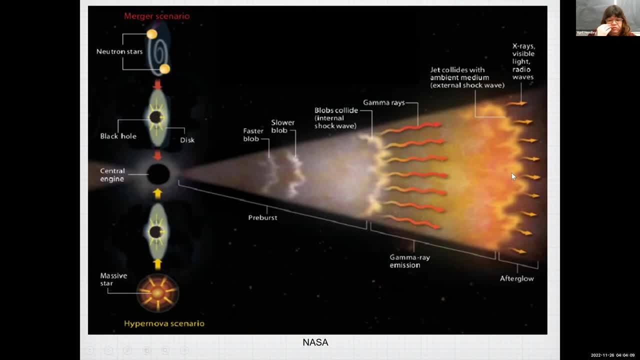 this far out. basically, this is this far out. basically, this is as you go left to right. it's basically as you go left to right. it's basically as you go left to right. it's basically times increasing, too times increasing, too times increasing too. yeah, yeah, yeah. so, in other words, 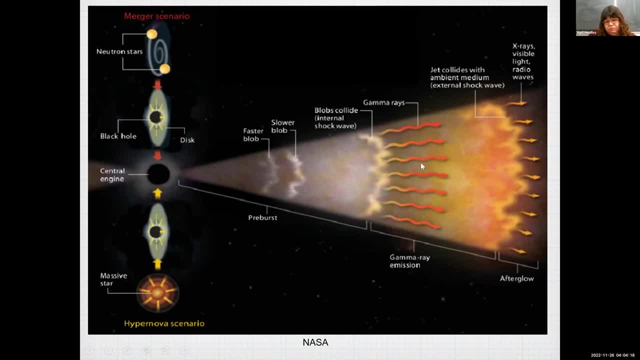 so, in other words, so, in other words, this: the gamma ray burst here might be this. the gamma ray burst here might be this: the gamma ray burst here might be able to escape, able to escape, able to escape before the material runs into vanishtela, before the material runs into vanishtela. 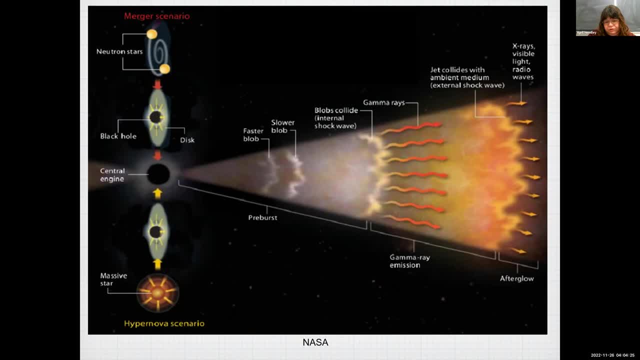 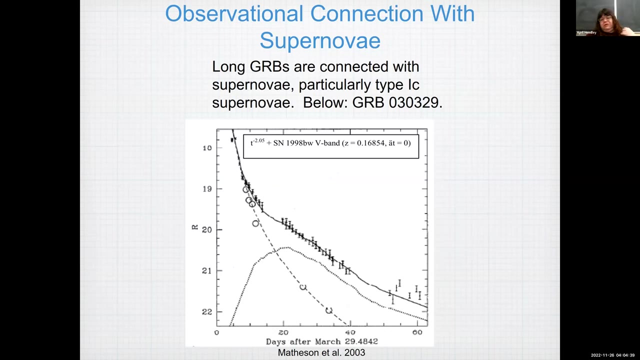 before the material runs into vanishtela medium and produces the medium, and produces the medium and produces the afterglow. the next, the next, the next couple of slides is couple of slides is couple of slides is it's on a long burst and evidence they 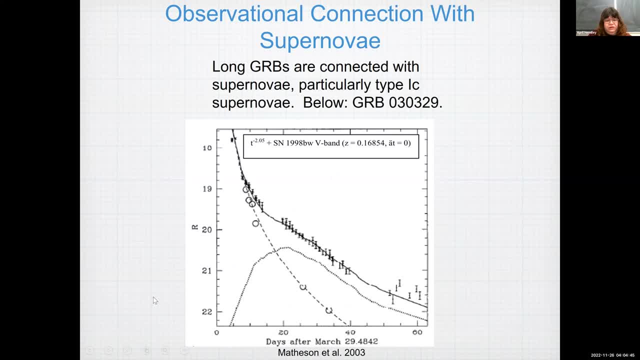 it's on a long burst and evidence they it's on a long burst and evidence they are connected. some evidence they are are connected. some evidence they are are connected. some evidence they are connected. supernova: there's been connected. supernova: there's been connected. supernova: there's been um. i'm going to look at one in particular. 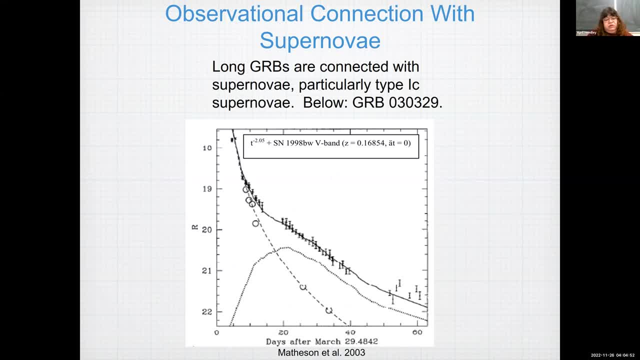 um, i'm going to look at one in particular. um, i'm going to look at one in particular- there's been other ones- since there's been other ones, since there's been other ones, since that shows a connection to supernova, but that shows a connection to supernova, but 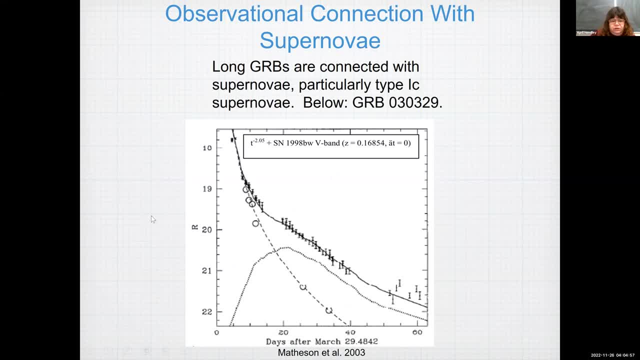 that shows a connection to supernova. but um, um, um, this is one, this is one, this is one. battery burst oh three, oh three. two. battery burst oh three, two battery burst oh three, two. nine. it occurred um march 29: nine. it occurred um march 29. 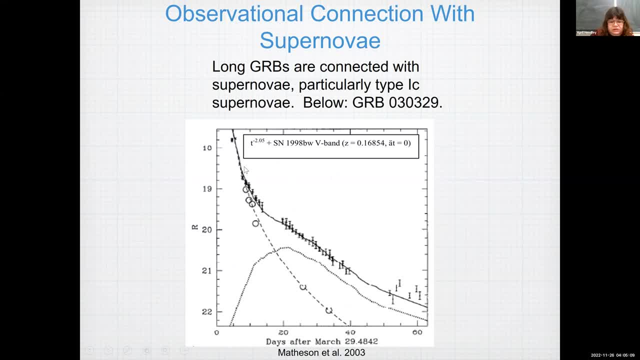 nine. it occurred um march 29, 2003.. 2003. 2003. anyway, these curves here, just the dashed. anyway, these curves here, just the dashed. anyway, these curves here, just the dashed one. one one would be for, would be for, would be for um. 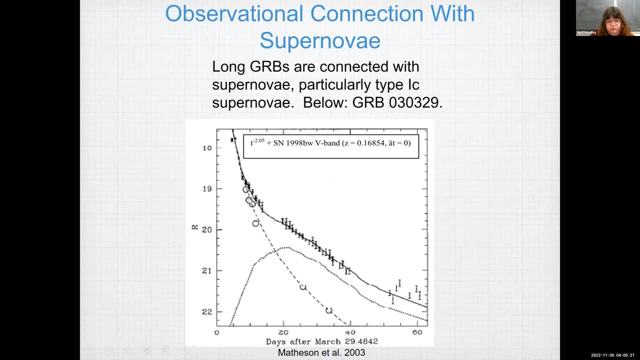 um, um, basically just the gallery burst, basically just the gallery burst, basically just the gallery burst after the glow itself, how much light it after the glow itself, how much light it after the glow itself, how much light it puts out, puts out, puts out. so it's basically, you think, intensity. 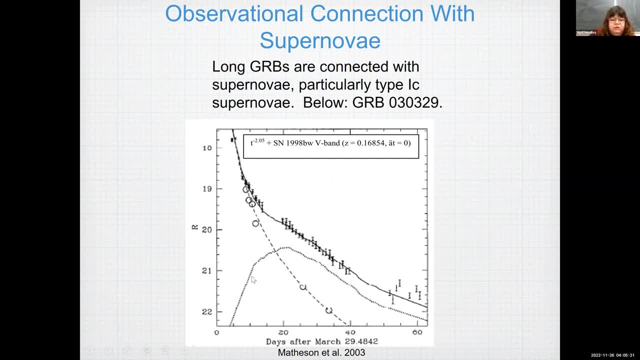 so it's basically, you think, intensity. so it's basically you think intensity versus, versus, versus. number of days, number of days, number of days. this curve, the dotted one, is this curve. the dotted one is this curve. the dotted one is a supernova. they're using a supernova. they're using. 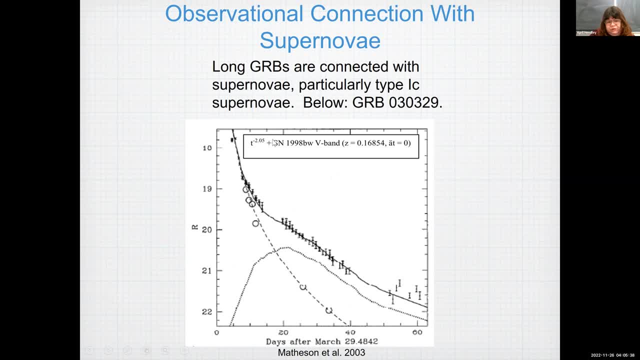 a supernova. they're using a similar. what they think of as a a similar, what they think of as a a similar. what they think of as a similar thing would be a similar. similar thing would be a similar. similar thing would be a similar supernova- supernova. 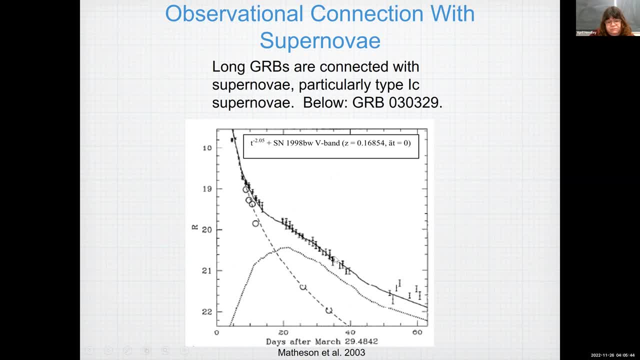 supernova and adding the two together and and adding the two together and and adding the two together, and basically it, basically it, basically it fit those light curve, for fit those light curve, for fit those light curve for the gallery burst, the gallery burst the gallery burst afterglow. 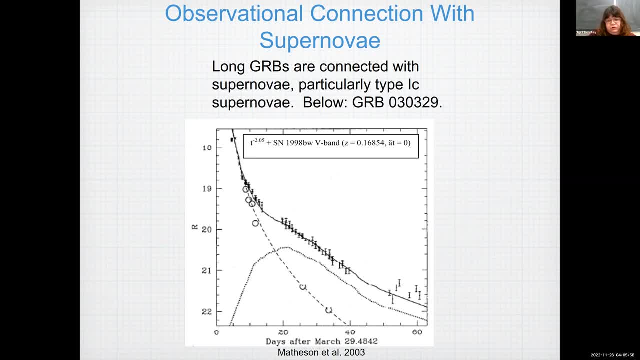 afterglow, afterglow. in other words, basically the afterglow, in other words, basically the afterglow, in other words, basically the afterglow from this gary burst. look like from this gary burst, look like from this gary burst. look like what they think of the typical afterglow. 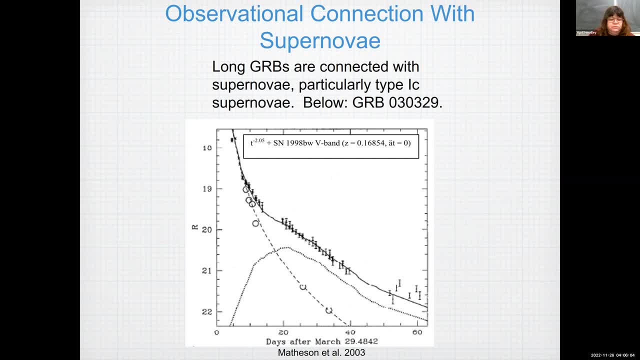 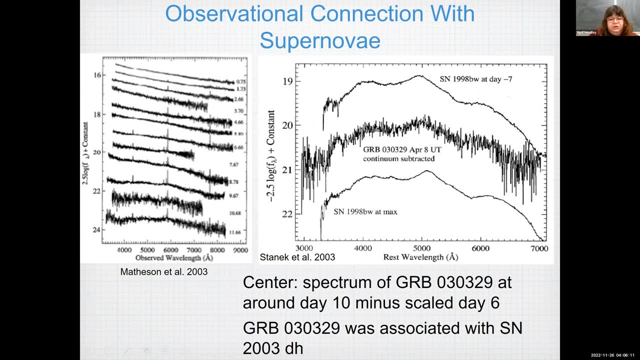 what they think of the typical afterglow, what they think of the typical afterglow plus a supernova. they also same one looked at spectrum. they also same one looked at spectrum. they also same one looked at spectrum. they basically took the. they basically took the. 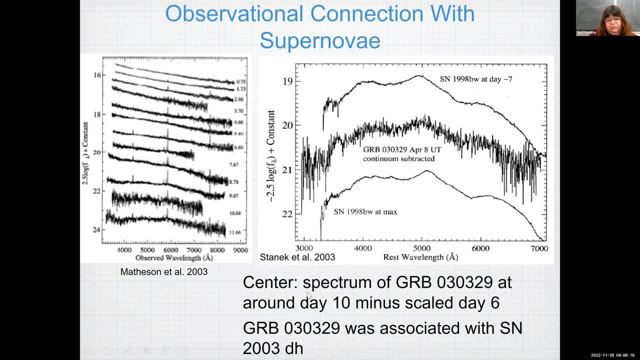 they basically took the spectrum about 10 days and subtracted the spectrum about 10 days and subtracted the spectrum about 10 days and subtracted the spectrum about spectrum, about spectrum about about six days, about six days, about six days, and got this and compared it to. 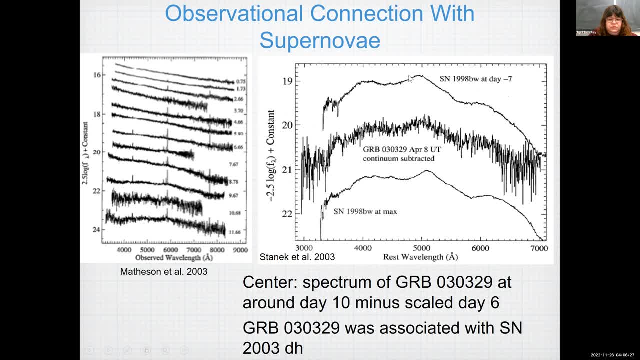 and got this and compared it to, and got this and compared it to two other supernovas, two other supernovas, two other supernovas, or another supernova at two different, or another supernova at two different or another supernova at two different times, and 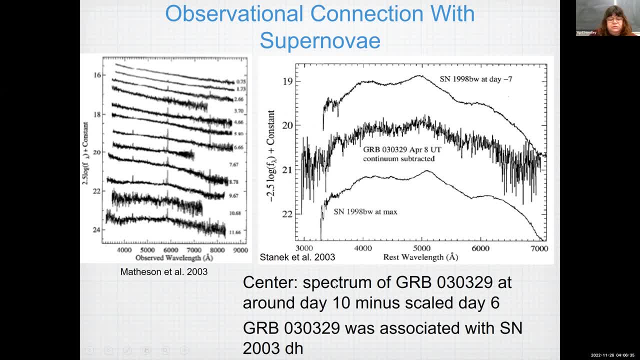 times and times, and it looks fairly similar in shape. it looks fairly similar in shape. it looks fairly similar in shape. so the reason why they took one day, so the reason why they took one day, so the reason why they took one day amongst the others, the. amongst the others, the. 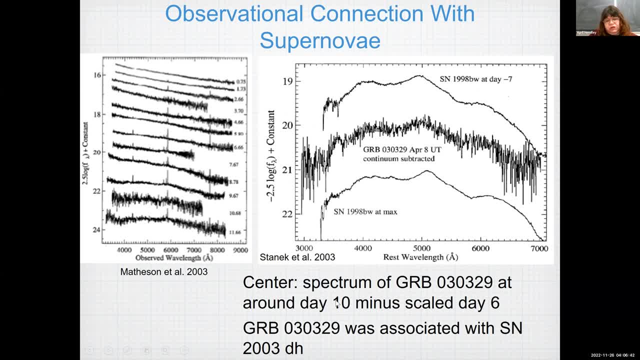 amongst the others, the one they subtracted was mostly just the one they subtracted was mostly just the one they subtracted was mostly just the continuum before it showed much evidence. continuum before it showed much evidence. continuum before it showed much evidence of the supernova, of the supernova. 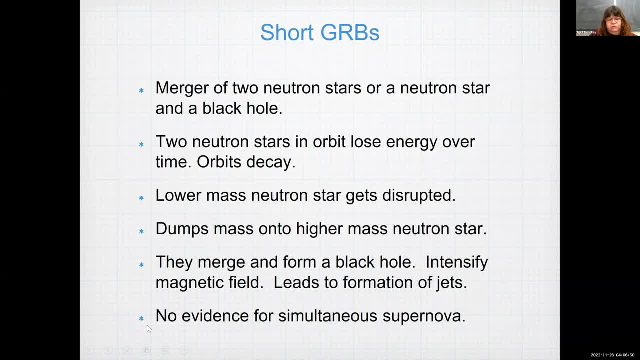 of the supernova. so they wanted to try to subtract out the. they wanted to try to subtract out the. they wanted to try to subtract out the gary burst afterglow part and just get. they wanted to try to subtract out the gary burst afterglow part and just get. 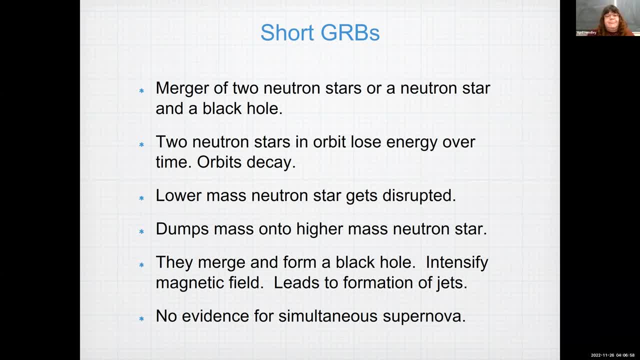 they wanted to try to subtract out the gary burst afterglow part and just get the mission from the supernova. okay so, short gamma reverse. okay so, short gamma, reverse. okay so, short gamma, reverse. um, i think, instead of being a death of a, i think, instead of being a death of a, 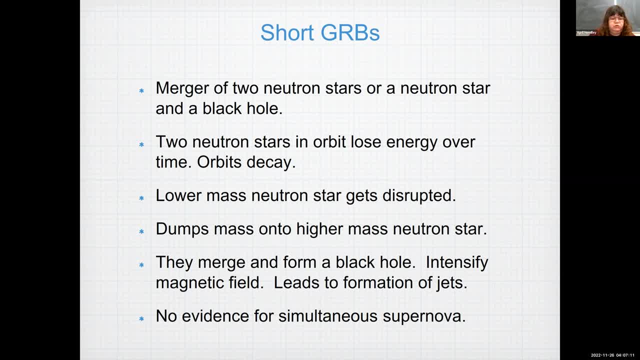 i think, instead of being a death of a massive star there, massive star there, massive star there, either two neutron stars merging, or either two neutron stars merging, or either two neutron stars merging, or neutron star in a black hole, neutron star in a black hole, neutron star in a black hole merging. so you have the two neutron. 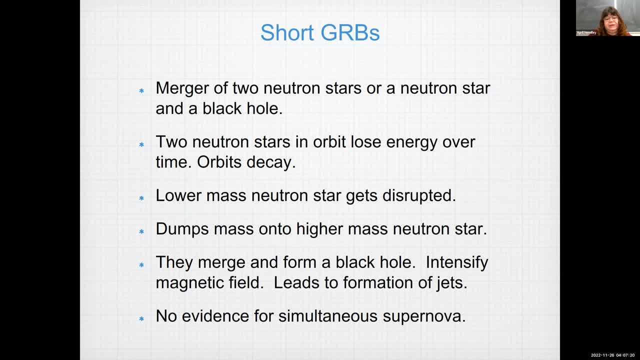 merging. so you have the two neutron merging. so you have the two neutron stars in orbit. they lose energy. stars in orbit. they lose energy, stars in orbit. they lose energy. the orbits decay eventually the lower the orbits decay eventually the lower the orbits decay. eventually the lower mass one gets disrupted. 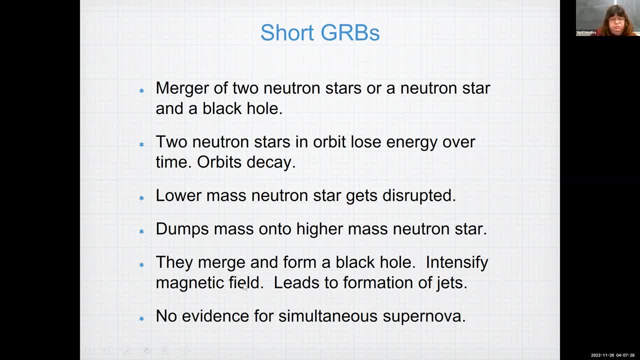 mass one gets disrupted. mass one gets disrupted. those masses on a higher, those masses on a higher, those masses on a higher mass. neutron star eventually emerge. mass neutron star eventually emerge. mass. neutron star eventually emerge. born black coal: get, get, get. magnetic field gets intensified, you get. magnetic field gets intensified, you get. 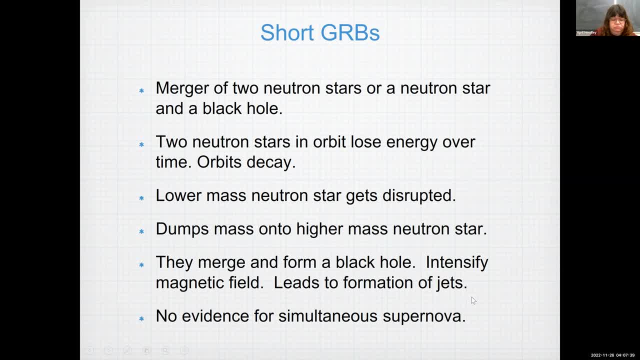 magnetic field gets intensified, you get a relativistic jet, like you did. and for a relativistic jet, like you did, and for a relativistic jet, like you did, and for the the the other type of gary burst, other type of gary burst, other type of gary burst. it's just in this case. 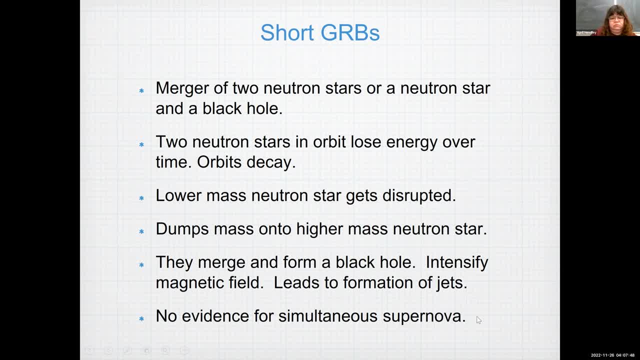 it's just in this case. it's just in this case because we don't see a supernova, because we don't see a supernova, because we don't see a supernova accompanying it, and the energy is like, and the energy is like, and the energy is like said. 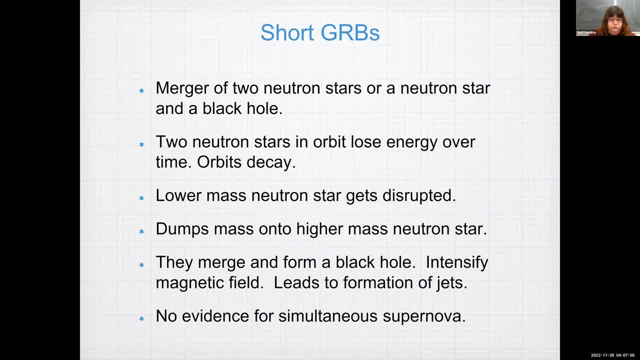 said said, tends to be hard. high energy photons tends to be hard. high energy photons tends to be hard. high energy photons though. overall, though overall. though overall, the overall energy tends to be less, but the overall energy tends to be less, but the overall energy tends to be less, but the photons 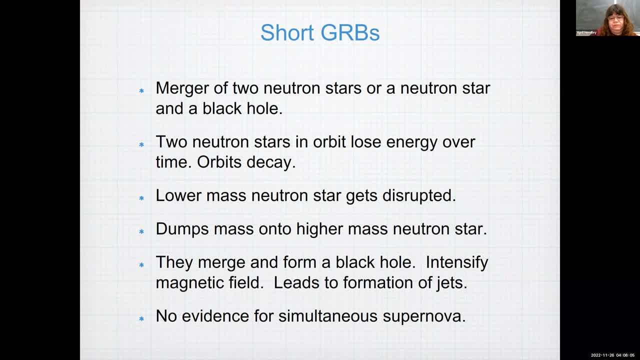 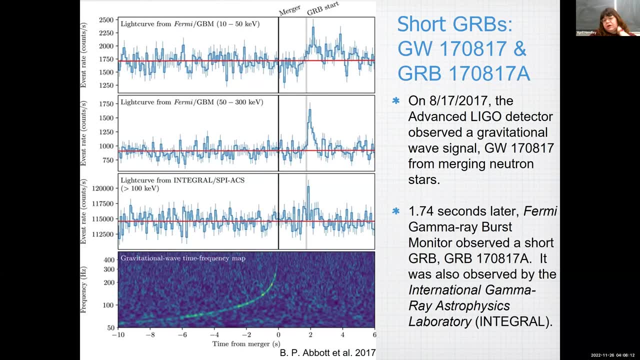 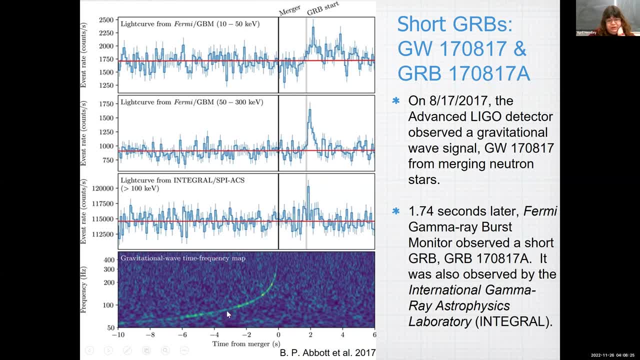 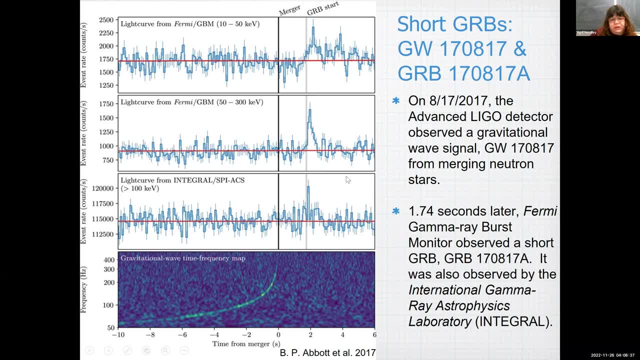 august 17, 2017. from a couple emerging neutron stars. from a couple emerging neutron stars. from a couple emerging neutron stars: 1.74 seconds later. 1.74 seconds later. 1.74 seconds later, they detected a gary burst. they detected a gary burst. 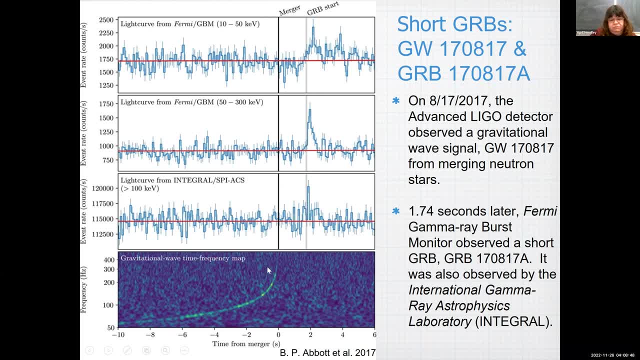 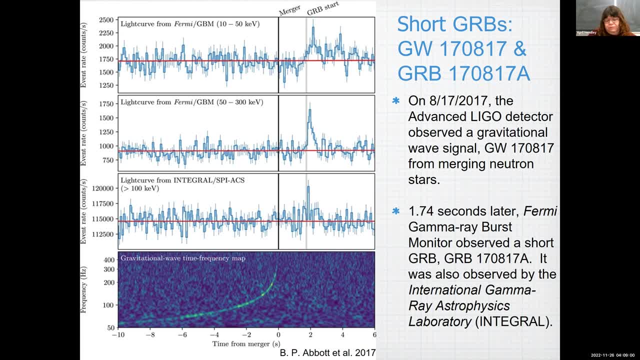 basically corresponds to what they think. basically corresponds to what they think that at least this, that, at least this, that, at least this, what the theoretical delay would be, what the theoretical delay would be, what the theoretical delay would be closely enough that basically it seemed. closely enough that basically it seemed. 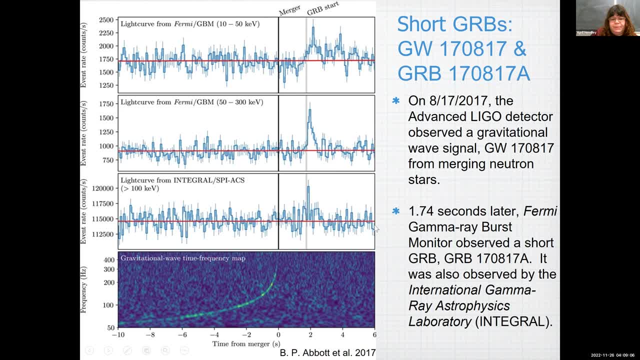 closely enough that basically, it seemed to fit to fit. to fit. models for that, models for that, models for that. so this is the so, this is the so, this is the the top three of the gary burst. so the top three of the gary burst, so. 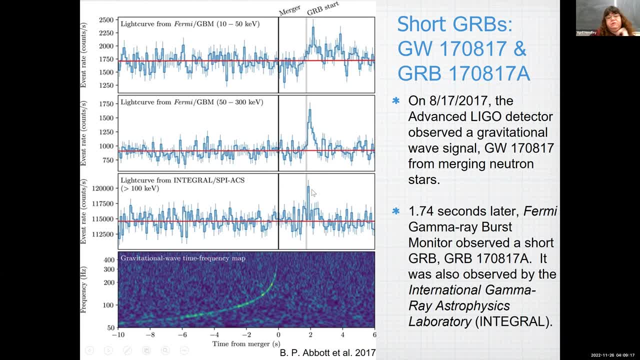 the top three of the gary burst. so, and just like the other ones, the peak is, and just like the other ones, the peak is, and just like the other ones, the peak is slightly different for different, slightly different for different, slightly different for different parts of the spectrum. 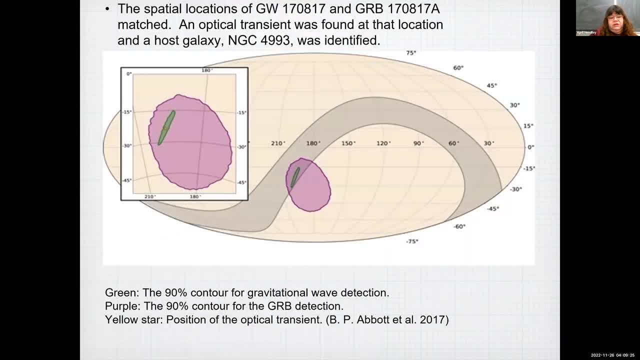 parts of the spectrum. parts of the spectrum not like that. the um not like that. the um not like that. the um gary, gary, gary, or the gravitational wave basically, or the gravitational wave basically, or the gravitational wave basically. narrowed it down to this little green. 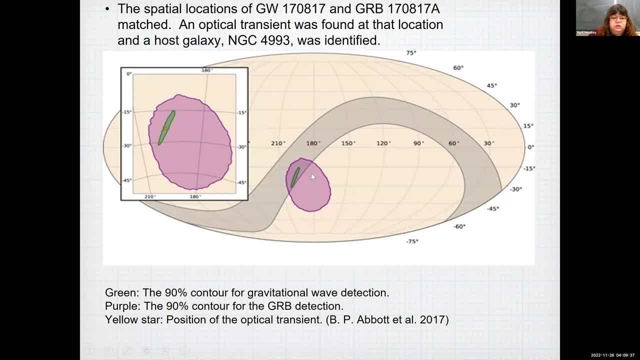 narrowed it down to this little green, narrowed it down to this little green area, area, area in its location, in its location, in its location, the gallery burst, the gallery burst, the gallery burst, the location almost narrowed it down to the location, almost narrowed it down to the location, almost narrowed it down to the purple area. 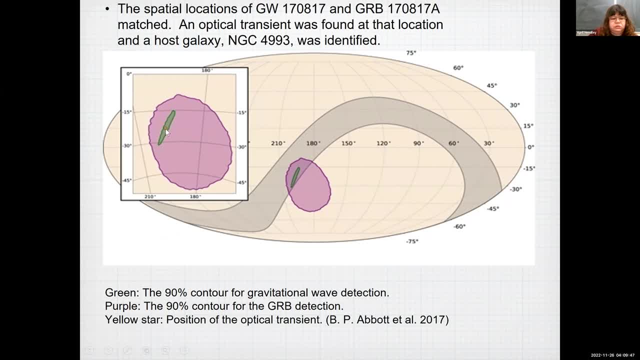 the purple area, the purple area, and then they detected optical transient, and then they detected optical transient, and then they detected optical transient, basically, basically, basically like the visible light from the like, the visible light from the like the visible light from the supernova, And I hope the optical transient is a star here. 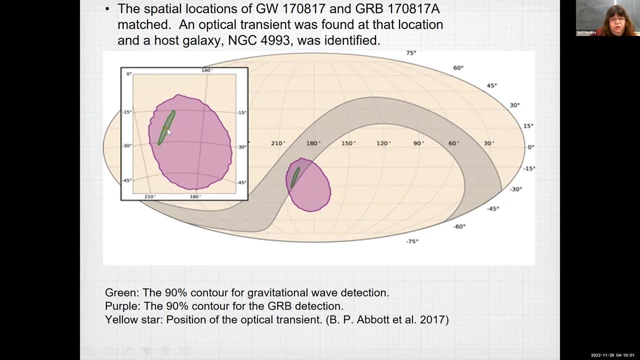 And they also found a host galaxy too, that all basically lined up or were consistent with the location. So this is just one star. that is what you're saying. like the optical spectrum that was observed, that was only from one star. 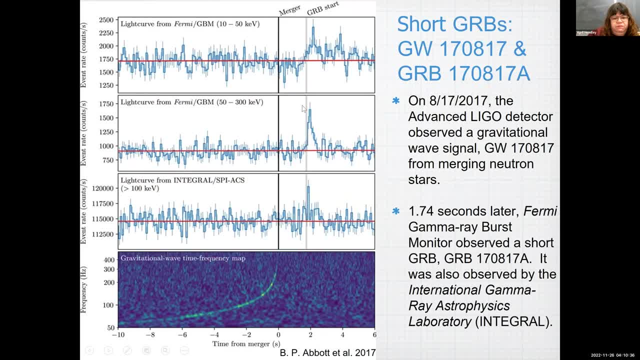 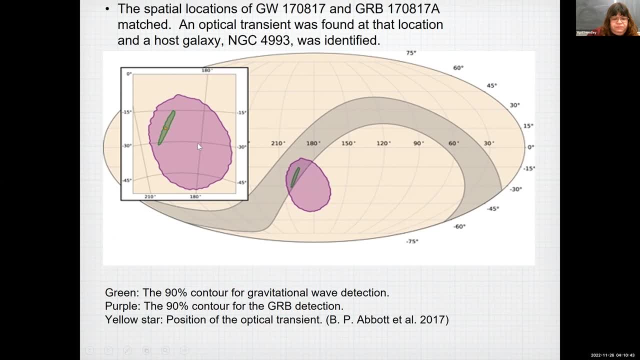 Yeah, like this was here All from one short gallery burst And this is, like I said, the purple is that gallery burst and the yellow dot is basically the optical light from it, basically the supernova part, Interesting Okay. 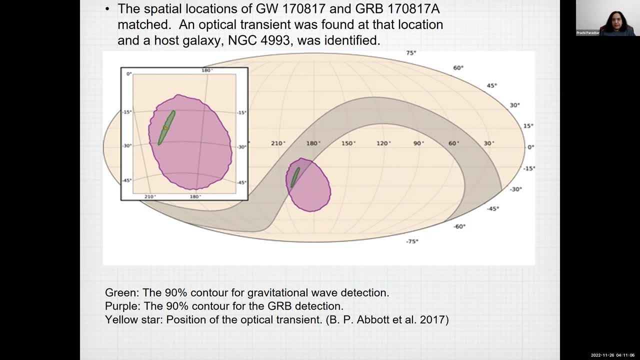 So you're saying that this particular thing like the galaxy- Yeah, Yeah, Yeah, Yeah, The galaxy was not known before. No, the galaxy, I think, with having this catalog number, the galaxy was known before. but the optical transient and all this lined up more or less with this galaxy too. 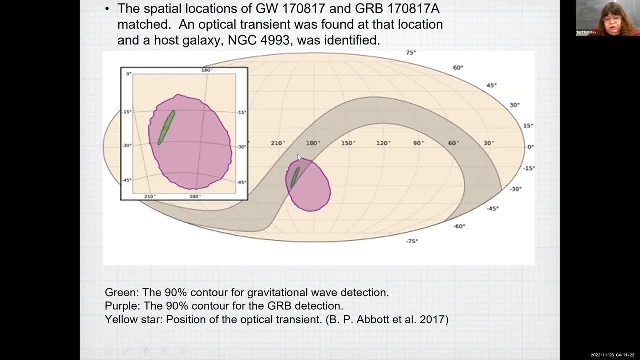 But there could be a number of galaxies in the purple area for sure, And even the green area even covers enough that it could be several green areas. It's just the optical transients where this yellow star is. It's just that Everything at least fit in the same overlap and where they were. 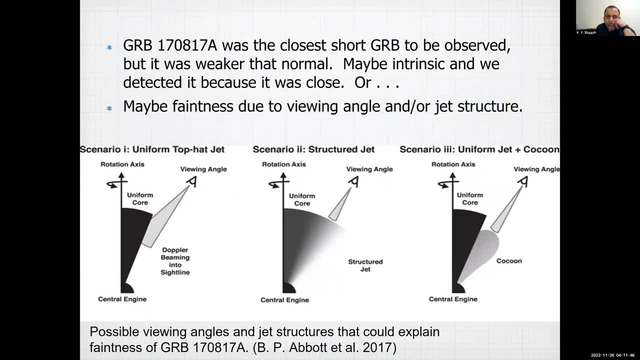 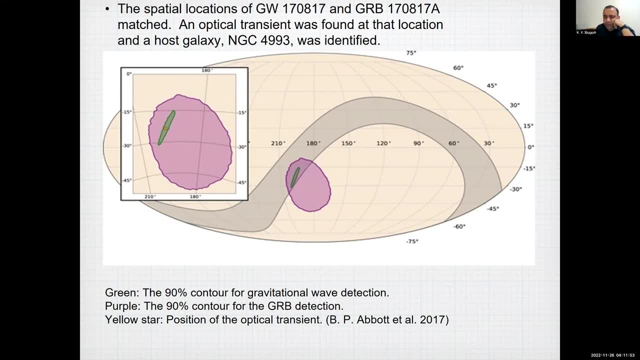 So, So, Krishen, when there is so much error in the gamma ray detection, is that because of the device we are using, or is it just that gamma ray burst seems to be so, so much across in the sky? All right, 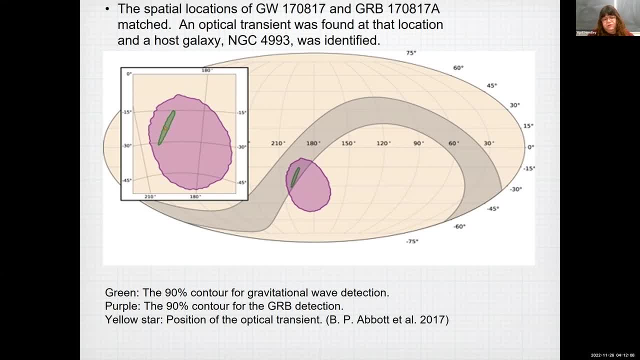 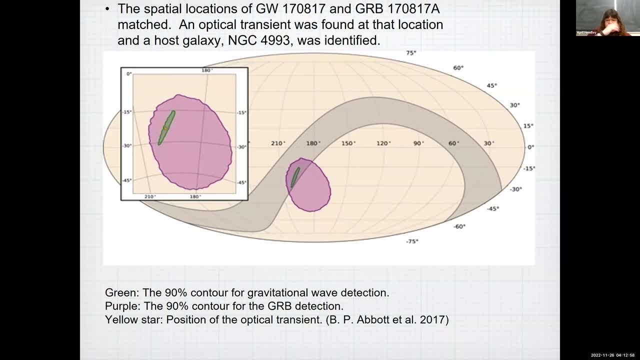 cells, cylindrical mirrors. it's at very slight angles because if the um- basically if they're at angle like that and the gamma ray comes in or the x-ray comes in at a shown angle, it can bounce off some and come and you have nested ones. you can bring x-rays to focus that. way, because you'll have like another one, that'll basically be kind of cylindrical and you and the x-rays will bounce off at that angle, but they won't. if you send it more and more normal to the mirror, the x-rays would go through, but the gamma rays, that don't even work. 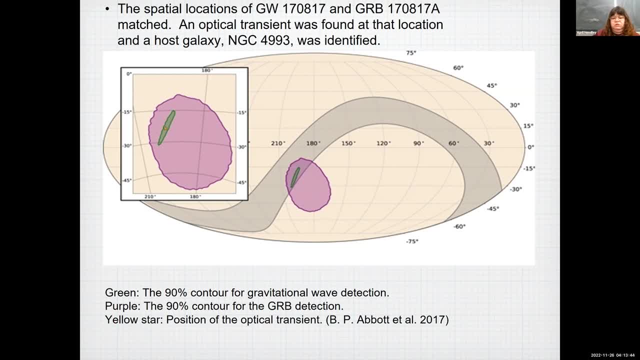 so, in other words, it's part of a lot of the problem they had finding, and still do find, location just based on the gamma rays is the fact you can't really get true images. so, okay, thanks. um, one thing about this gary burst that was associated with this gravitational wave: 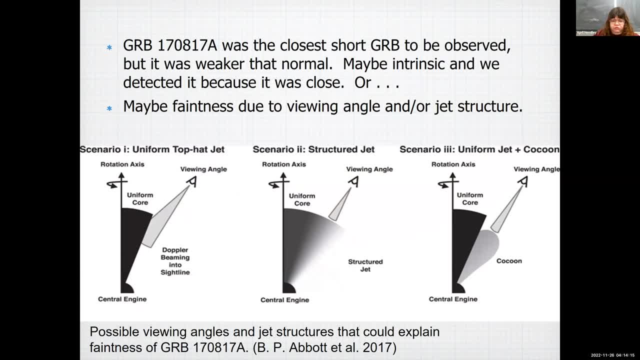 was. it was the closest burst that had been observed, but it was also weaker than normal, which leads to some questions about what was going on. now. question is: could it be intrinsic and we just happened to take that was because it was close? or could the jet have some structure and us? and it depend on our viewing angle. 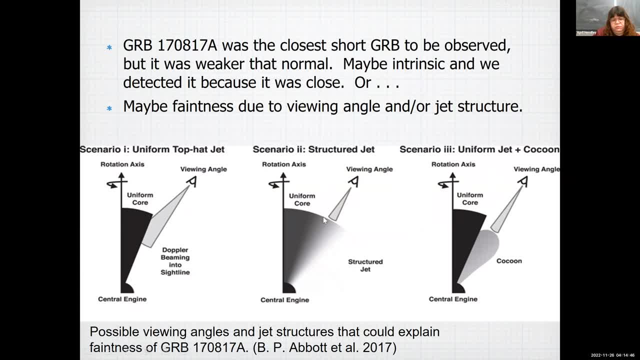 like. are we viewing the side of the jet instead of straight on one? is the jet to where it's more intense, basically with, let's say, more intense or denser at the center and not as much at the edges- and we're seeing it edge. or could there be some material forming some type of cocoon around? 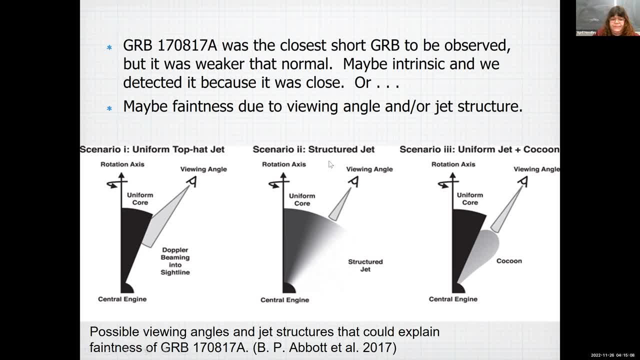 the jet and we're seeing that it's more instead. so, um, i'm don't. i'm trying to think, if i don't remember looked up stuff recently- whether there had been- i don't remember seeing anything about another one- detected gravitational waves yet, but i don't think they've detected. if there has been one that hasn't. 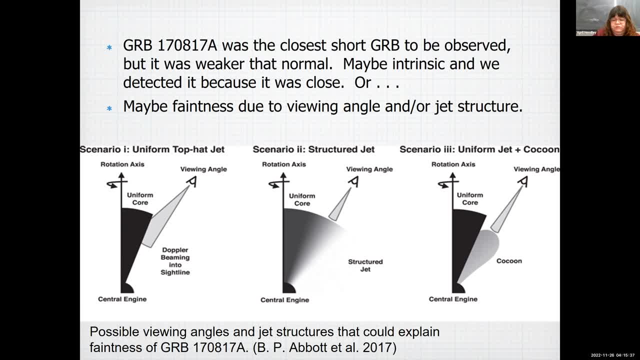 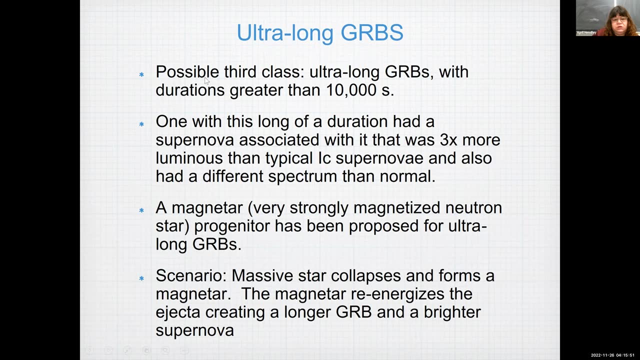 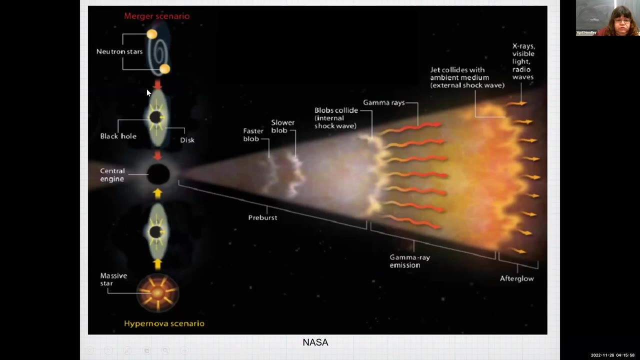 been too many at all, so i don't remember seeing one when i was looking at more recent research recently. okay, So go forward for a second right here. so this is the for the merging neutron stars: get the black hole, still get an accretion, just just no supernova and you still get the jet. so this would be. 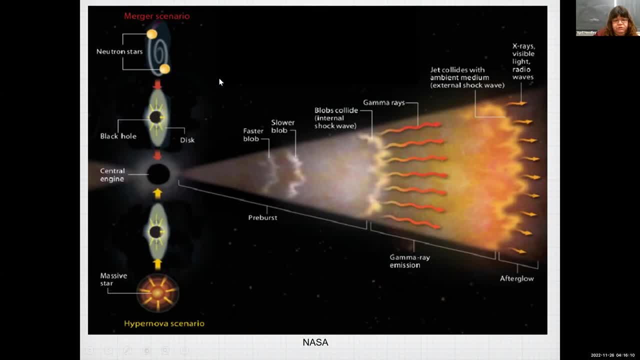 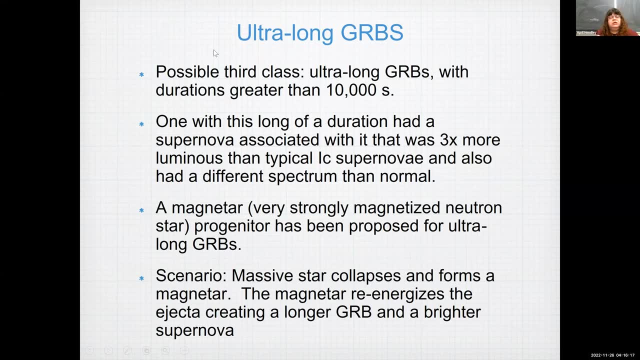 basically the short gamma ray path on this diagram. okay, so there was a possible long class of Gary burst with durations like larger than 10,000 seconds anyway, um, one that had one that had duration that long, had a supernova that was three times more luminous than typical supernova, and also 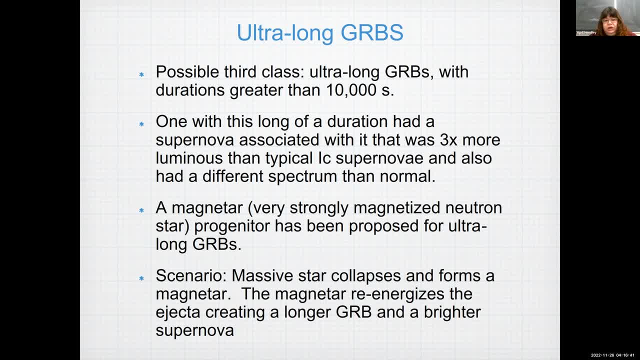 spectrum was different. um man, the one of the proposed possible progenitors was called magnetar, which very strongly magnetized neutron star, and the possible theory on that would be: you have a massive star collapse, you get the magtar and the supernova. uh, magnetar then managerizes that ejecta. you get longer and brighter supernova. 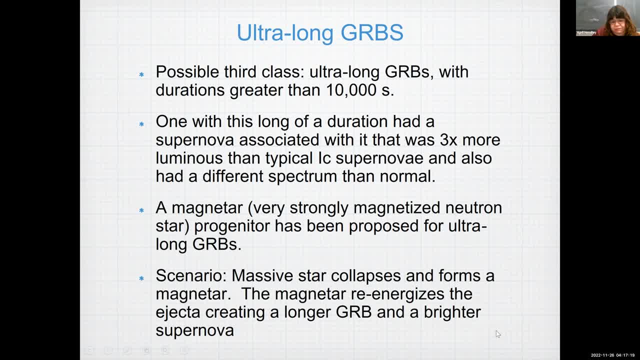 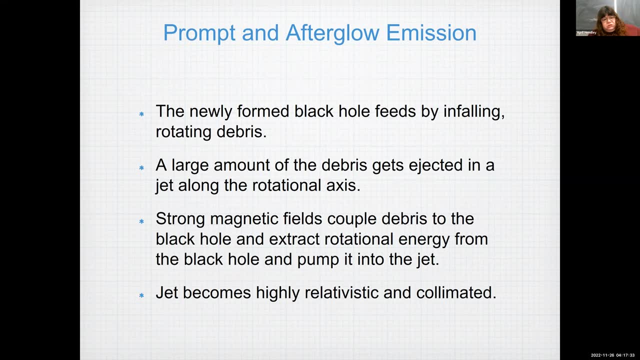 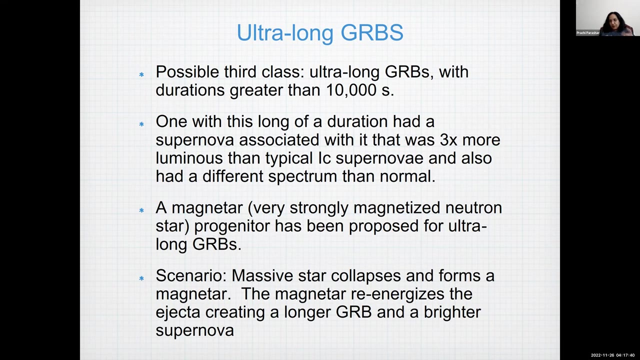 this period more uncertain than the previous one, than the short and long ones on the previous slides, But they have been observed, right? Like, basically, you're saying that the intensity for more than 10,000 seconds from single source has been observed, right, Yeah, some have been. 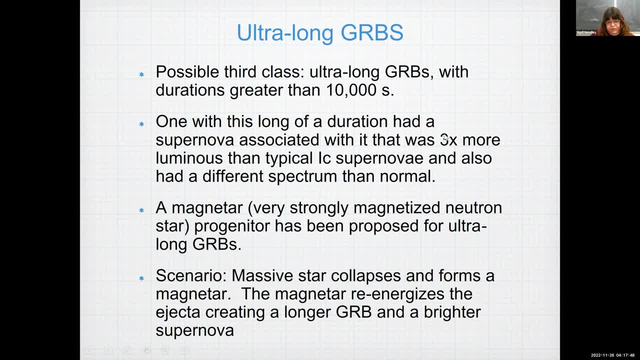 I don't think. to me it's been this bright, but it's still fairly. So what is actually the confusion here? Like I mean, you said that like there are it's not like. so basically, it is not known that it is from the magnetized one. 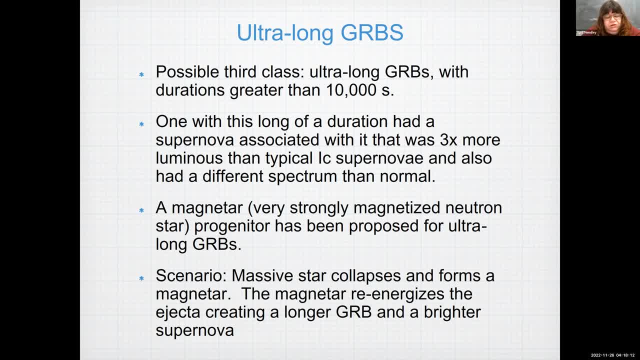 or like: what is the? This combination of that and the fact that I think they're really More enough recent that they still are coming up with explanations, So source is not certain. Yeah, It took a while after they started localizing the other Gary verse before they ended up. 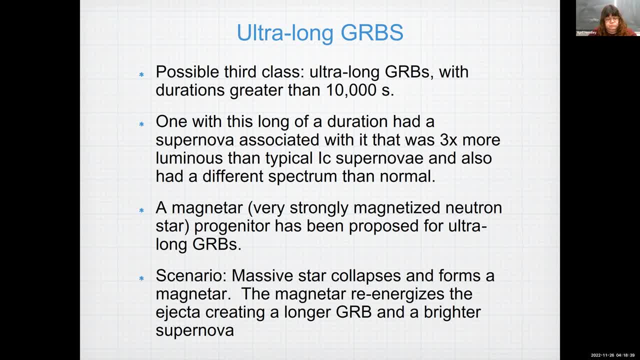 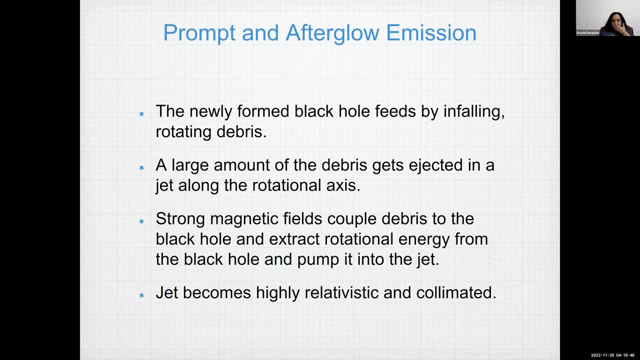 getting a good idea of what source is on them. so You had a question, Shahjesh. No, I'm good. Thanks, Okay, That's for the mission itself. You get this linearly formed black hole and, following rotating debris, You get debris that gets ejected in a jet along the rotation axis. You get magnetic fields. 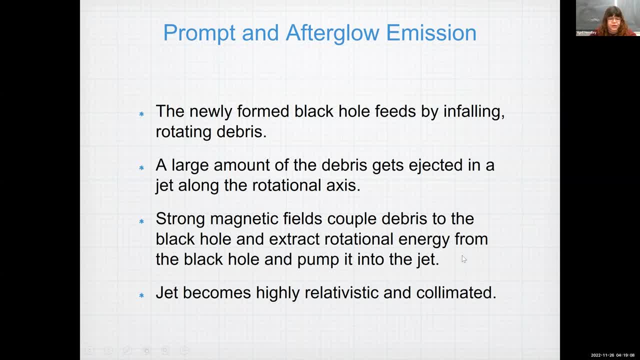 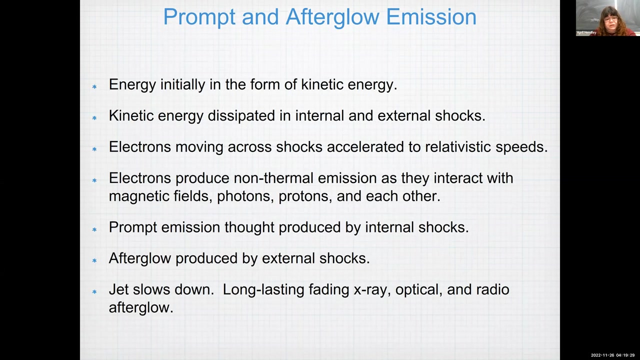 a couple of debris to the black hole, get rotational energy from the black hole, pumping a jet, and the jet becomes highly relativistic and basically collimated. And then, as I said it, Hugh will turn on the simulator when I die. you get the. 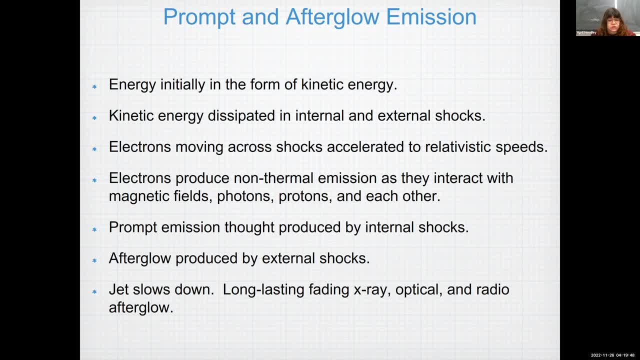 stuff surrounding the star And then electrons across the shock will get serrated at relativistic speeds, get non-thermal emission. they interact with magnetic fields, each other protons, protons, basically synchrotron. what was it? 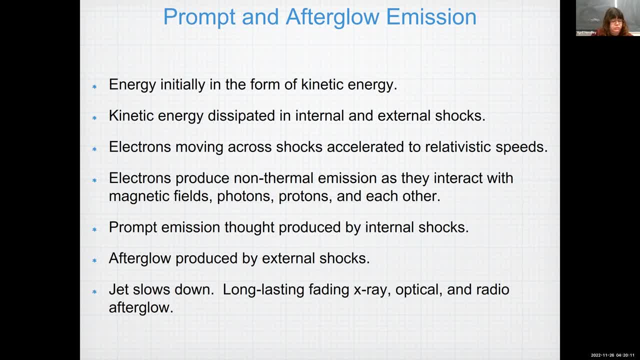 I'm trying to remember Andrus-Compton and that took us picture on my screen earlier, so I'd remember, because I get slightly confused. Andrus-Compton and synchrotron-Seph-Compton- I get confused on the two Comptons sometimes. 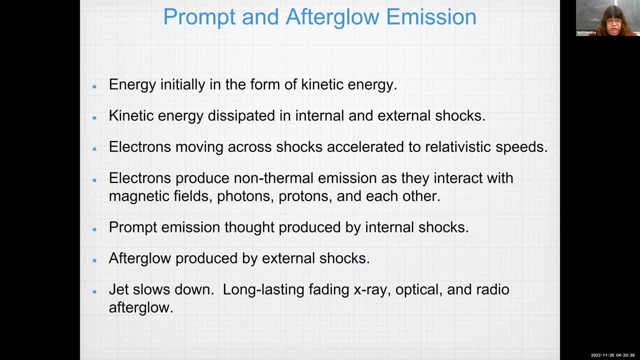 But anyway, I saw the prompt emissions from the N-tron shocks and the afterglows from the X-tron shock And eventually jet slows down, loses energy and get X-rays, optical, radio and poly poly in between X-rays and optical. 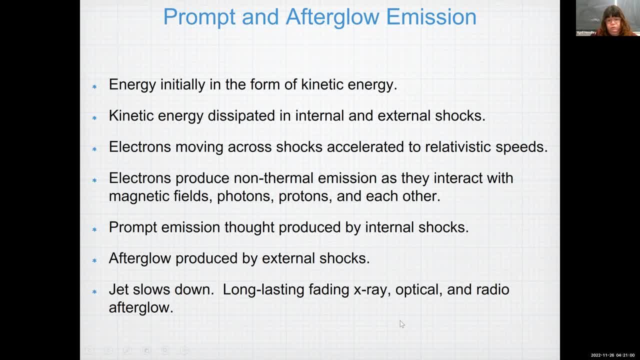 poly ultraviolet and also infrared, in between the optical and radio. And that is actually it, Any questions? Do you have any questions? I mean, I was asking in the meantime, so I think if we just discuss something, then probably something comes out more naturally. 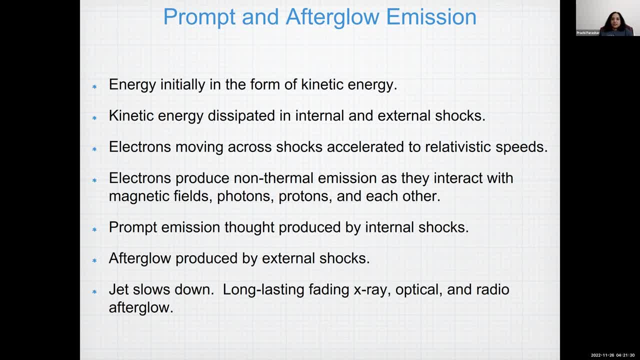 I think the answer to our question is no, and you know, we just had to think about this. So would it be correct to say that, like supernova, supernova is used to measure distances, Like one-eighth supernova is used to measure distances? 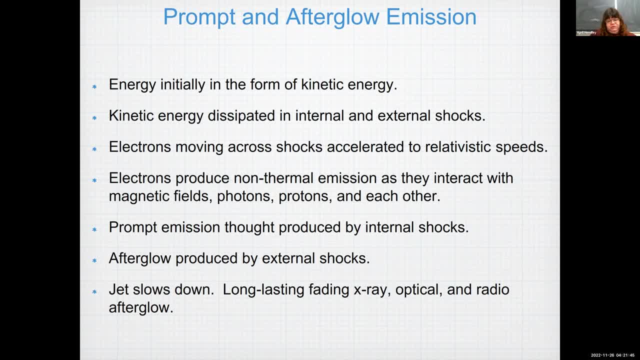 right, Supernova, yes, supernova, supernova, supernova, supernova, Right, supernova, supernova is used to measure distances. used to measure distances, though. oh, and these are from 1c, is it? yeah, they're not used to measure. 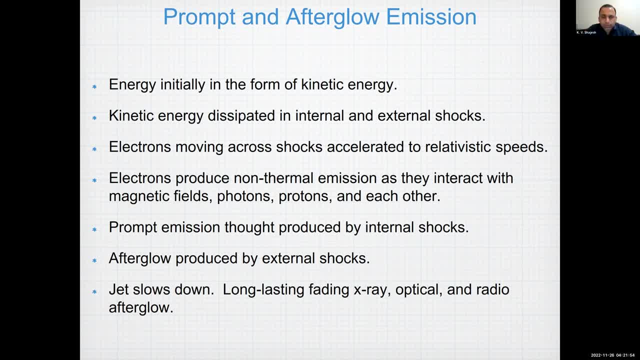 distances. so much, i see you get the distances for these. they had to be able to get them localized enough to find the host galaxy. then they could get distances from that. okay, so, okay. so my question is not even there. yeah, the 1c's can have different brightnesses. 1a's hell have about the same. 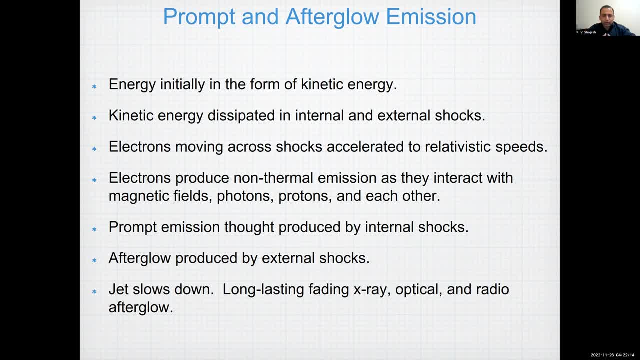 brightness. yeah, that answer, because i was going to ask that how come they are able to measure distances when it's not a clarity on? so whenever they observe, like these 1c emissions, like it's not like they're coming in, i mean, is it quite clear that these gamma ray bursts whenever they're? 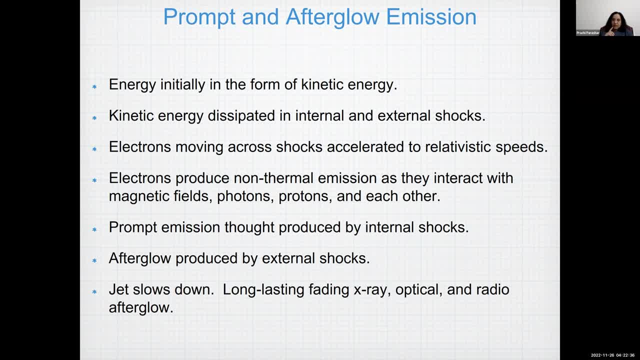 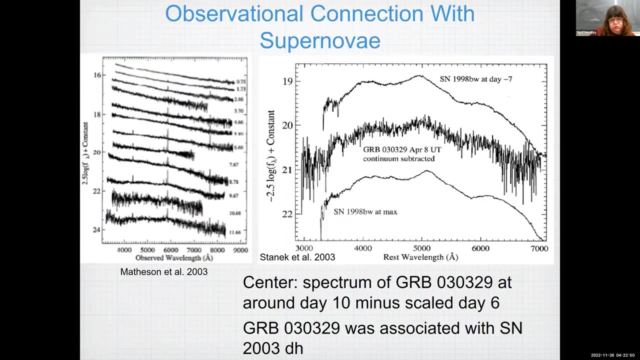 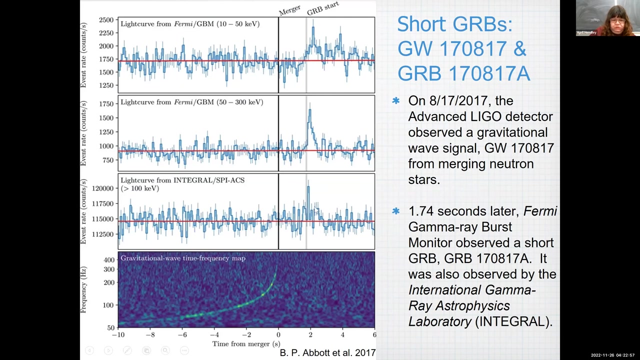 observed. they're all coming only from one source and it is not that like it is just one star doing it, but multiple stars in the in the galaxy are sending out the burst. yeah, um, they're fairly sure it's only one star. i'll go back. actually, this slide will work how it has to do with how spiky these things can be. 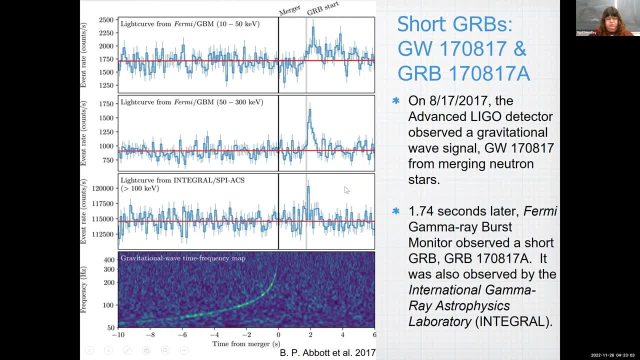 like how it fluctuates rapidly with the brightness. that gives an eye maximum limit to their size, because the light of the galaxy is not the same as the light of the galaxy. so it's not the same as the light of the galaxy. so it's not the same as the light of the galaxy. so if something can in some astronomical 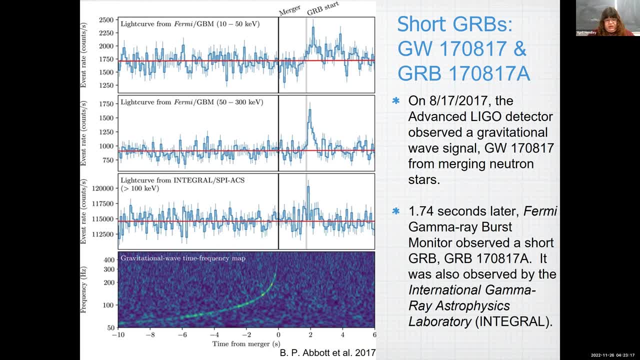 object and only fluctuate as fast as light can travel across it. so if it takes light one second to travel across the source, that's the fastest it can fluctuate in terms of its luminosity. so basically, because of how fast they can change the light output, that says they have to be fairly. 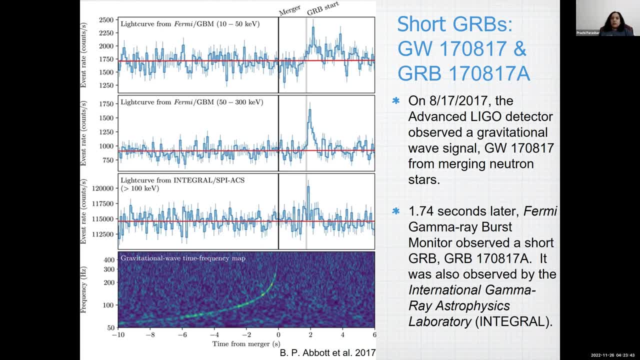 small. so okay, so can you show me another example where you cannot show? say that it is, uh, it's from one source. it could be from multiple sources. um, you mean, like, like a graph of the same kind, like right now. you said that the peak, like narrow peak, decides that whether it is a one source or not a one source. but 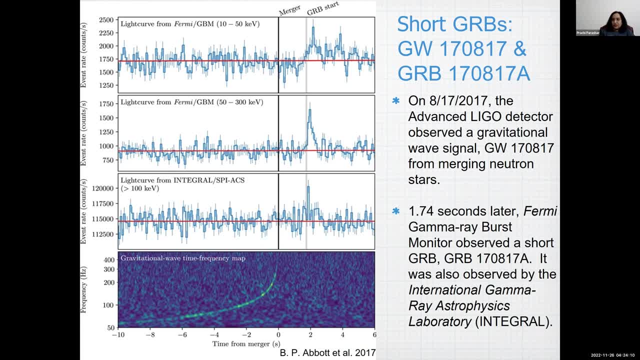 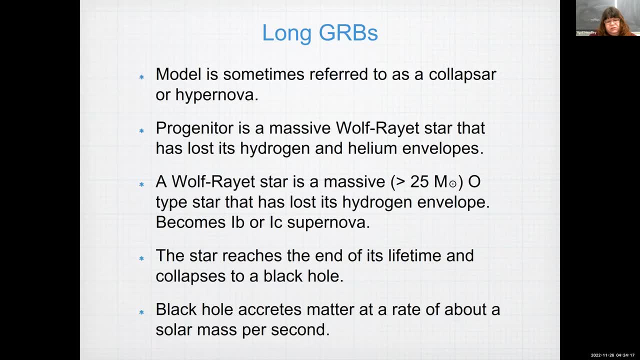 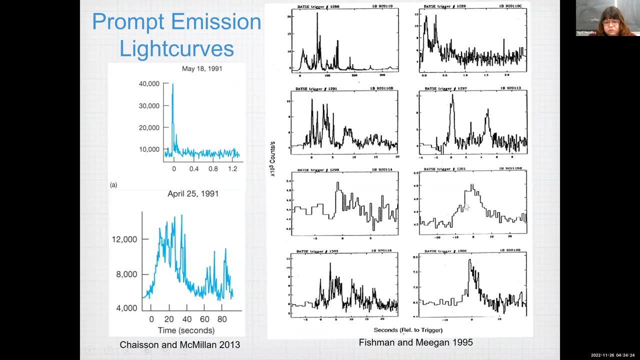 do you have another graph which shows a broader peak, or something where you can surely say that it is not from one source? not that i can say surely, but the broadest one i have is just this one. you still have the spikes- or this one's just 10 seconds, so from here that's 10 seconds to zero. so so does it say something like i: 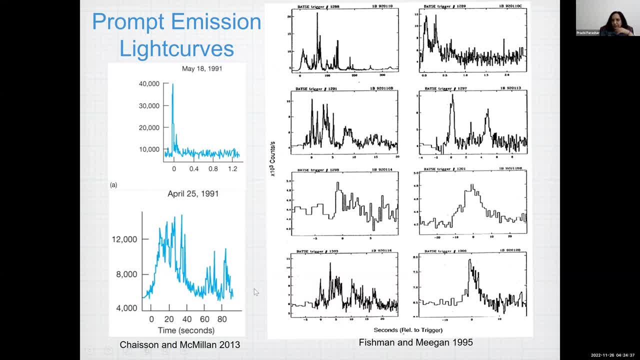 mean does, can you? from there you cannot conclude that it is from one source. it could be multiple sources. yeah well, that was different from one source to another source, so i don't know if it's still have to be something that's, but most probably 10 second, 10 light seconds across. so 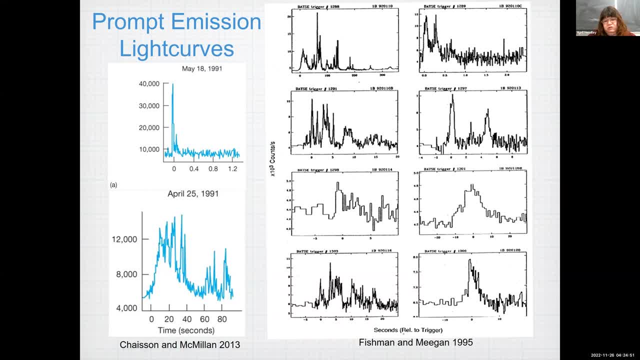 so that's still, i don't know- takes eight minutes for light to reach us from the sun. so what's the? what's the size of sun in light seconds, or i don't know, on that one, how long it long it takes to reach the sun. I don't know how long I'd take, in terms of light seconds, for the sun across the sun. 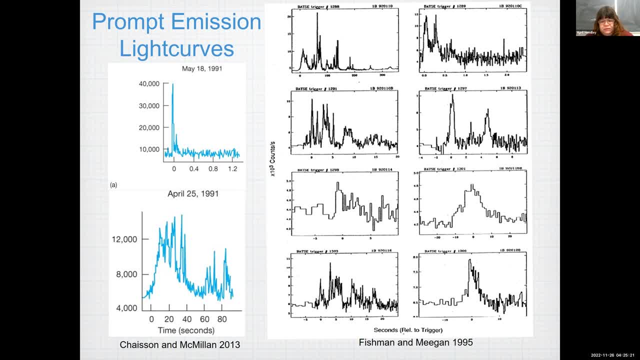 Like, yeah, go ahead, Shajesh. I'm saying it basically: if this is roughly 10 light seconds, it's still be probably smaller than Mercury's orbit, for sure, which, Which is still can be just one star. Yeah, because there's stars that's basically about as big as our orbit. Like, the way I am thinking is that, like, see, the most galaxies are formed. like most stars in the galaxies are formed during the same time, right, So they're aging the same way, most likely. 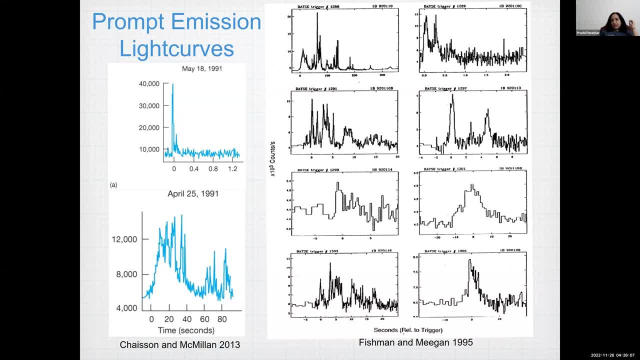 There will be, like numerous stars in a galaxy That might be going through the process of this supernova formation or like I mean a gamma ray burst or something. And if you are like, if you are observing it, like suppose the telescopes are pointed in the direction there of collecting data. 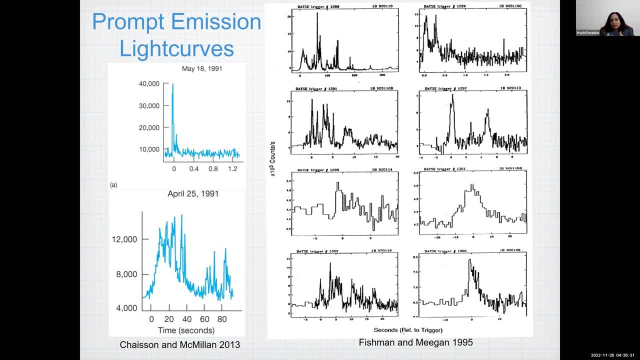 Like how do you distinguish whether this is coming from multiple stars in a galaxy or it's just Yeah? I mean, you know I'm Partly. they're probably using nearby galaxies, this supernova rate, to get an idea of how many is likely at any one time. 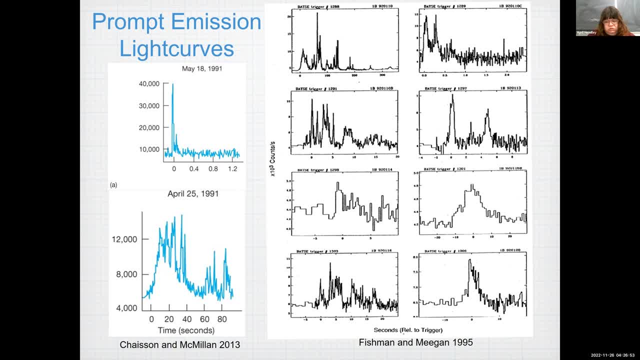 I mean, let's say, just like in our galaxy. it was like: well, the last one that occurred in our galaxy was like Kepler, I think, Kepler's supernova so nova, so that we know of so, and like, if they look at andromeda they can see the rate of it, and other ones. so it'd be well. i wouldn't say it's impossible to have a couple of stars at the same time. it's just based on what we can see with the galaxies nearby and supernova in general and the galaxies that we can see in galaxies. it's just not that likely. 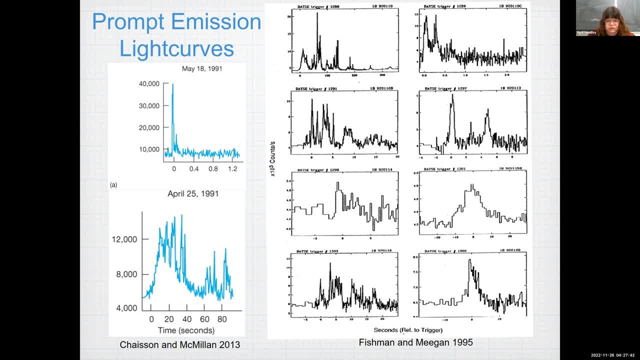 so that's great, that's supernova. just so, from what i gather, would it be correct to say that the area under these curves give a measure of the mass of the of the star that was dying? i say i'm trying to think if, because the area on the curve would probably be overall. 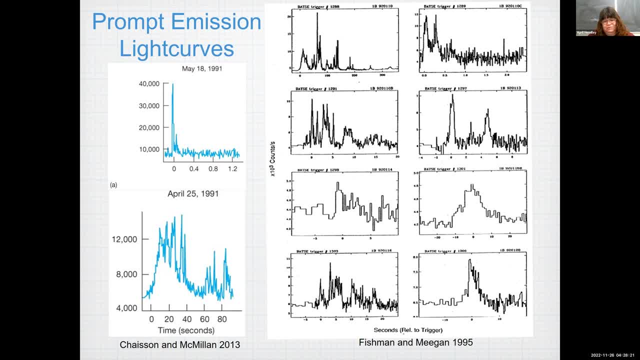 luminosity of the gamma ray burst and that may not correspond to the actual mass. if there's enough, uh, there will be dust released. also, right, a lot of matter particles will be out if they lost enough mass before they went supernova and had the gallery burst and that wouldn't be as 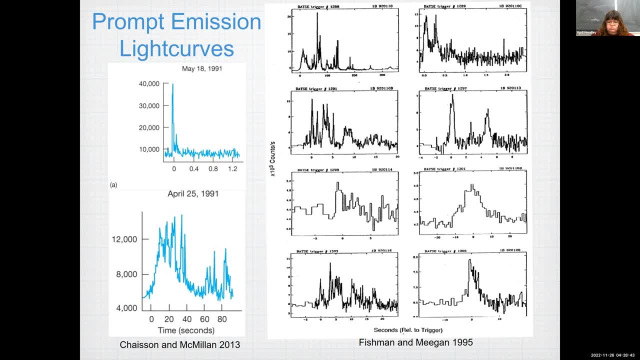 then some of that dust could obscure it, it wouldn't be as bright. i see, okay, yeah, very interesting, yeah, interesting, but i i get confused also a lot uh with, uh, the galaxy formations, basically. so when the, the nebula, the like the, uh, eventually, when the stars die, they create the planetary. 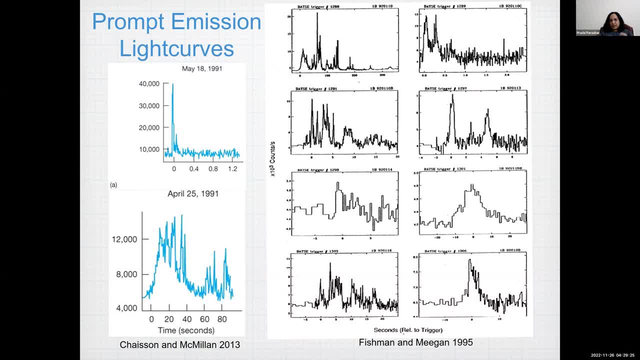 nebulas right or like nebula basically, where the star formations will begin again. the planetary nebula is like lower mac's star formation and that's what i'm trying to tell you about the star formation, and you can go to the nebula foundation and you can just keep forgetting. that's a lot of heads, because that's not the best�. 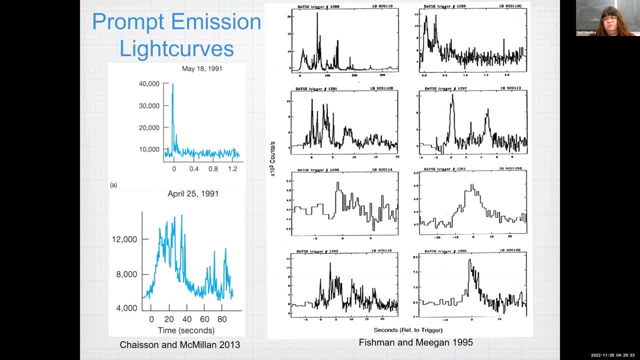 stars and that material will eventually get mixed in an interstellar medium, but, um, because i expand slowly enough that it'll be a while before it gets incorporated into a new star. so, yeah, like, i mean, just like, i mean, i'm just trying to like, understand the fact of for galaxies. 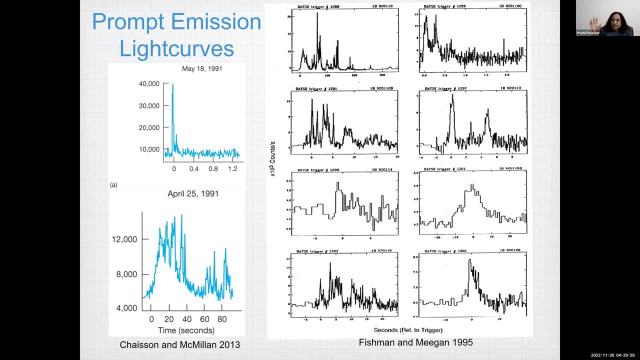 we say that almost all galaxies have a black hole at the center of that, which means that they are probably coming from the earlier supernova, somewhere where the black hole actually formed a supermassive star when it collapsed and created the supernova and then it got the. 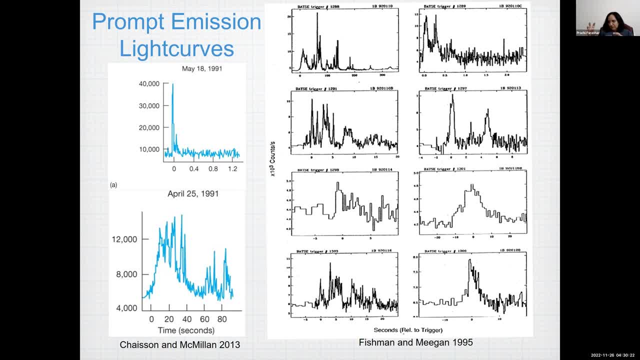 uh, formed the black hole. i i don't know like i'm slight. i don't know like i'm slight. i don't know, i don't know like i'm slight. i don't know like i'm slight. i don't know like i'm slight, i don't know like i'm slight拜拜. 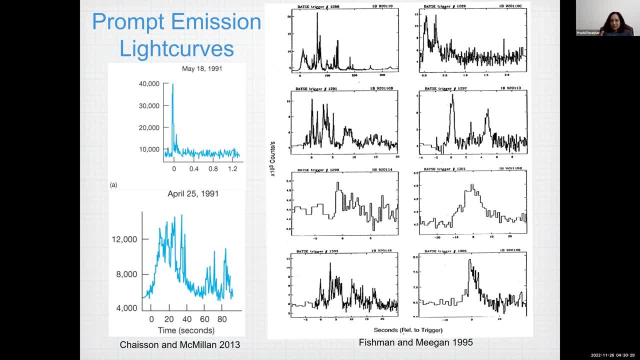 get always confused, like because each galaxy has like millions of stars, right? yeah, keep in mind. they also don't really know how the galaxies get the black holes at the center um, and generally a lot of times they're regarded as separate entities from the? um stellar mass black holes. 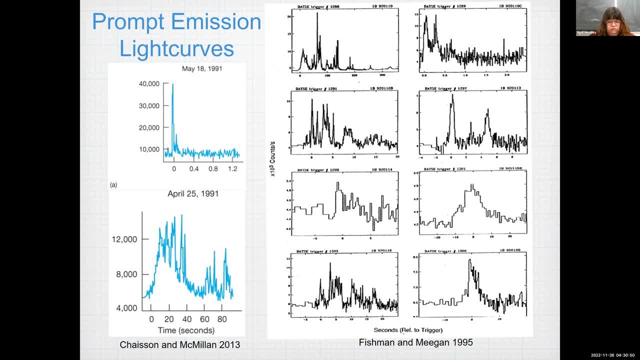 so there's even black holes somewhere, that's in the like tens of thousands of solar masses, and they really in immediate mass black holes and they really don't know, yeah, why, how they formed either. so there's a lot of things are still unanswered. um, yeah, lots of uncertainties. 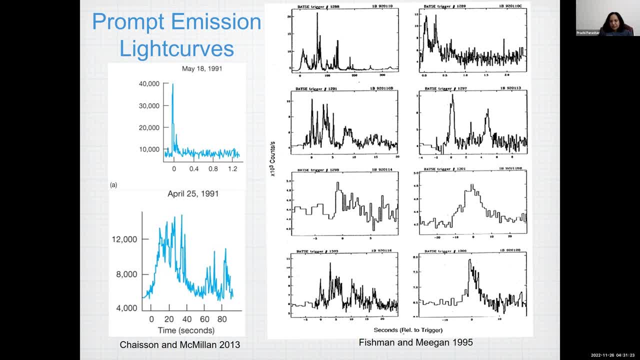 and and the point is like, when we talk in terms of like, uh, death of stars, i mean galaxy again. the galaxy has millions of stars and they are formed around the same time, roughly the same time, probably be dying around the same time also, like this could be on a span of millions of years. but it is around the same time they are dying and, uh, the most of them will go supernova, right. uh, most stars are going in like the sun, just as a planetary nebula, just kind of, as they say, kind of with a whimper rather than a pain. 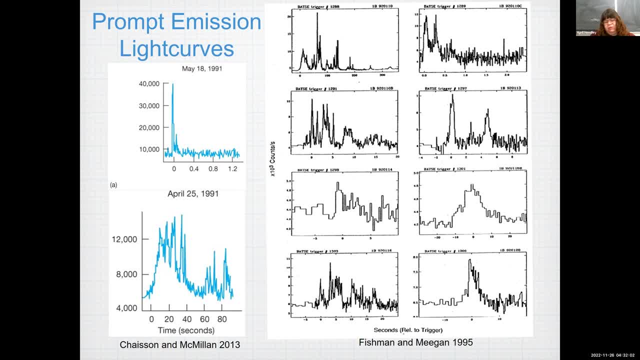 yeah, yeah, ones that blow up in supernova are the rarest stars. maybe what i think it's like one in ten thousand stars fall into that massive star category. yeah, but it's still one galaxy will have multiples of them. yeah, yeah, yeah, I don't know, but, like i said, they can look at galaxies and the. since we see supernova and other galaxies, they get an idea of how often a supernova occurs. 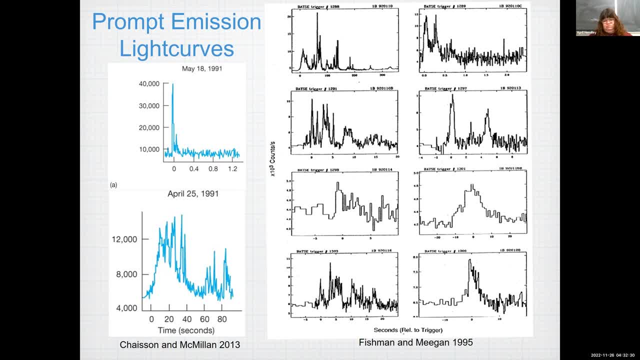 so when it's, and keep in mind you could, but we want to think that at the same plus, at the same time. the other thing to keep in mind is in terms of stars: half of them are stars, half of them are stars. yeah, yeah, no, i agree, i mean. that's why i'm saying, like the, the birth and death, all are happening in millions of years time period. 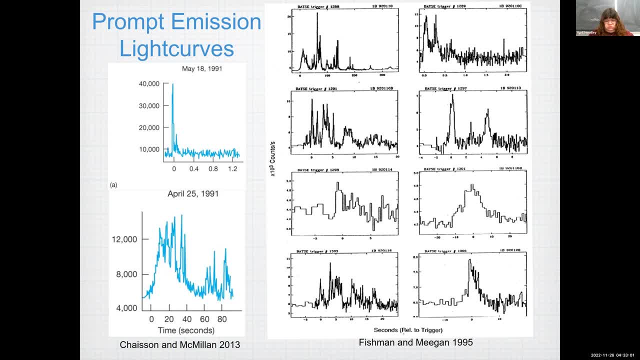 and again i was thinking like there should be multiple supernova in a galaxy, yeah, but i was gonna say you might have once every few thousand years in a galaxy, but for us that seems long, for galaxy that's short, or for a star that's short. so